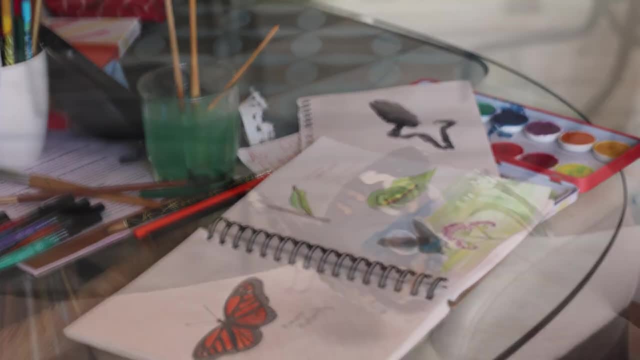 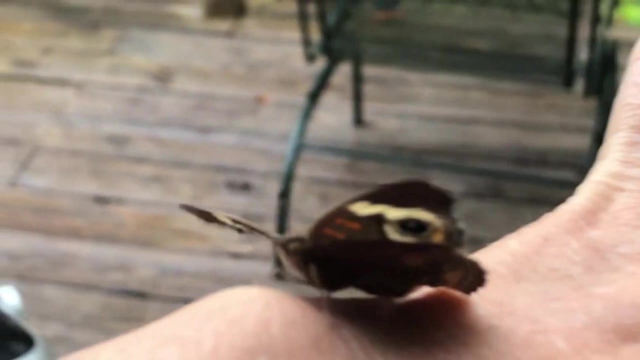 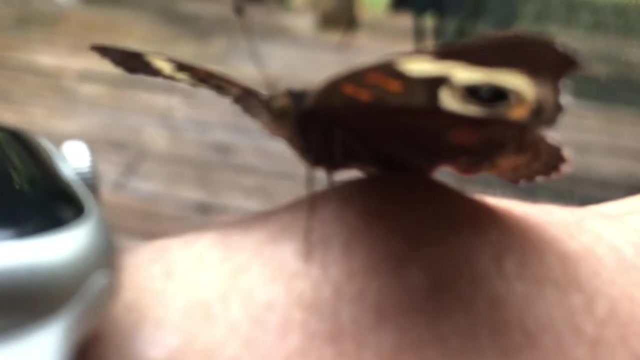 The goals for me were twofold. There was some time ago that I came to realize that there were two different ways of knowing in regards to the natural world. You could study and have book learning and know a bunch of different facts in the natural world, and then you could also have a 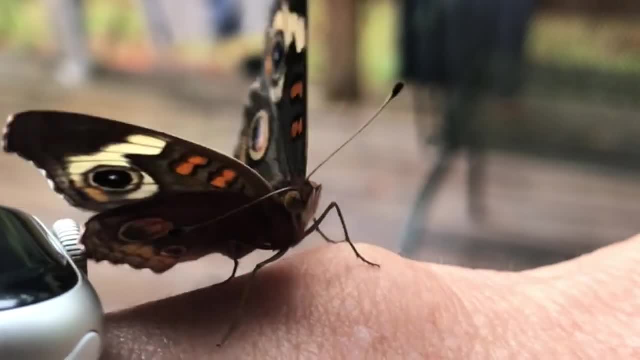 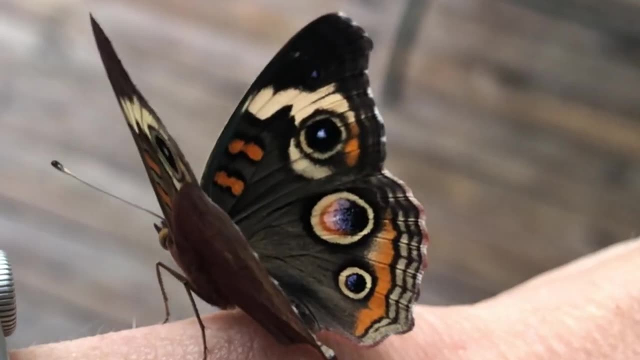 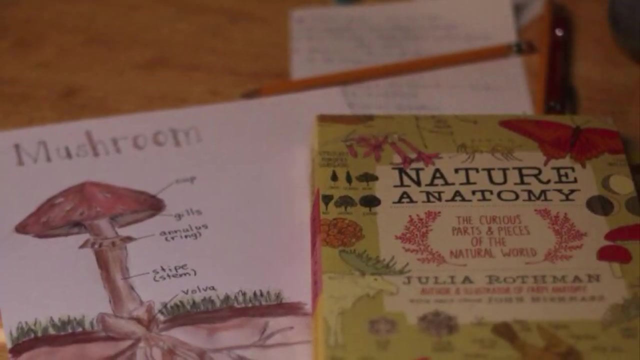 more intimate relationship with the natural world, observe and truly get to know something from the observations. And what I realized was that I wanted my children to have both types of knowledge. I wanted them to have the book scientific knowledge that we're all used to, and I also wanted them. 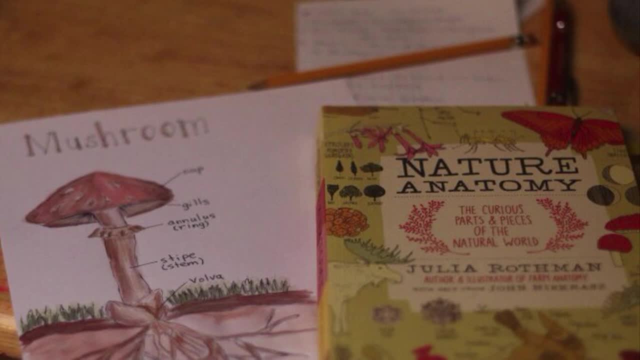 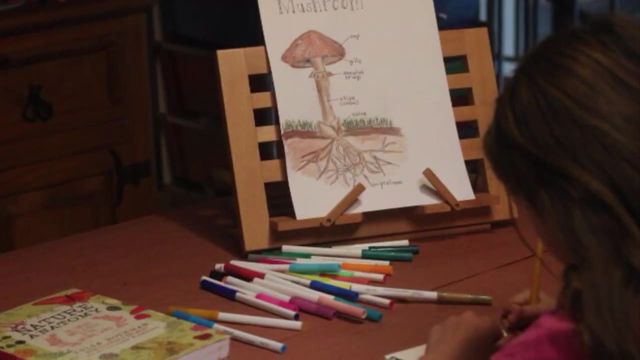 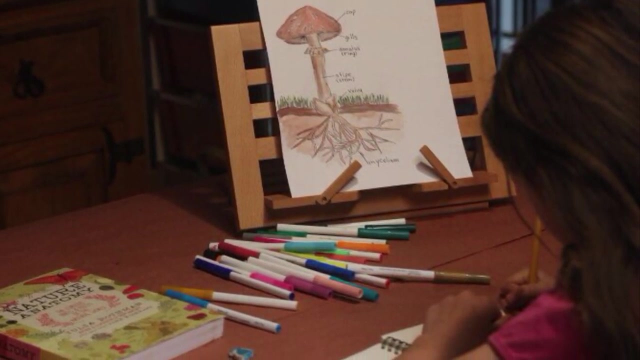 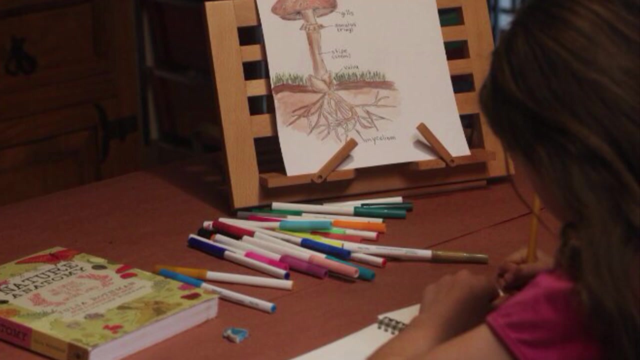 to have the experience, the intimacy with nature, the connection with nature and nature journaling is the way that I did that. it was one of the primary goals for nature journal was that connection with nature. the other goal that I had was that I wanted to cultivate an awareness of what was around them, so when they 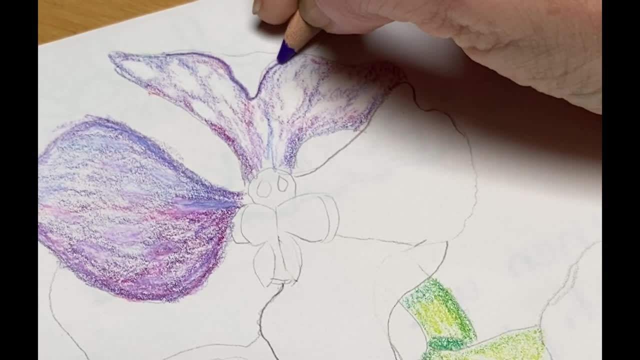 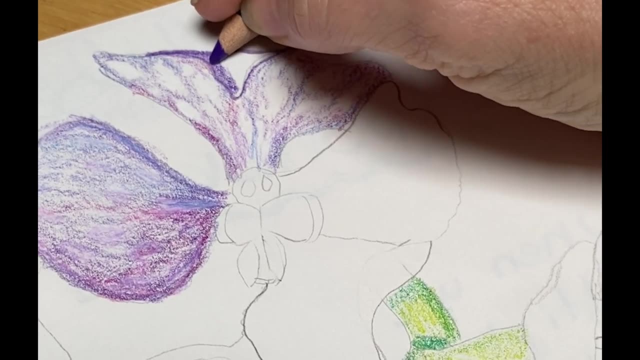 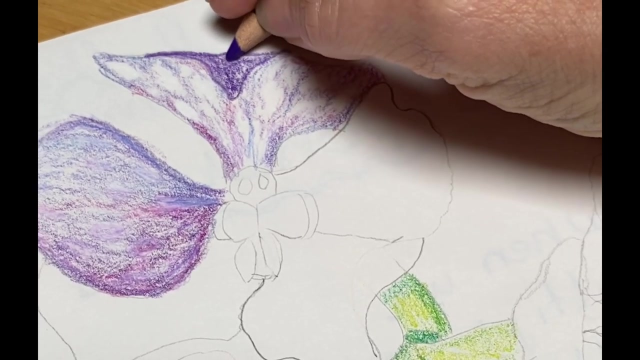 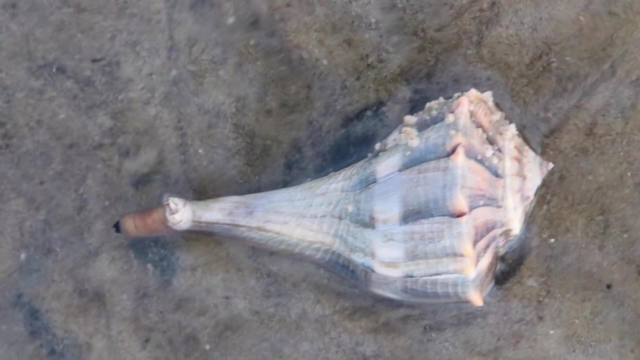 were out in nature. I wanted to. I don't even know if you cultivate it, it's more like encouraged because it's already there- that level of curiosity and I wanted to encourage that awareness of what was around them, to spark that curiosity or maintain the natural curiosity that is already there. I also 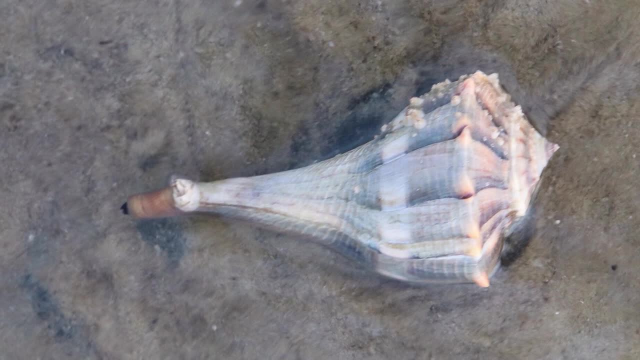 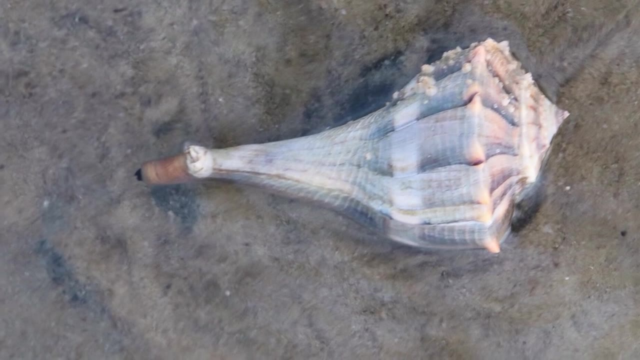 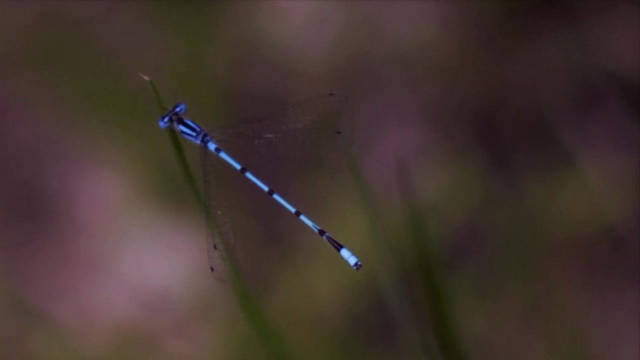 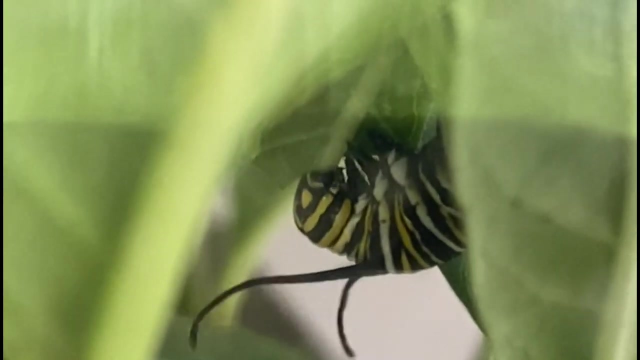 wanted them to have an understanding of life cycles and, dare I say, enjoy being out in nature enjoying life, taking in the fullness. we're very outdoor family, we really enjoy being outdoors and I wanted to cultivate that. in addition, I wanted them to be able to identify and know several different 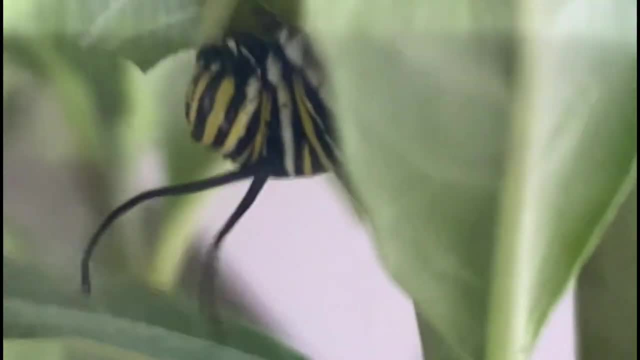 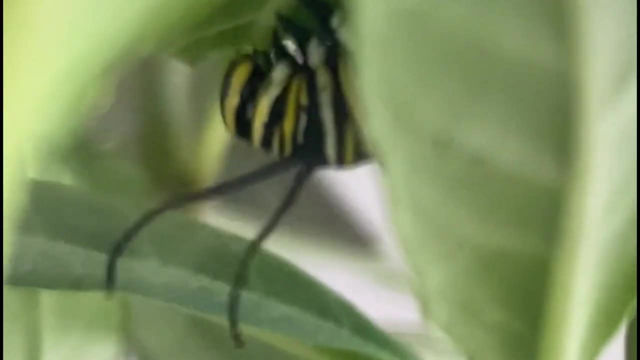 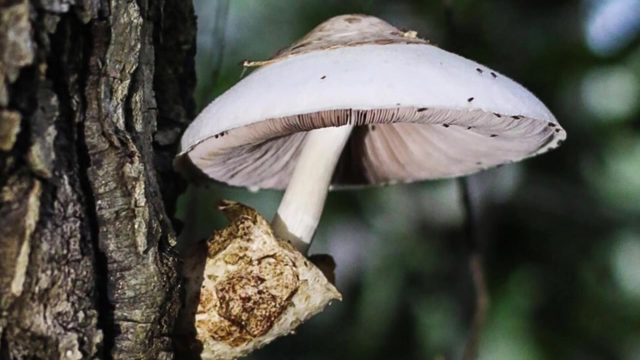 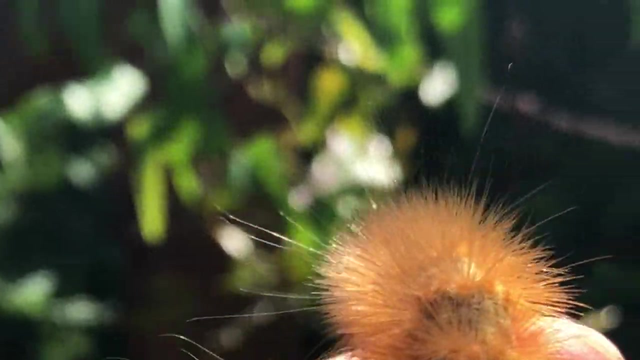 species within our area, like understand the ecology a little bit, know so many birds, so many plants, understand how they rely on each other. and before I move on, I also want to acknowledge that different families have different circumstances, different levels in nature, and that will direct how you do. 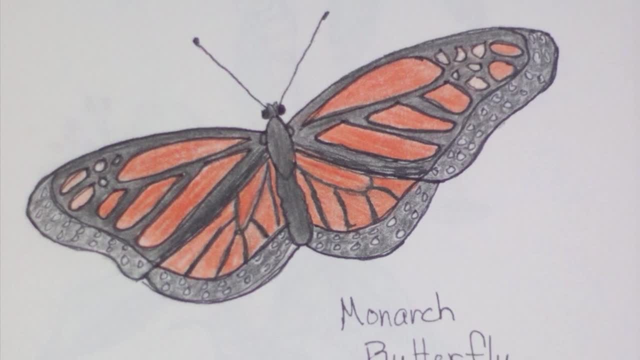 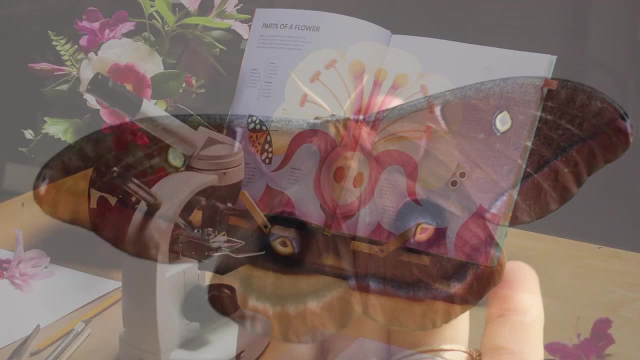 nature and how you do things in nature, and that will direct how you do things in nature and that will direct how you do nature study, if you include it. for instance, we all live in different climates, so some of our climates, and summer, are not conducive for going out. 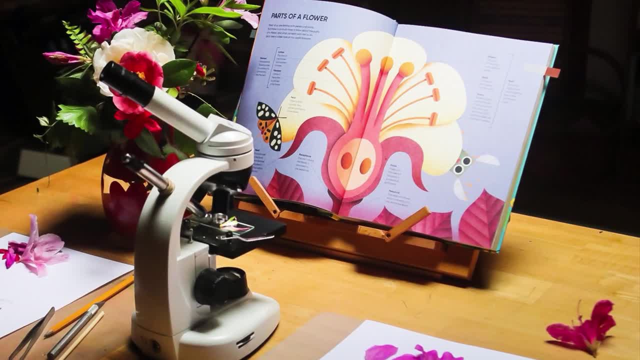 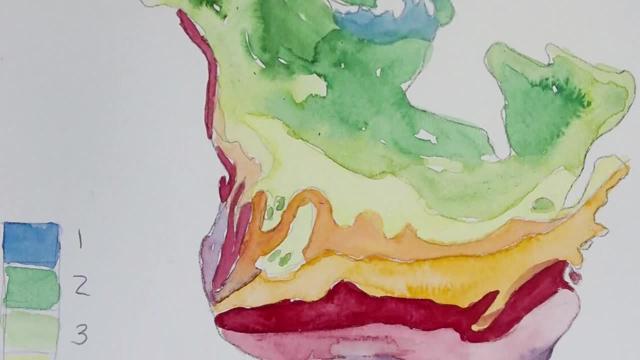 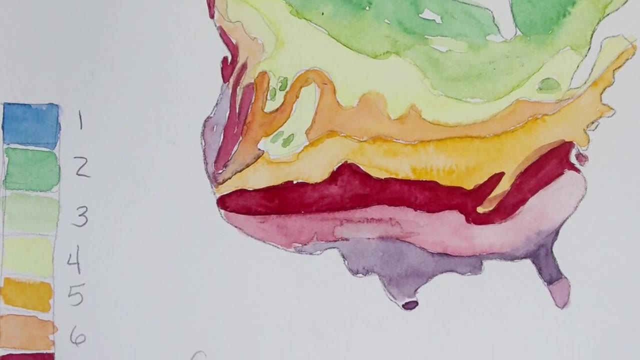 in nature some of our clients in winter makes it really challenging to go out in nature. the other thing is that we all have different abilities and different tolerances. in the bayous of Louisiana, when the mosquitoes are horrific, no one. tolerances in the bayous of Louisiana, when the mosquitoes are horrific- no one. 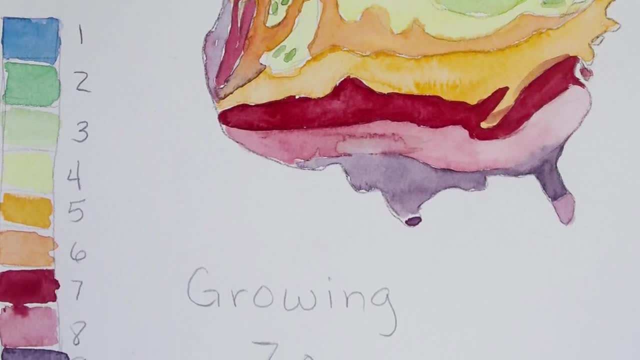 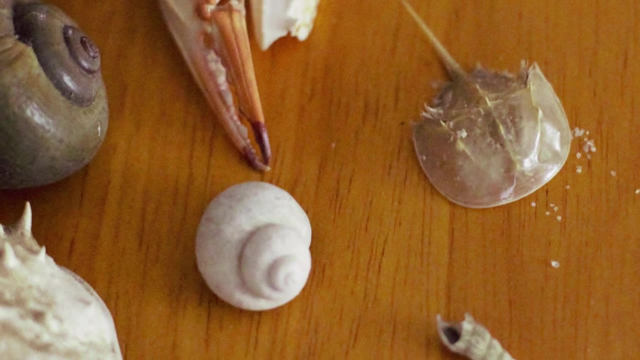 expects you to go out in the summer: get eaten alive by mosquitoes to go nature expects you to go out in the summer. get eaten alive by mosquitoes to go nature. journaling: that is not a pleasant experience. some of us have asthma. and in journaling: that is not a pleasant experience. some of us have asthma and in 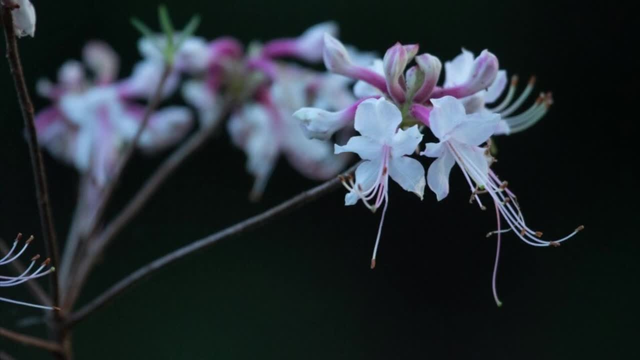 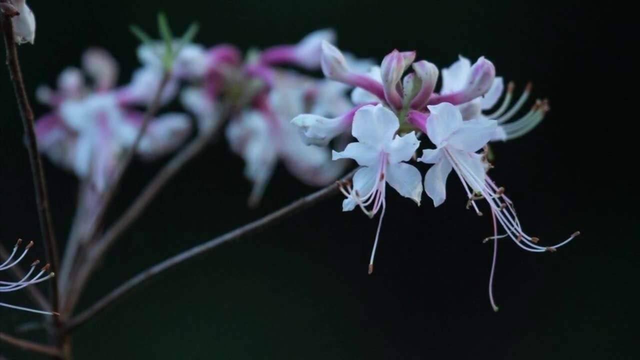 the spring instead of being an enjoyable experience watching everything bloom. and the spring, instead of being an enjoyable experience watching everything bloom and come to life. it's a miserable experience, so I want to also give some. come to life. it's a miserable experience, so I want to also give some. 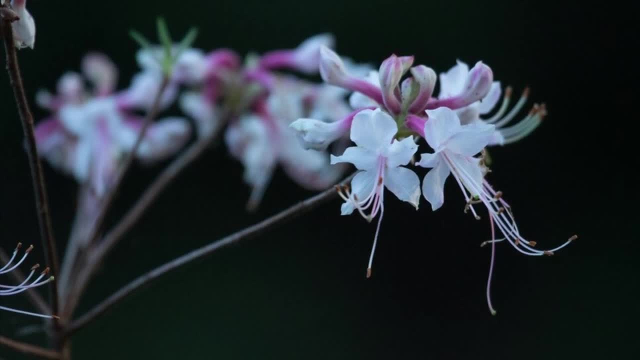 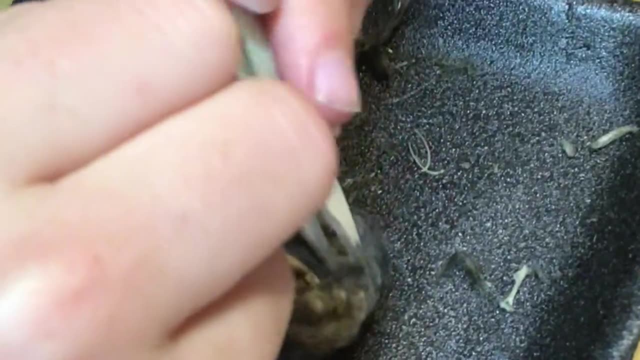 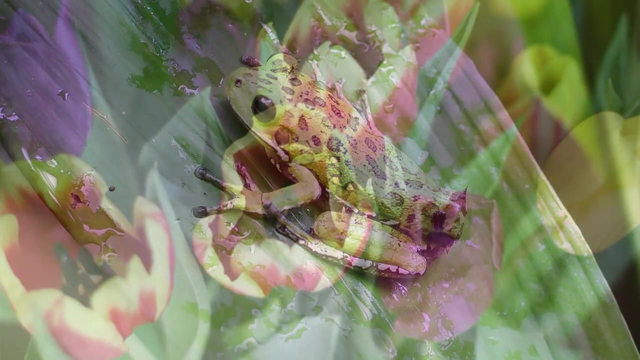 alternatives. it doesn't always have to be outdoors. I know that sounds alternatives. it doesn't always have to be outdoors. I know that sounds counterintuitive, but you can do a study each week of an animal or a lifecycle or some other project that's indoors. it doesn't have to be every season. it can. 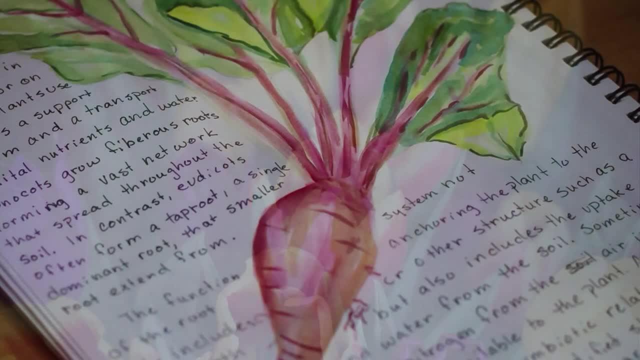 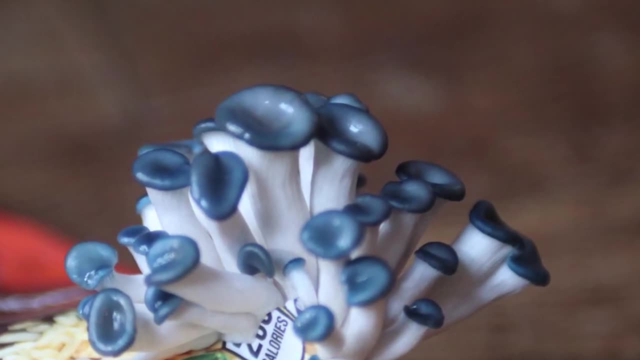 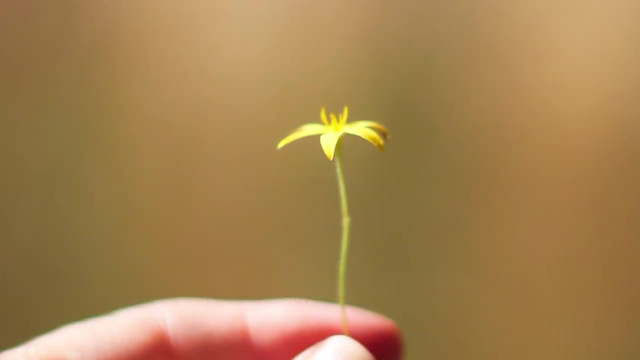 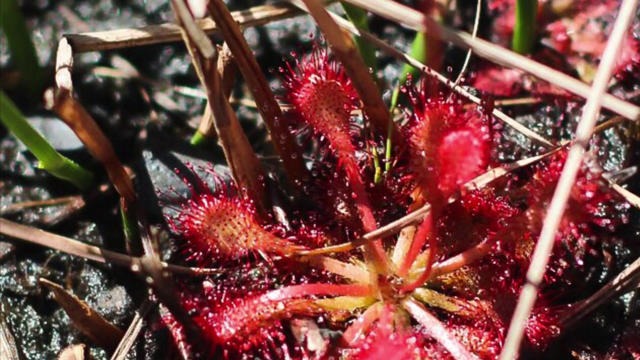 be seasonally that you do your nature studies. it doesn't have to be in the depths of some remote area. there's plenty of nature right outside the window, right outside the city park, or even if you're eating outdoors at a restaurant, you will see little finches and wrens that come to pick up the bread. 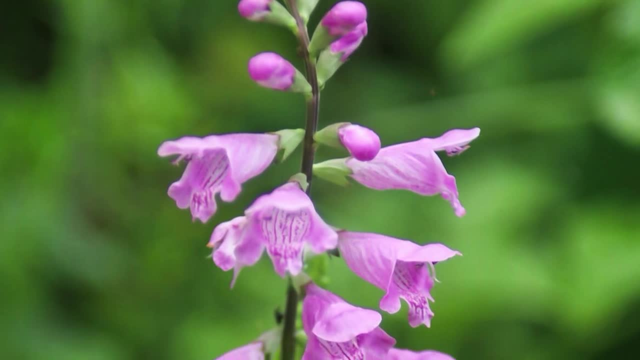 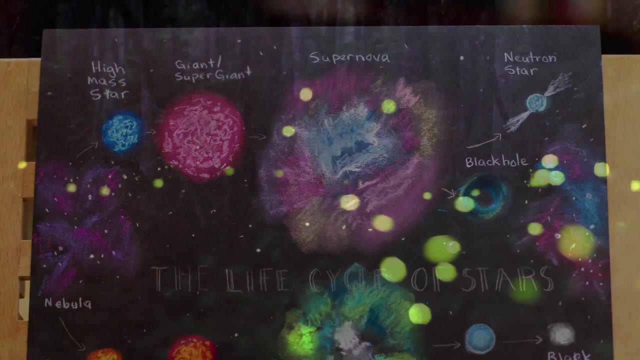 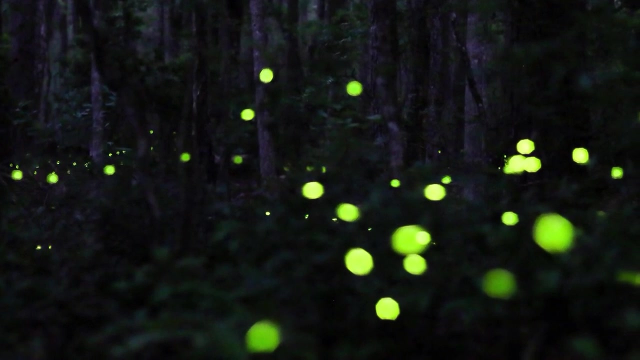 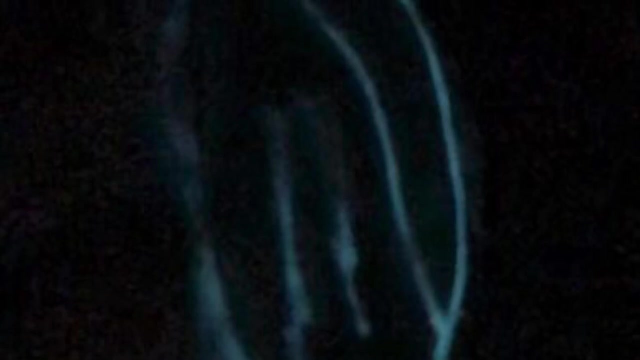 crumbs. nature is everywhere and I want to give a shout out for doing nature study at night, taking a look at the constellations, are the fireflies, the various owls that you can hear, the sounds. there's a lot to take in, even at night, so I want to expand the idea that we all have to go on these. Charlotte Mason. 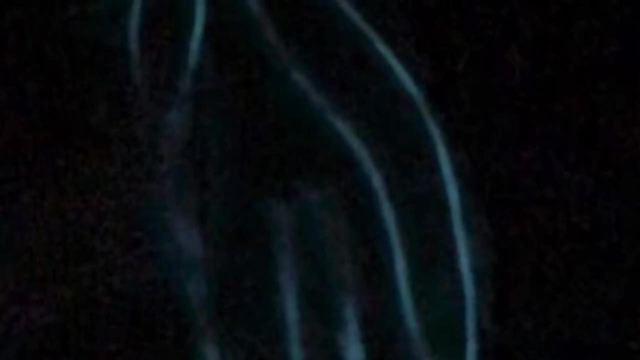 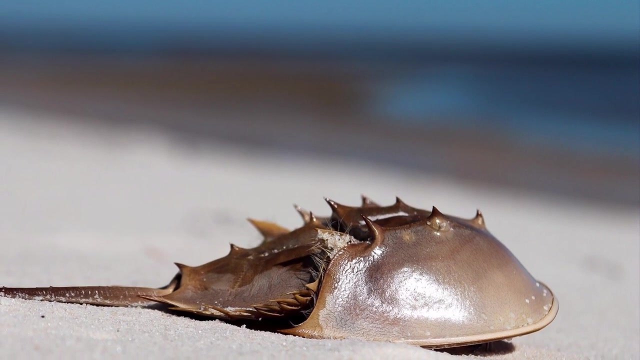 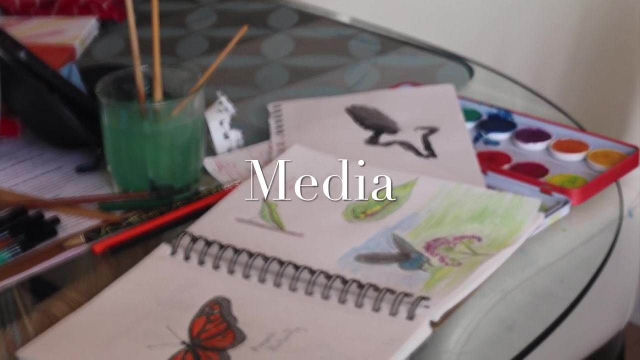 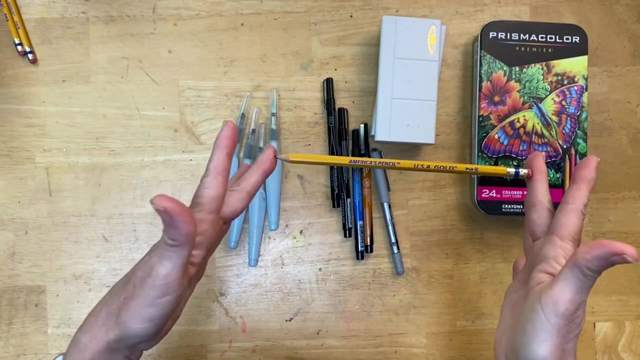 nature walks out in nature every week for nature journaling. nature journaling can be much more than that and I hope to show you in that process. today let's talk about media that can be used. nature journaling really only requires some kind of writing utensil right to 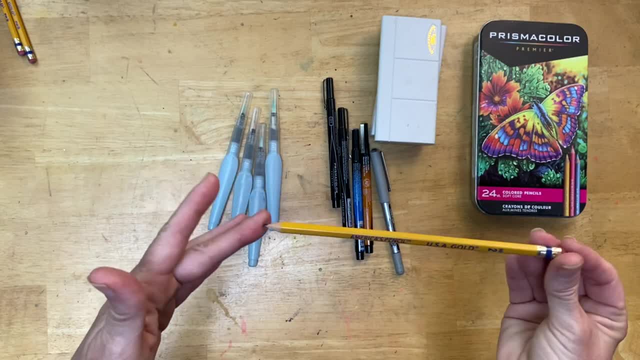 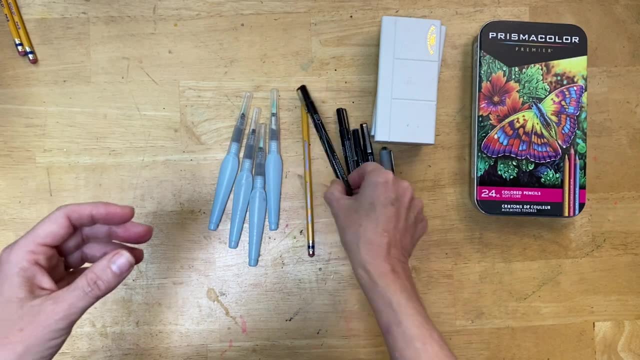 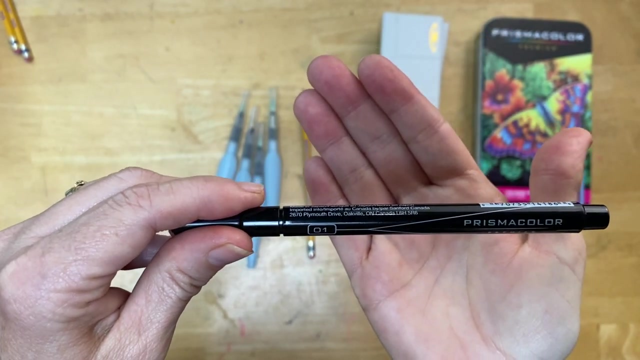 record stuff in your journal. but here are a few other things that you could add that will spark a little color and make your pictures a little more interesting. we use fine point pens. these are from Prisma color. you don't have to have Prisma color, they're okay. they're not fabulous. 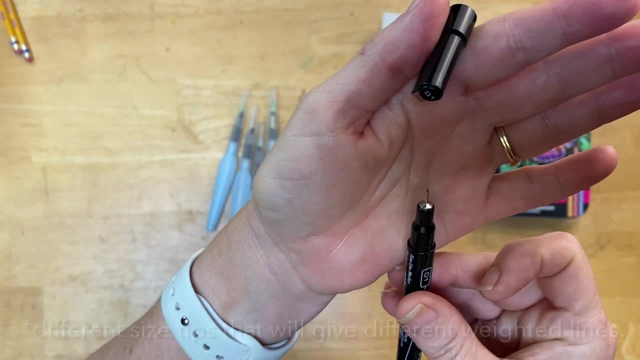 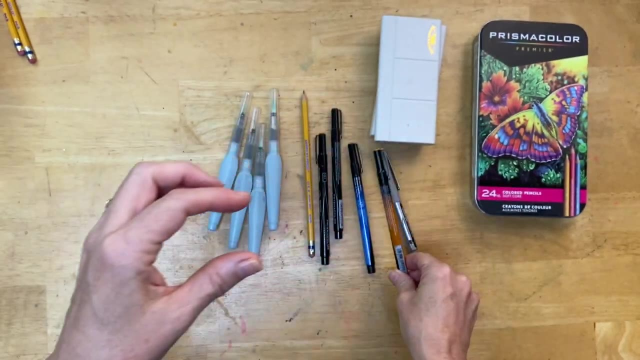 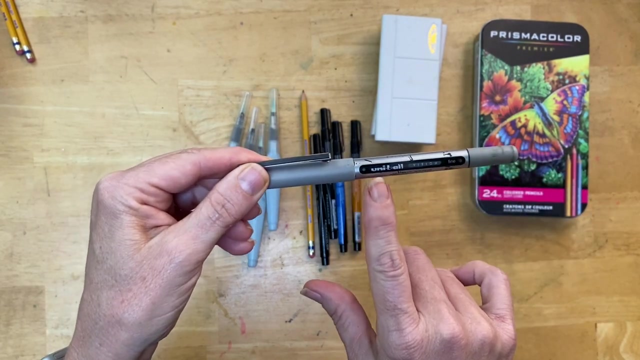 and they have different size pens that will give you different lenses. they also come in color, which is nice. we have those and of course, a regular ink pen is just fine. I will note that some of the ink pens are water soluble, so once you draw on them, if you. 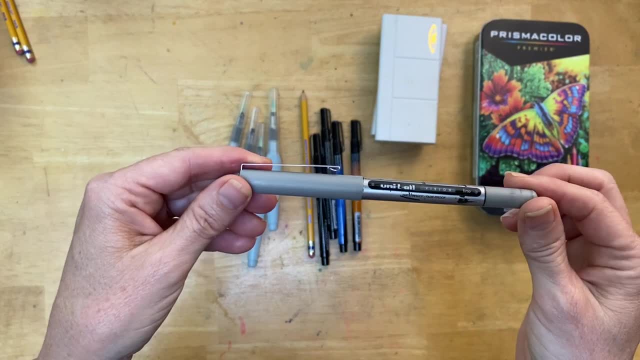 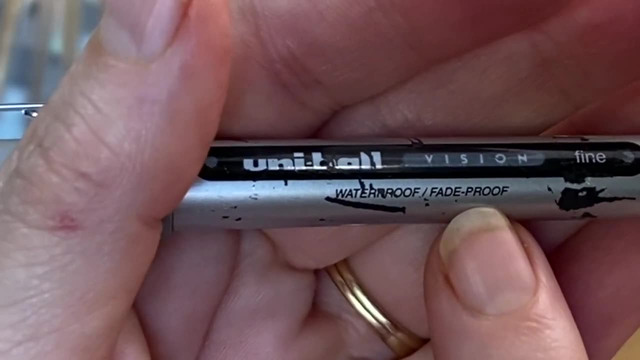 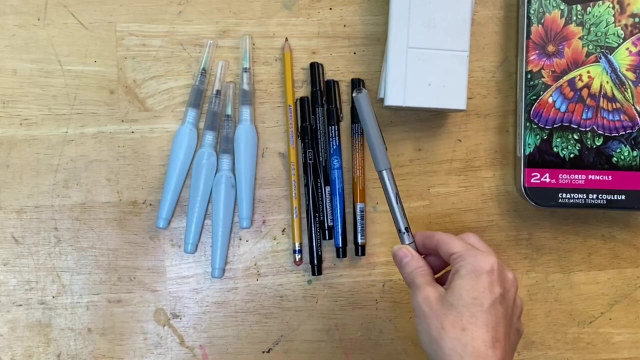 use watercolors, it will smear, so you want to make sure. for instance, this says: this is an old pin, that well, it's waterproof and fade proof. but of course again, those also come with their own challenges, particularly if the young child gets a hold of it. and then we have travel. I'm a little embarrassed to. 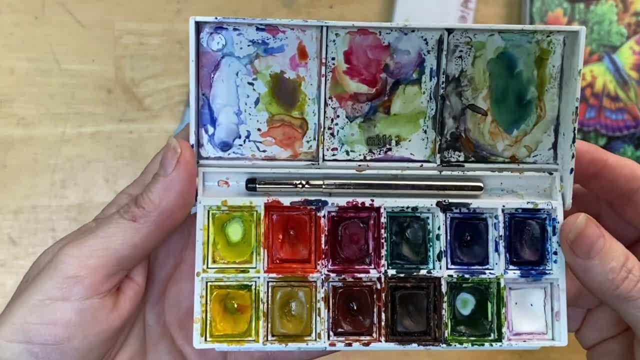 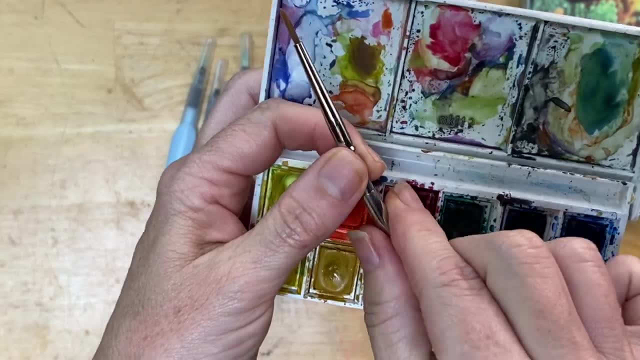 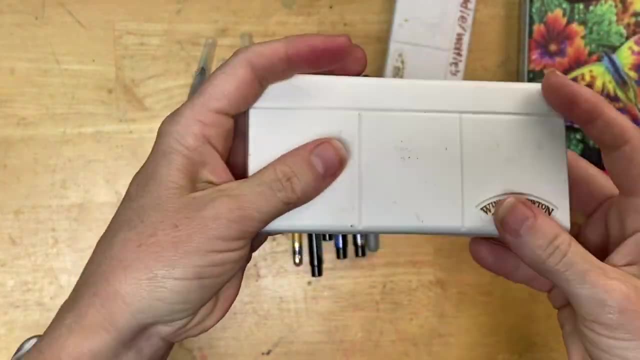 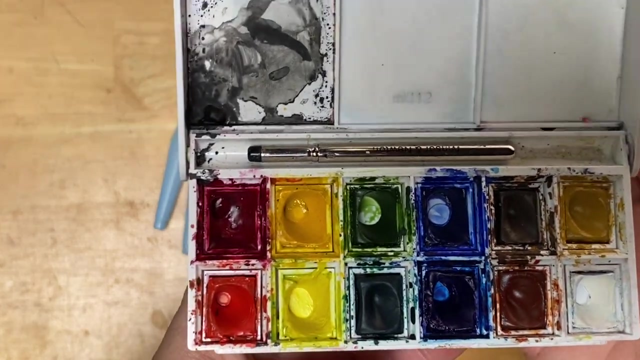 show you. this is my travel watercolor set. I'll leave a link for you with that. it does come with a brush which you can use, or I'm going to show you other brushes as well, but I want to show you my daughters, because she keeps hers extremely neat, much better than me. 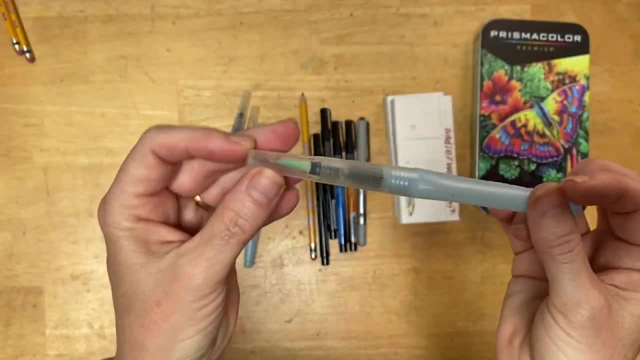 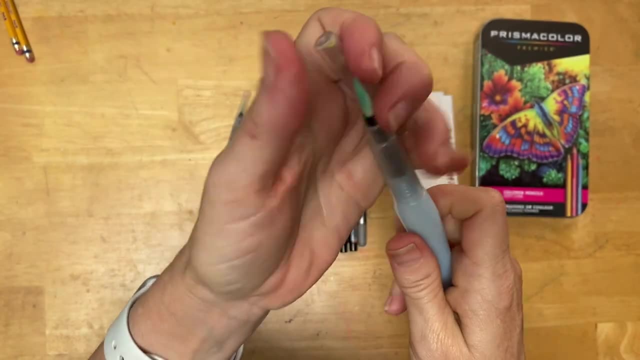 they have travel brushes and these work slightly different then other brushes. I see they twist incorrectly, so these twist off and you can place water in here. it does take a little bit to to put water in lunch boxes, but you don't see it in here. new, easy way to mix it with water instead of using whetstone, but I know. 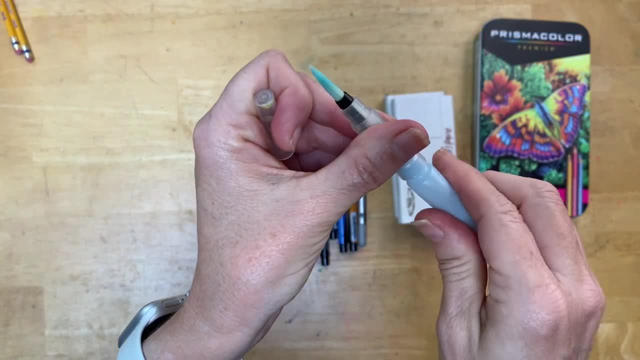 that there are some patterns in this. when you are looking for a watercolor set that works randomly, you can do the same thing and you can choose which. byOh, there's impossible tools. I can't. It does take a little bit to get used to because these work slightly different than a normal. 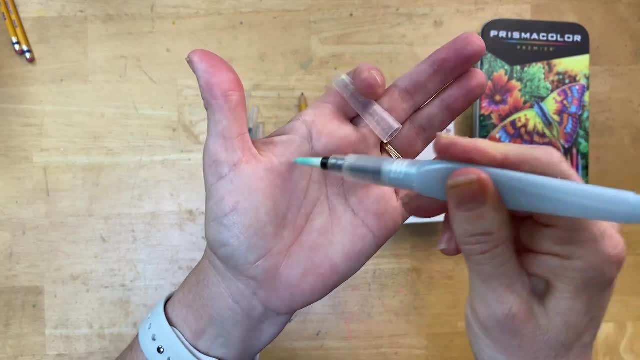 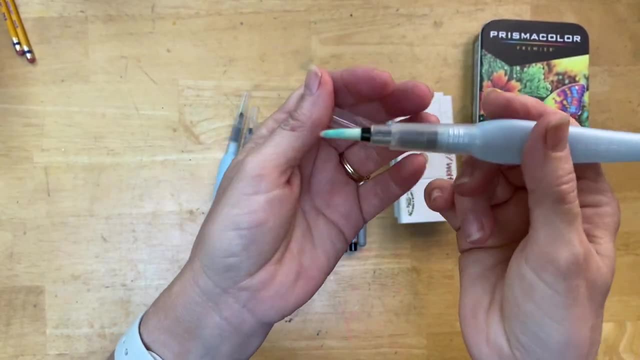 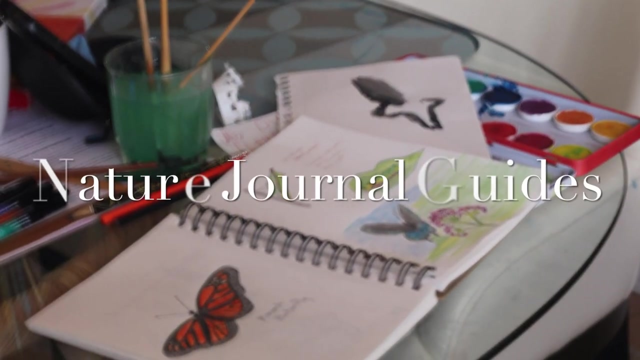 watercolor brush. To wash out the color from the brush, you squeeze it on a piece of paper until all the color is removed and then pick up your next color. So it takes a little bit of getting used to. It's slightly different than the other watercolors. 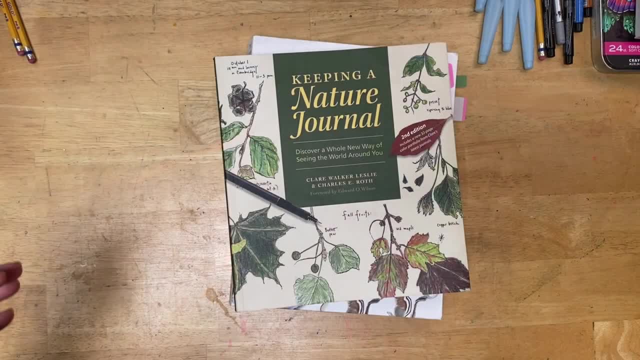 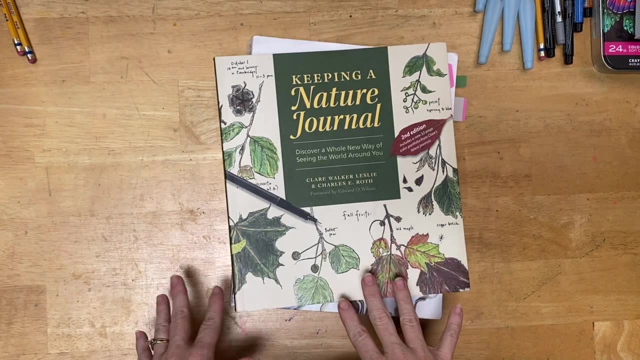 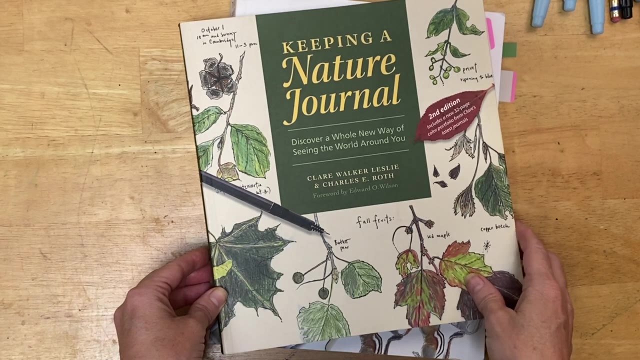 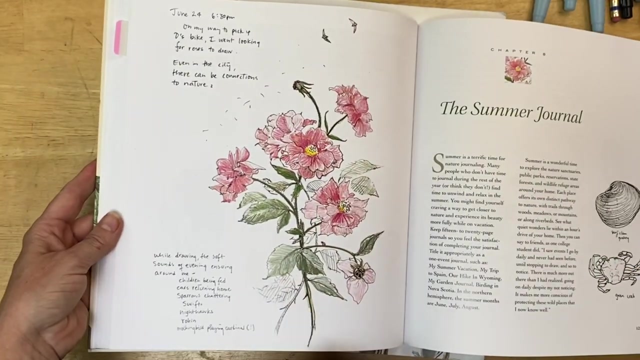 I want to show you a couple adult resources and then some children's resources for guides and nature journaling. I have two resources for nature journaling. One is Keeping a Nature Journal. This is by Claire Walker Leslie, And what I love about this is that it has examples of her nature journaling. 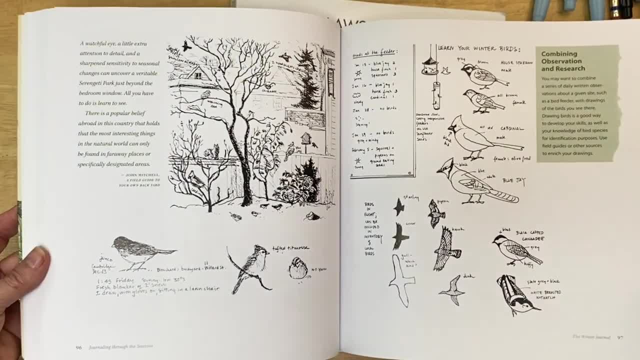 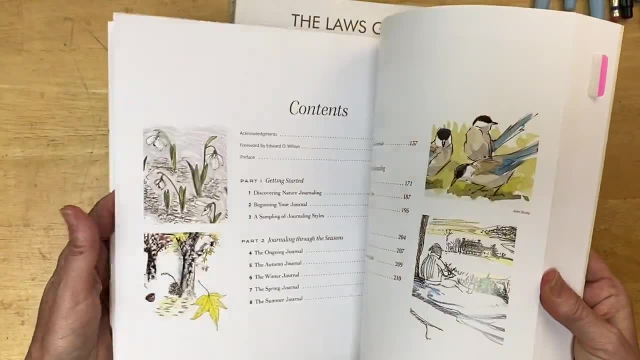 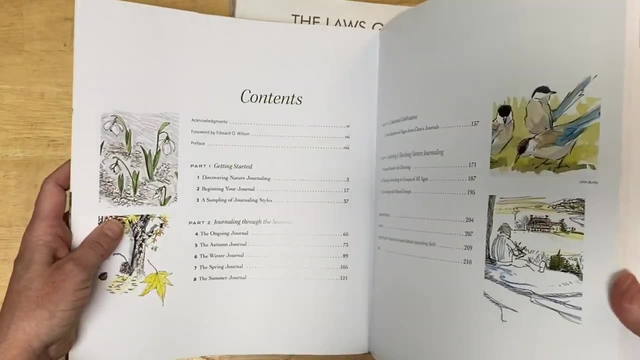 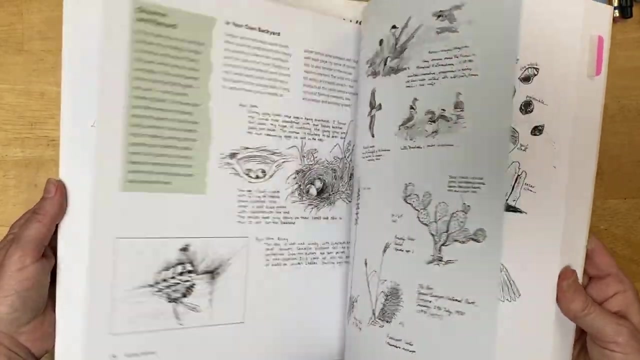 And some of it is quite messy, Which I love Because it's realistic in what is actually done. So she goes through this book, arranged by Getting Started and then The Seasons, And she gives examples. It is a pretty dense book to read through. 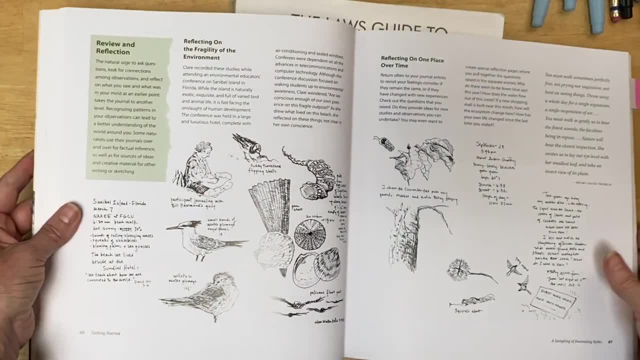 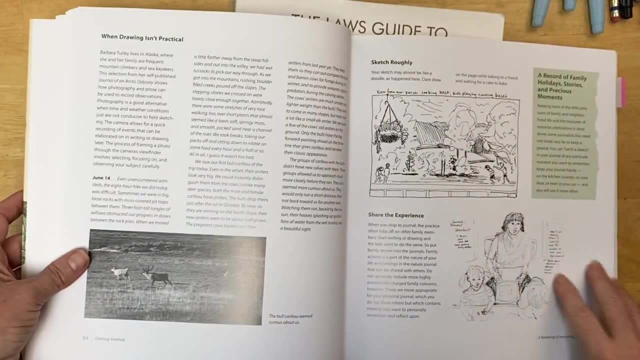 But I think it's fabulous to get some of the examples of her journaling And that our journaling doesn't have to be perfect, Because if you feel like you're not a wonderful artist, then it can be a little bit intimidating, But it doesn't have to be. 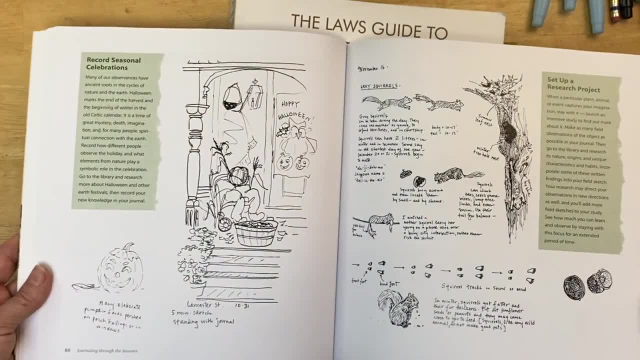 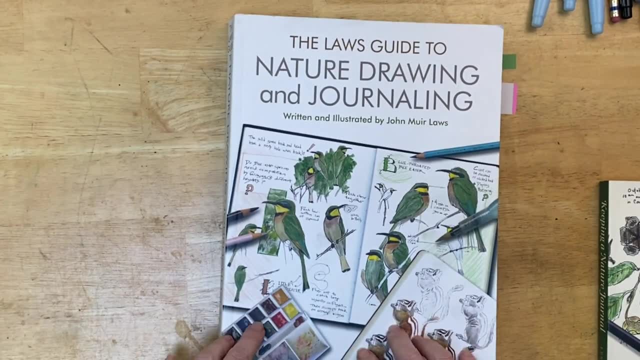 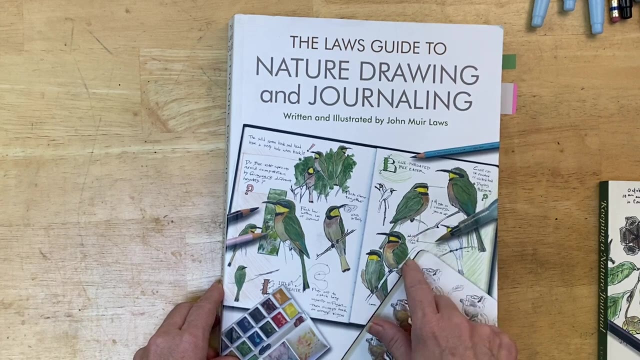 There's lots that can be included and we get better with practice. The next book that I want to show you- and I'll leave you a website that a member shared with me last week or a couple weeks ago that John Muir Law did on teaching nature journaling: 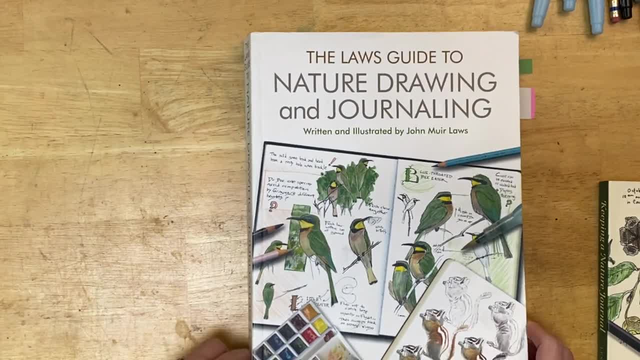 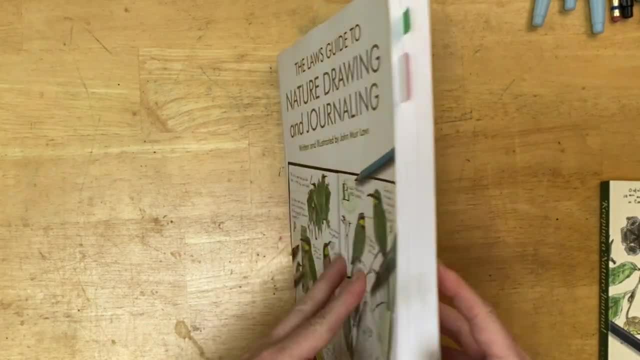 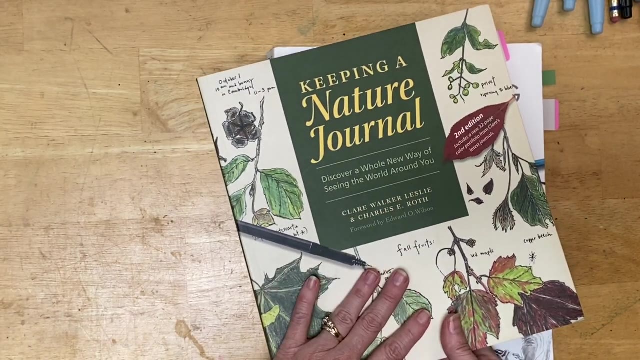 He is absolutely fabulous in nature journaling And this is his book, which I love. Again, it's fairly dense. This is a very different type of book than this one. I feel like this gives you all kinds of examples of what it can look like that are realistic. 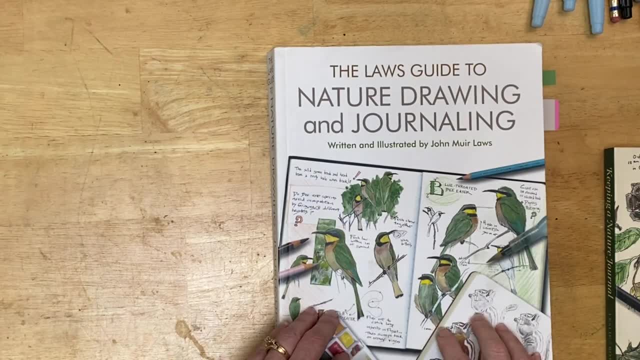 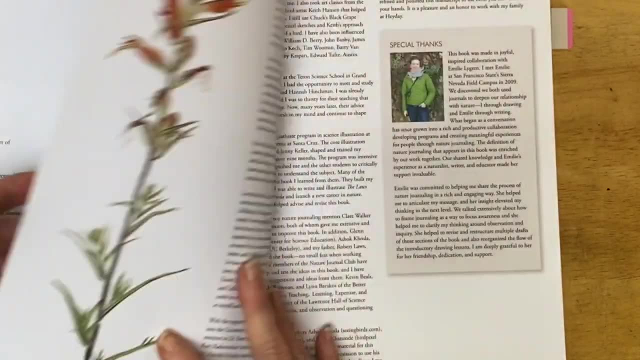 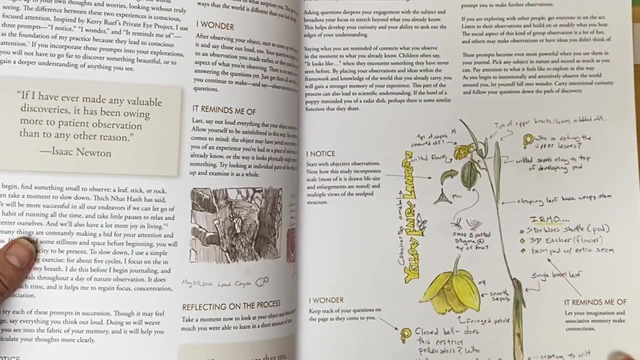 And also takes you through the seasons. This one is a drawing guide for the most part R The Table of Contents for Nature Journaling. For this one, And what I love is it goes through the normal kind of what nature journaling is. 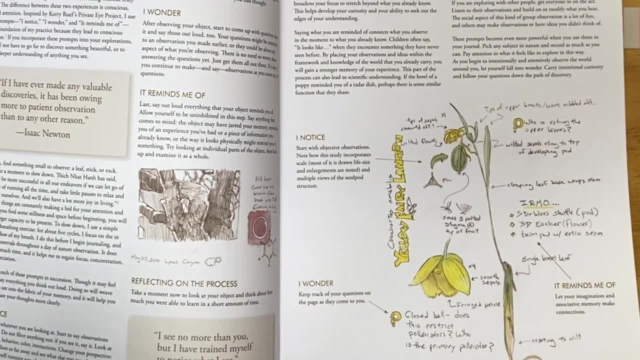 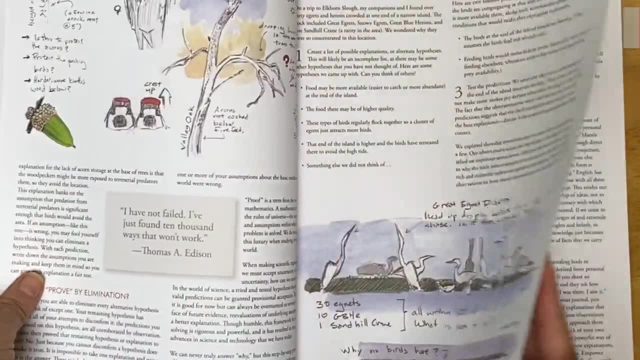 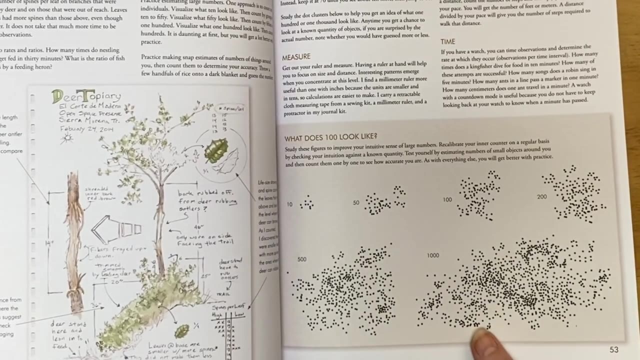 What media you can use for nature journaling, Things to notice and so forth, But it is a step-by-step guide for drawing. This is one of the things that I love is the data collection. It shows you different ways of collecting data. 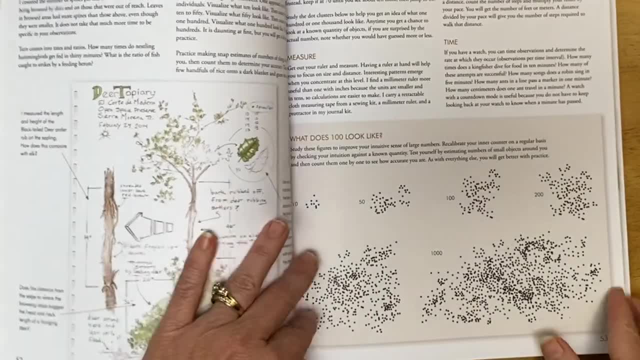 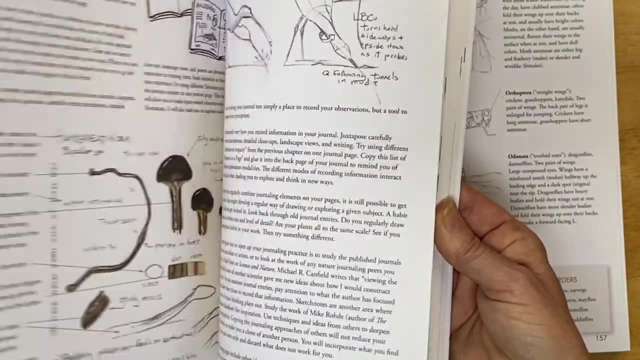 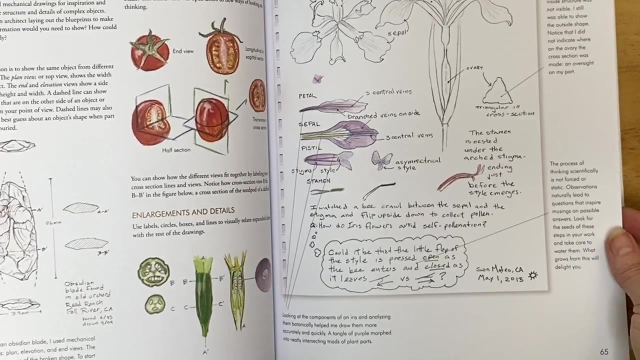 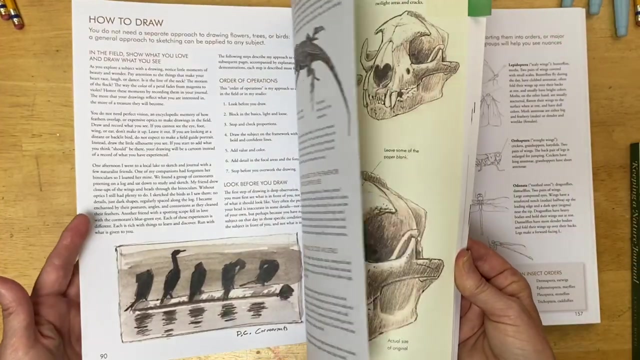 And it does have a few examples here as well, which I like. But what I really love about this is that it goes through and gives you very explicit details and teachings on how to draw. Here is the section on nature drawing. So it starts out. 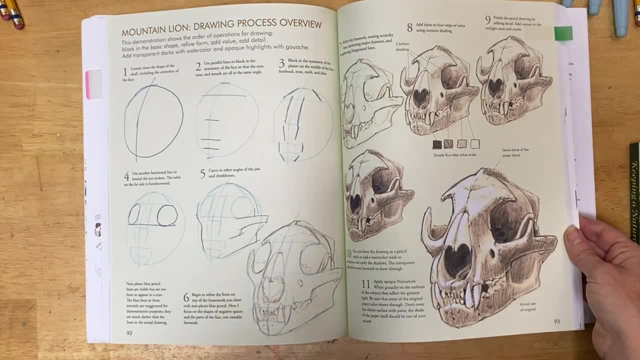 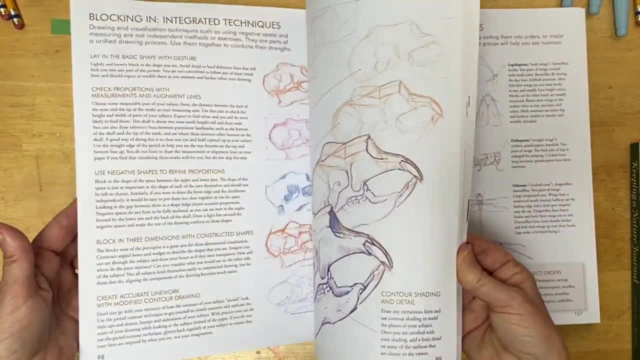 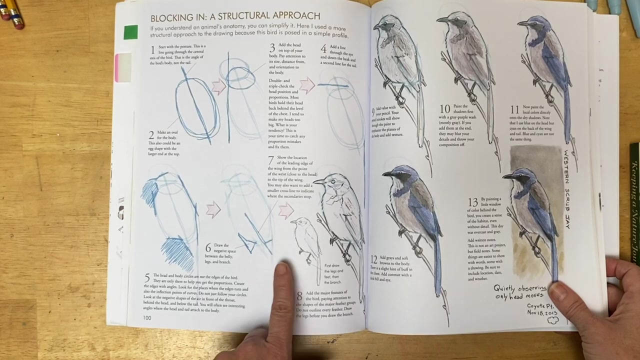 This one's actually complex. I'm going to go ahead and do that. Okay, But there are much simpler drawings in here. This is the skull of a mountain lion. There are step-by-step approaches for drawing birds in different positions, which is really. 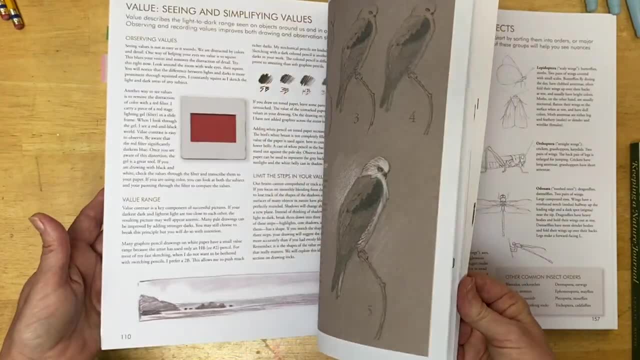 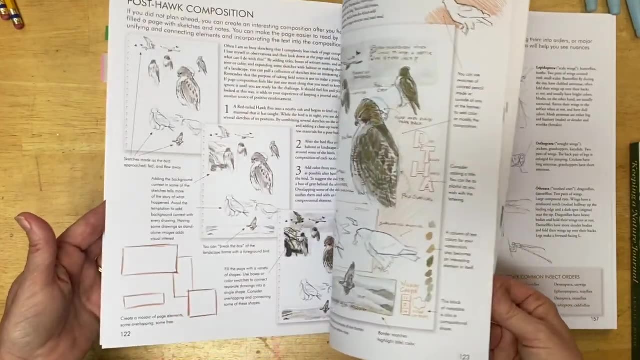 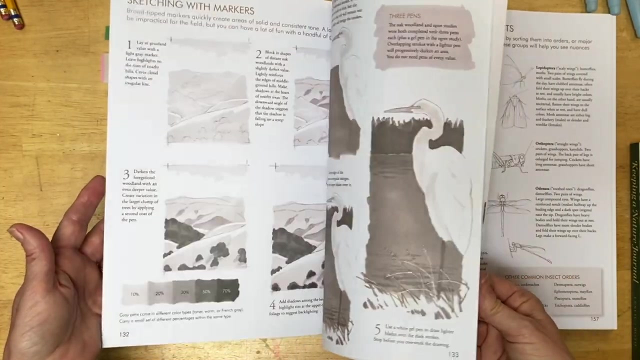 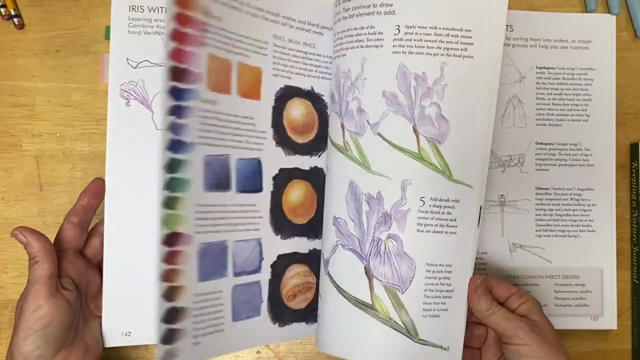 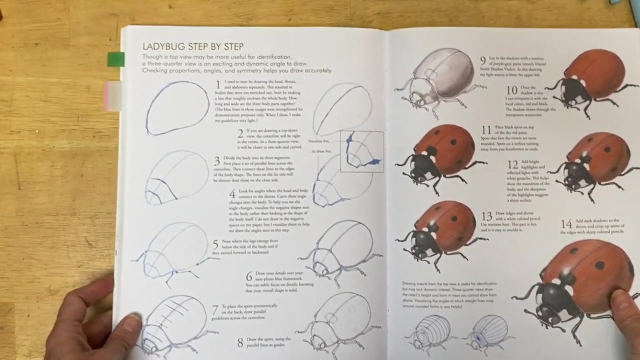 nice. They also have insect drawings, landscaped drawings, but it goes through and teaches how to estimate Proportions and how to draw based upon those proportions, For instance, on the ladybug when we're looking here. he goes over how to find shapes out. 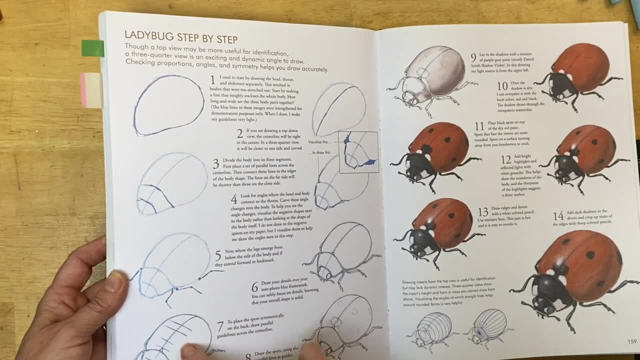 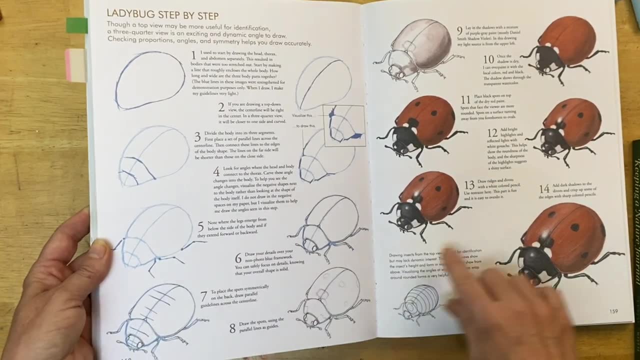 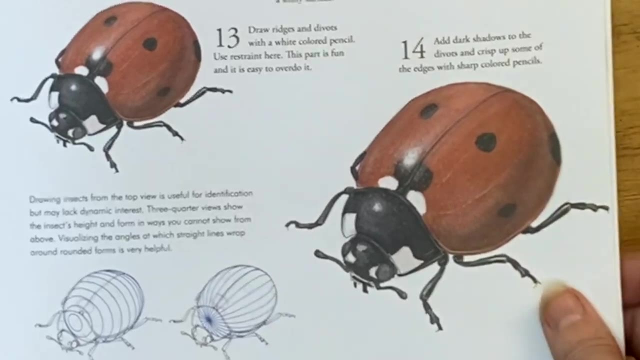 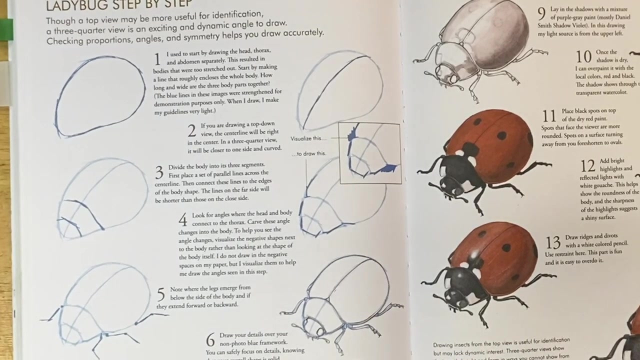 of the ladybug And what gives Depth to the ladybug, which are highlights, but also this rounded cross section. like you'll see, the brush strokes here are rounded, moving here. This adds depth. So this book is very good about giving proportions, drawing tips and talking about shadows and 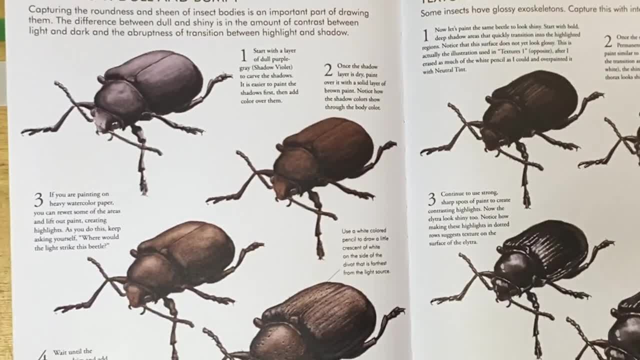 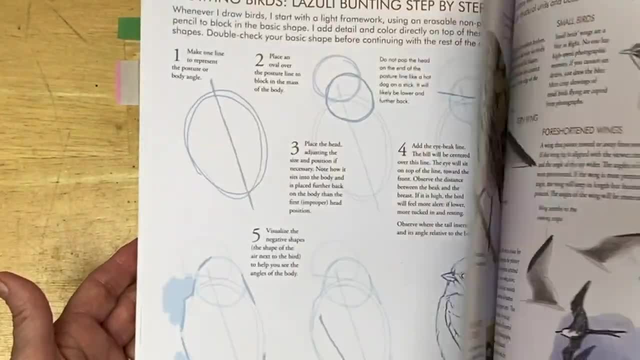 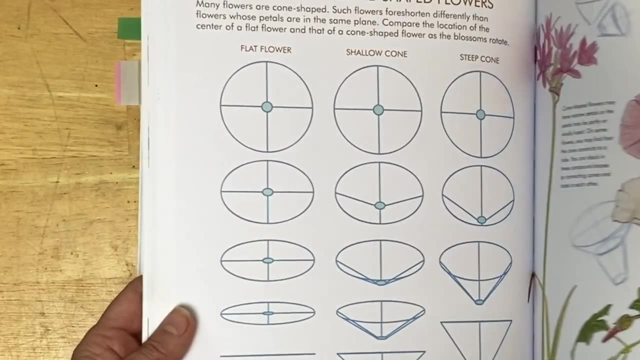 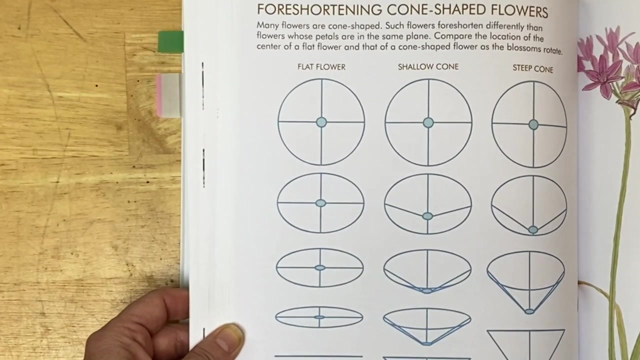 highlights and things that bring depth to a picture. So I really enjoy it. I really enjoy this book for its drawing and art skills, but it's pretty comprehensive. It does have a few examples- not a lot You can see here. it's talking about the foreshortening of flowers and the different elliptical and 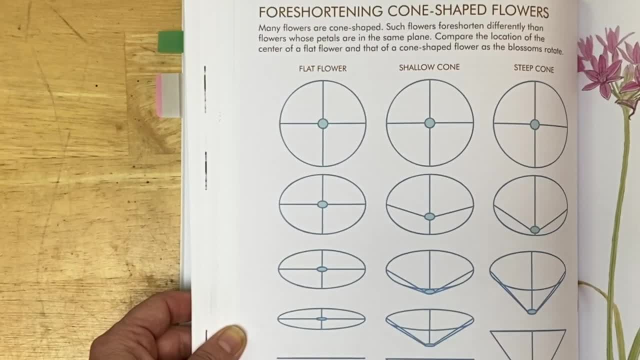 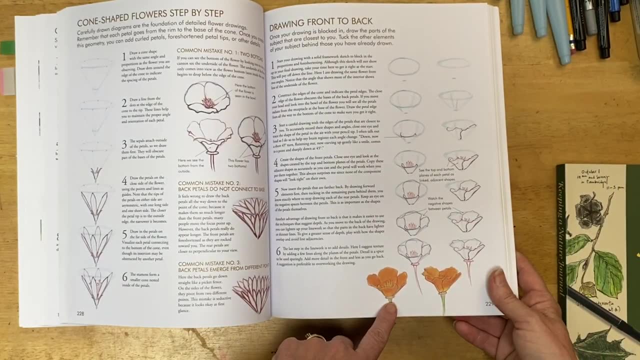 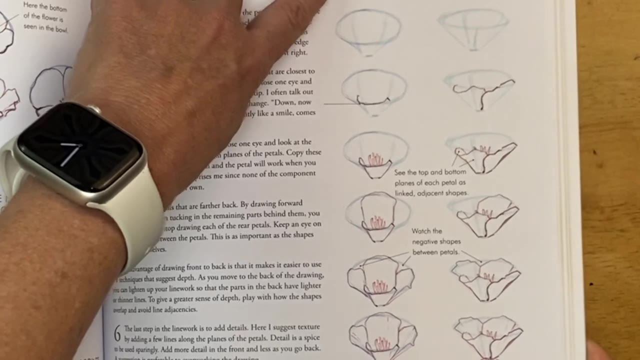 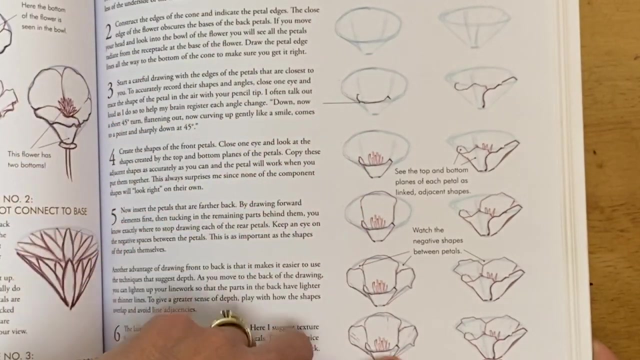 circle shapes that you can make depending on the flower that you're drawing. here They're drawing a cone shape- This is a poppy, I believe- And you can see the process of finding the view and what shape that has: elliptical shape and then the cone portion of the flower. 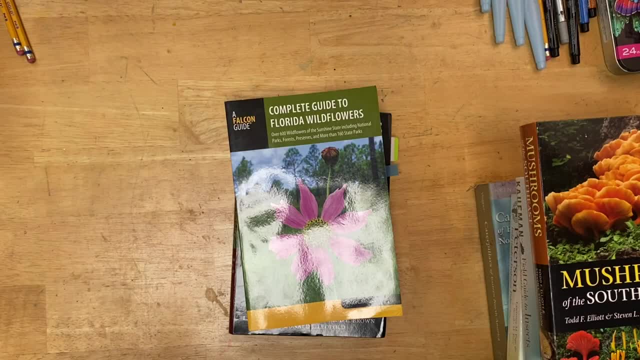 While we're on adult books, let's talk about field guides, which you're going to need if you want to identify plants, animals, mushrooms, various things out in nature. So let's start with the field guides. Field guides, Field guides. 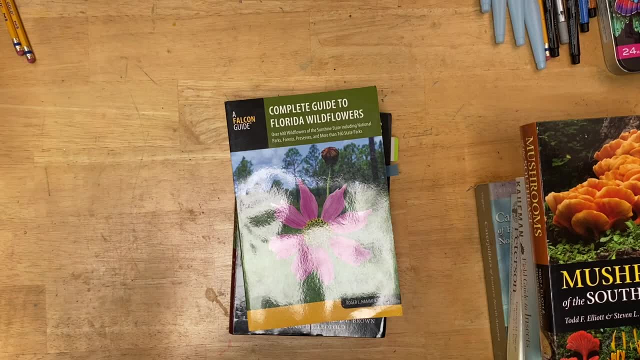 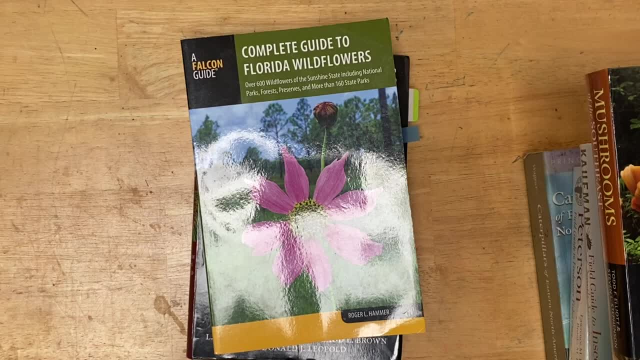 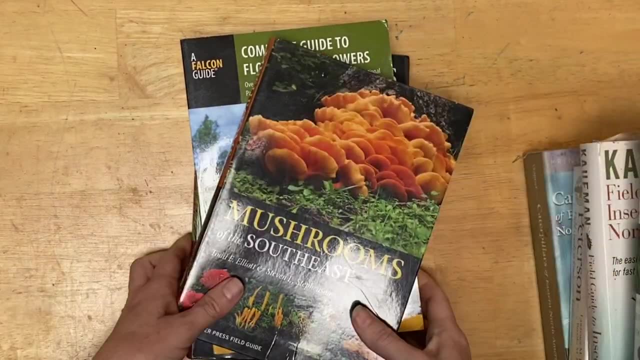 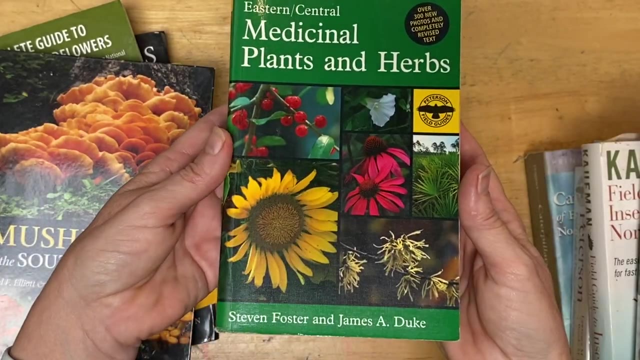 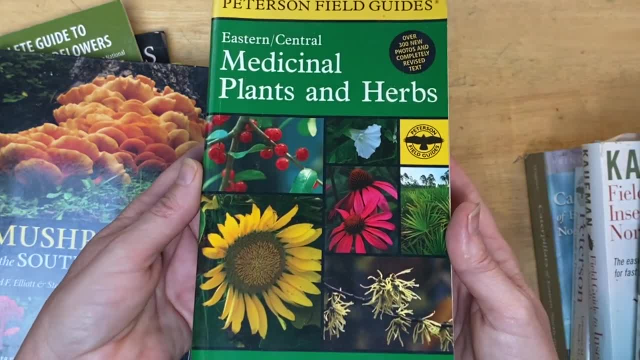 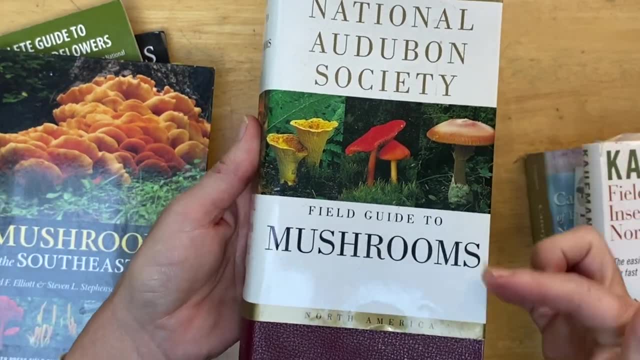 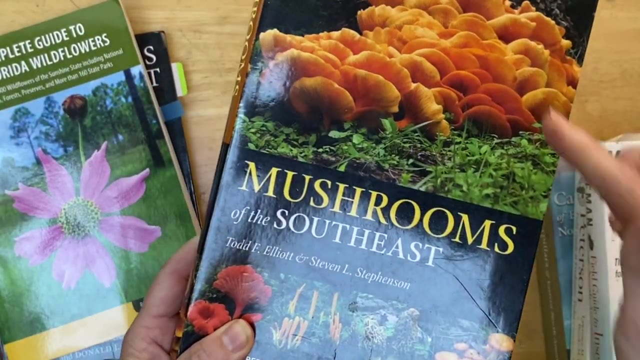 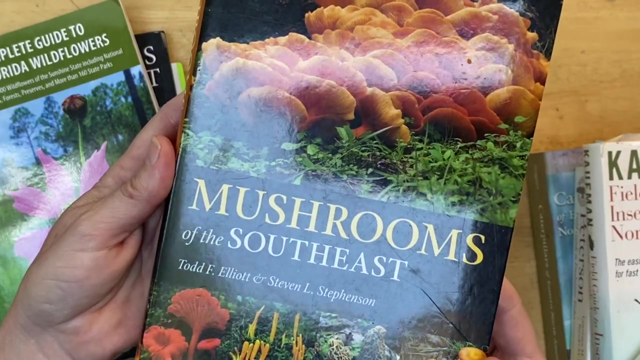 aren't as many specific to my area guides available for this, and then sometimes we have larger guides, like I have the Audubon's mushroom guide as a supplement to my native guide, native to this area, this our mushrooms of the southeast. if I could get one that said mother mushrooms of Florida, that was good. 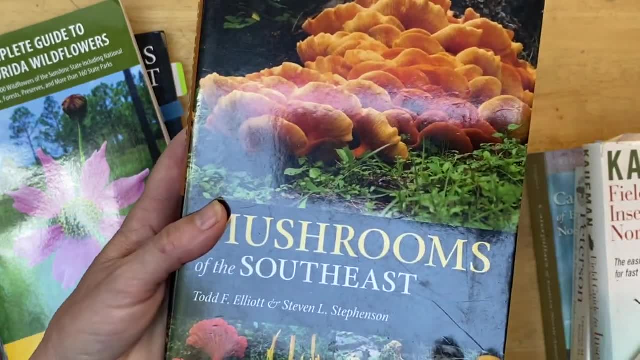 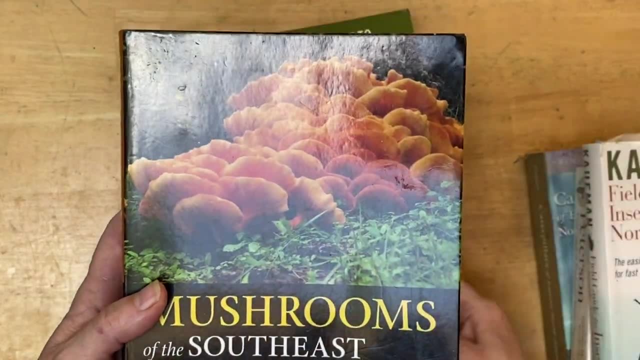 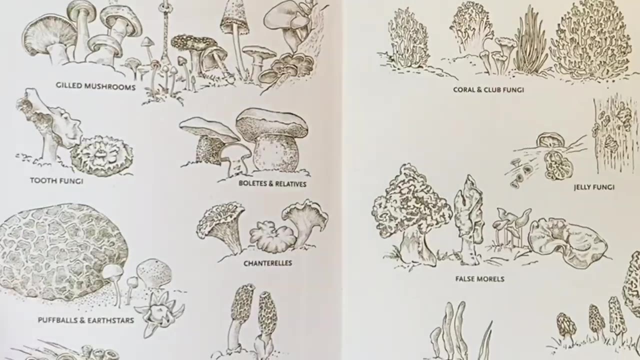 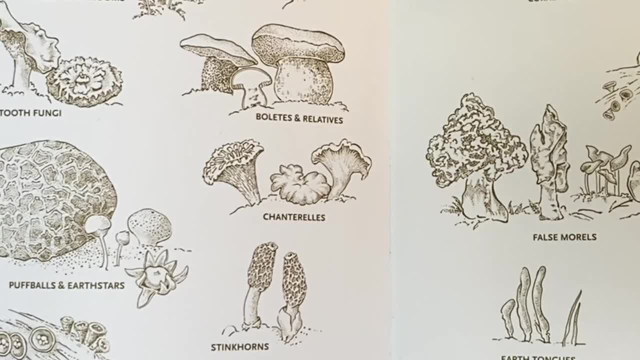 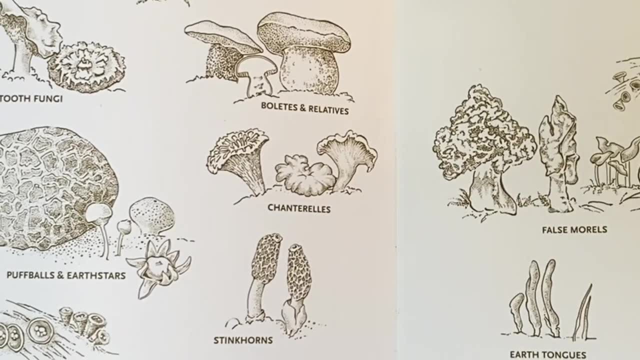 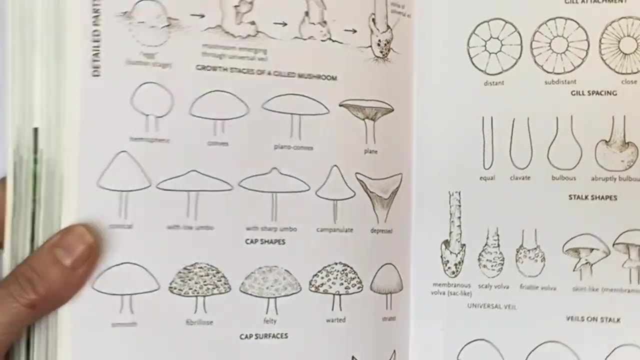 of your guide is the beginning of your guide is the beginning of your guide in various ways should have drawing and illustrations of filled marks or features that you're trying to identify. this is the mark of a really good field guide. so you'll see here, different features are drawn on the front and the 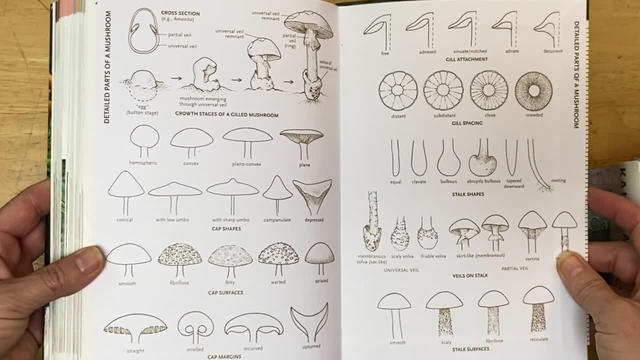 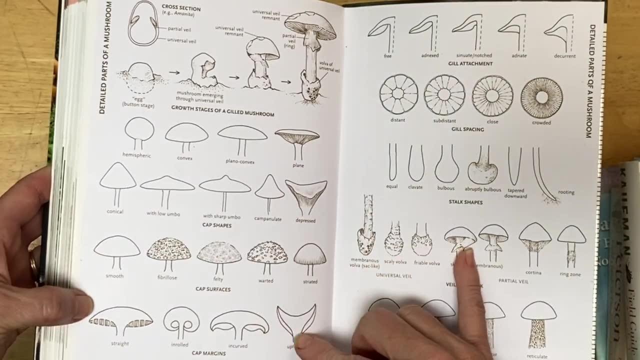 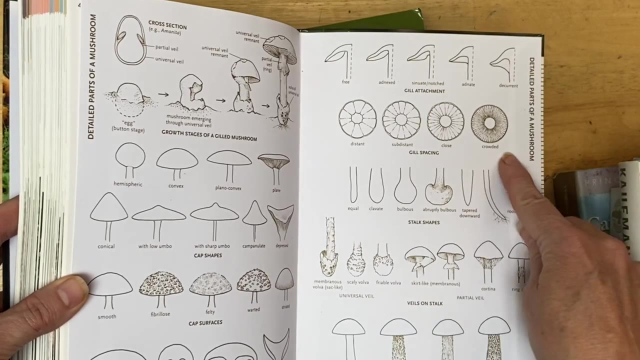 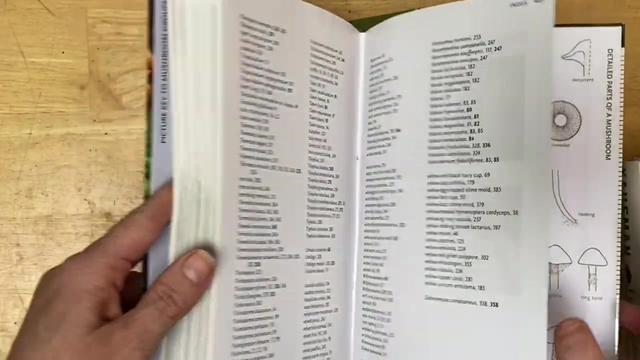 back. this is just various shapes of different kinds of mushrooms, and this is the different shapes of guild mushrooms and their caps. and then you have the different variations of the gills themselves, as well as the stalk shapes, the veins, like this is pretty specific. this is one of my favorite guides. a good guide is also going to have. 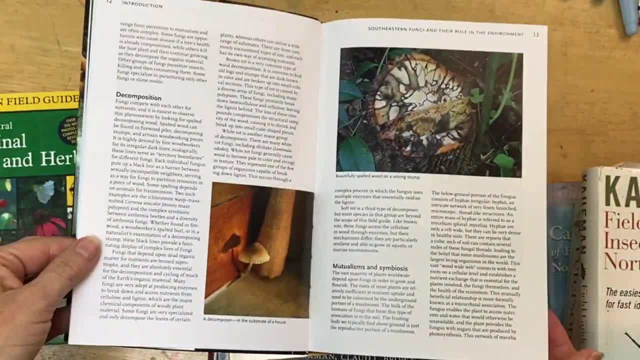 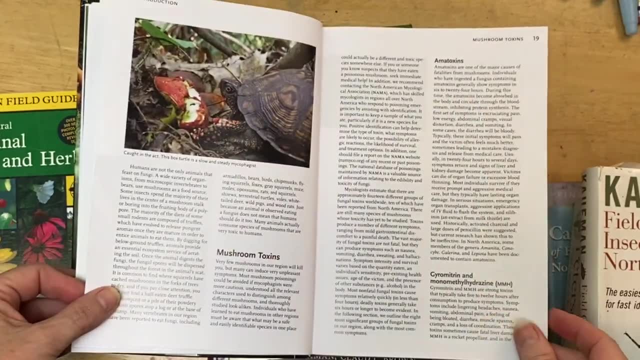 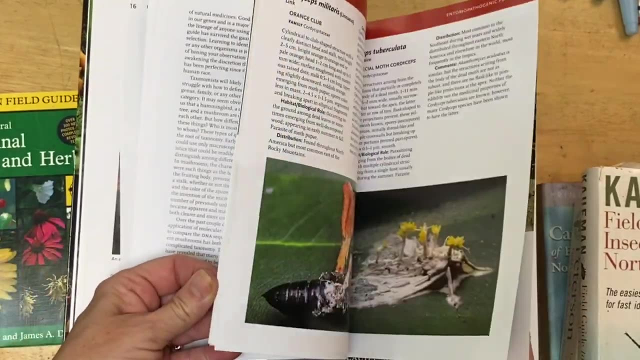 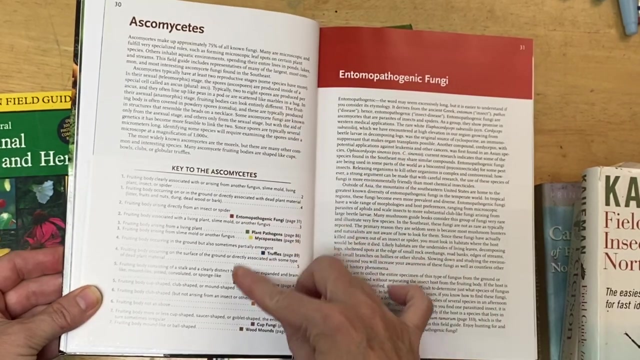 information at the beginning that will give you life cycle information, different field marks to look for what you can expect in your climate and ecosystem, and this one also gives information at the beginning of each type of mushroom that it goes through and has a key, and i love field guides that have a key. they can be hard to use. 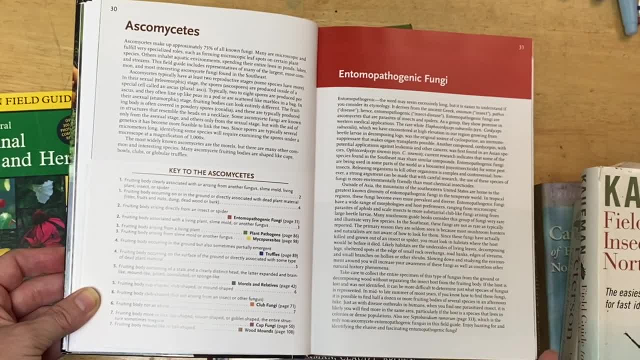 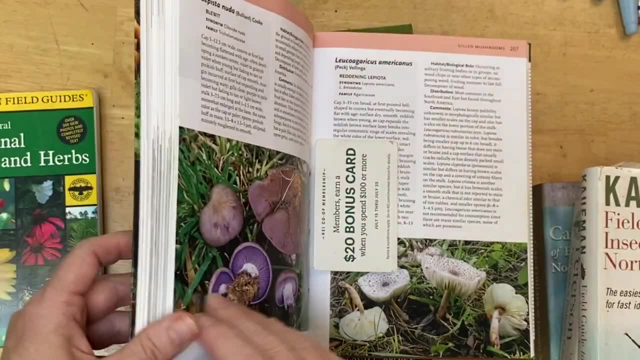 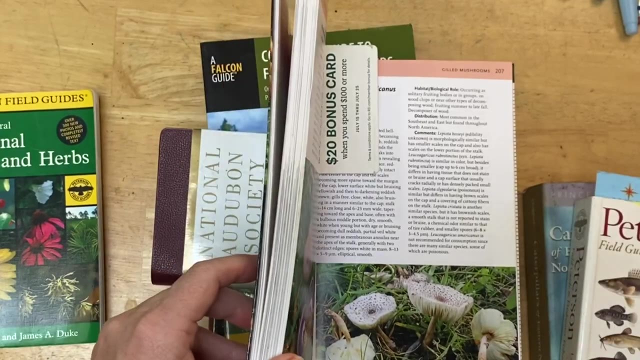 particularly if you're not a scientist. but as you get more of depth, they're more helpful in that, so this is one of my favorite ones. this has all kinds of identification and habitat, and i also really like- though i don't know if i have one here- 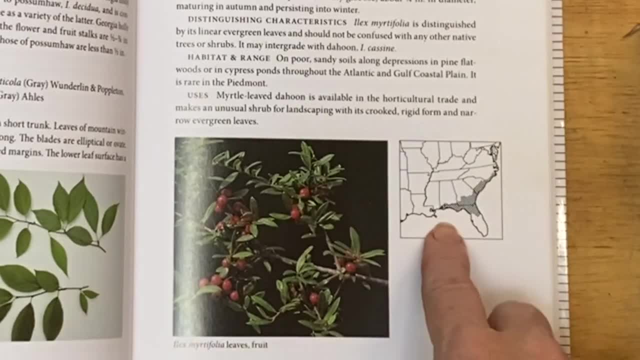 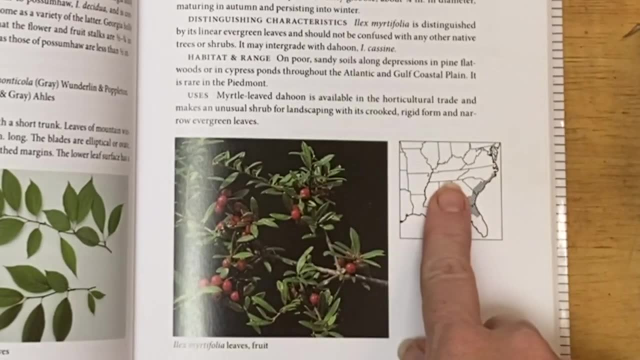 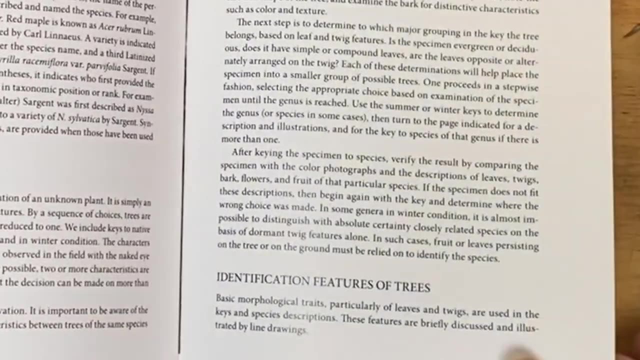 the range and distribution when guides have little maps of the range and distribution of that species. Sibley's bird book does, which is fabulous. i really like Sibley's bird books as well, so if you're looking for a bird book, that is a great book. this one is native trees to the southeast. 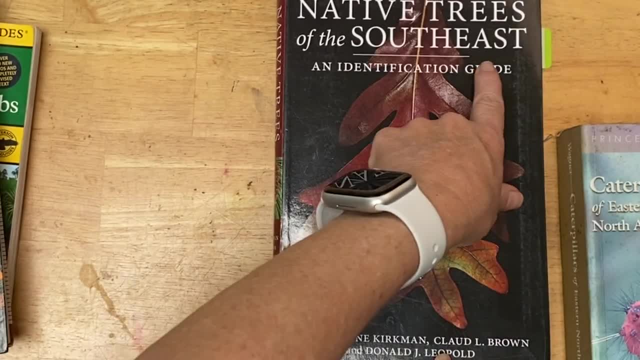 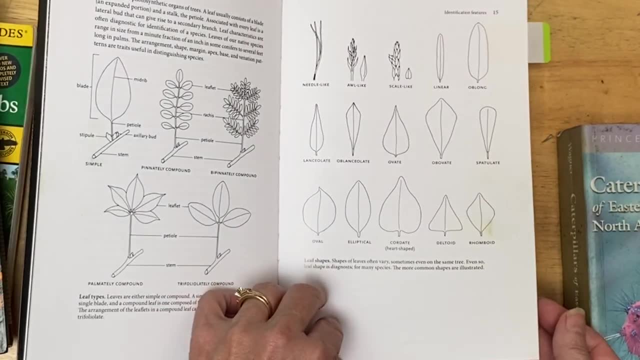 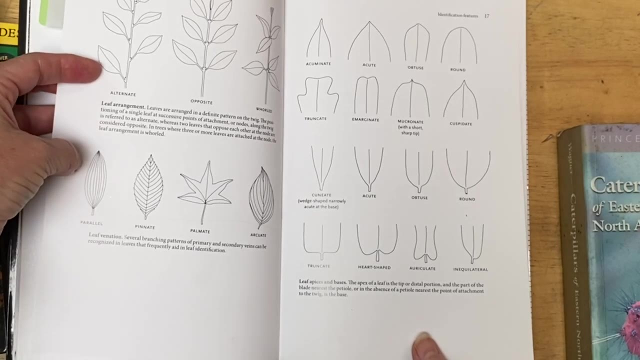 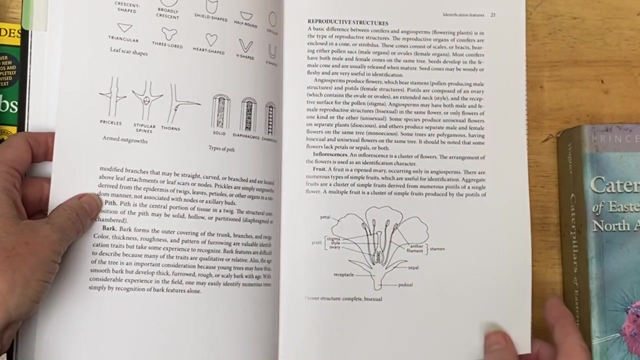 it is not quite as specific in Florida, but it definitely is specific in the region that i'm looking for and you can see here it has the different aspects of the leaves that you look for during identification, as well as the leaf arrangements, veins, shape and margins, and as well as twigs- the twigs- 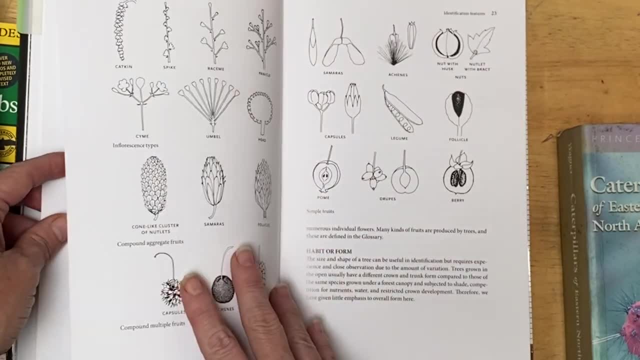 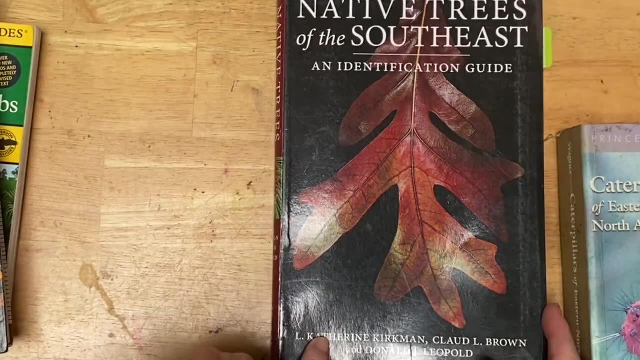 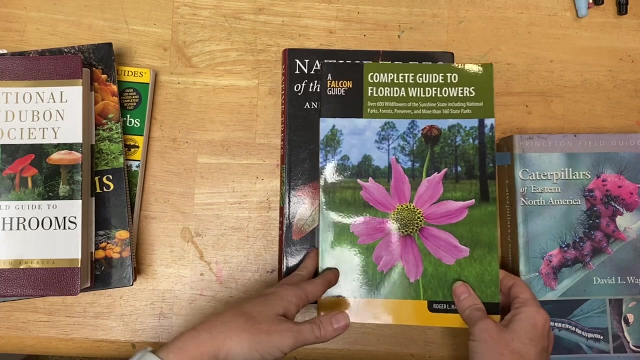 formation is also important in tree identification, and then the seeds and flowers, so i really like this guide as well. if you're in the southeastern United States, this is a fabulous guide. now i'm going to show you another guide that i think is going to work okay for us, but that i'm going to show. 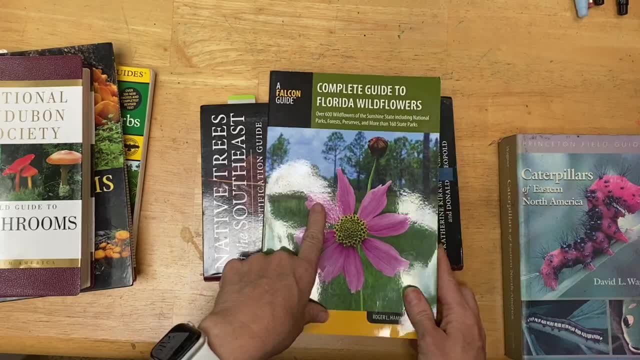 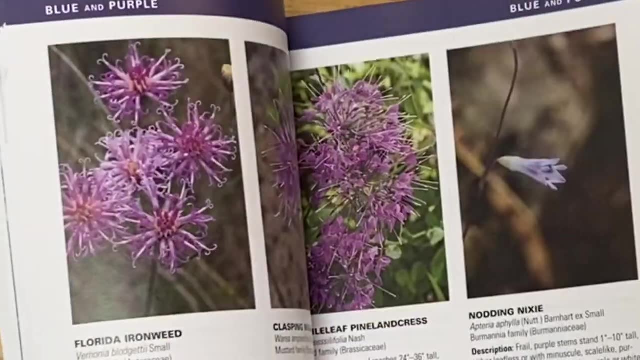 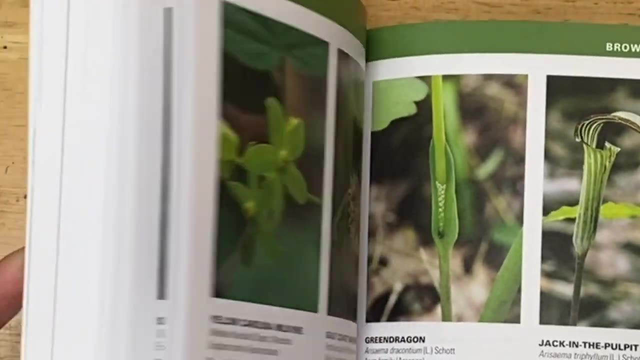 you I'm not a hundred percent happy with, and this is our wildflower guide. this is arranged by color, which I think is absolutely fabulous for a beginner, but one of the challenges that we're having is that we're learning these by family and they're not arranged by family and they're not. 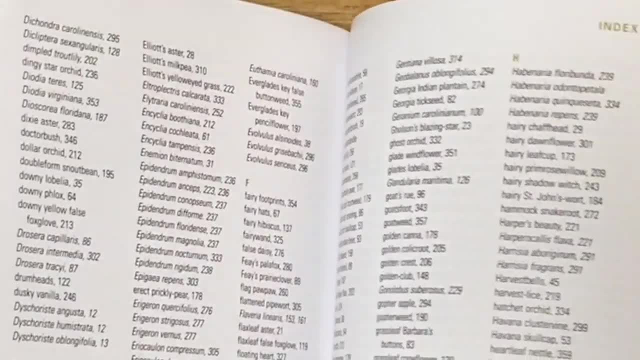 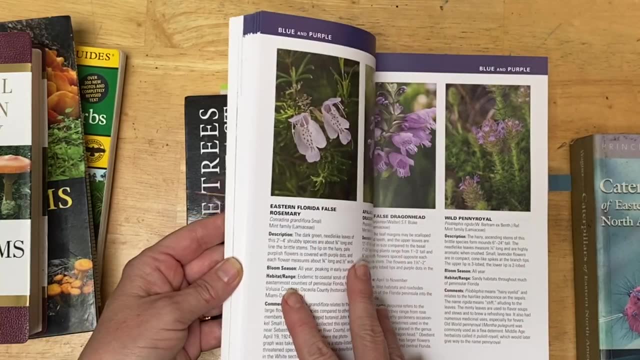 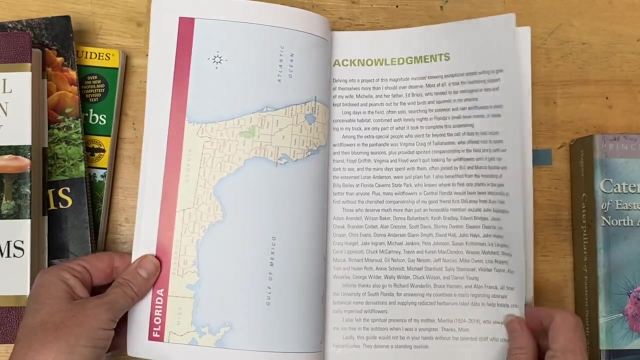 particularly good about having an index that indexes them by family, so that makes it a little challenging for us to use this if we don't know the color of the flower. in addition to that, you can see it's missing any map for distribution and the information in the beginning is okay. 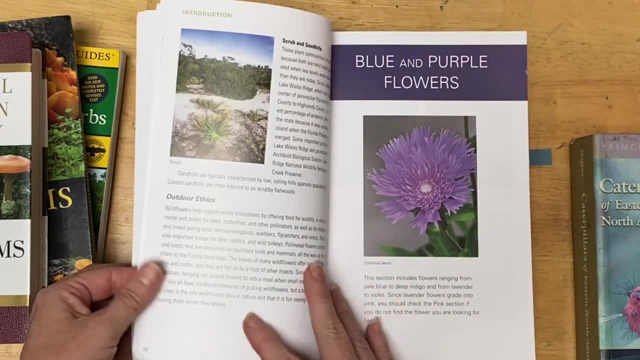 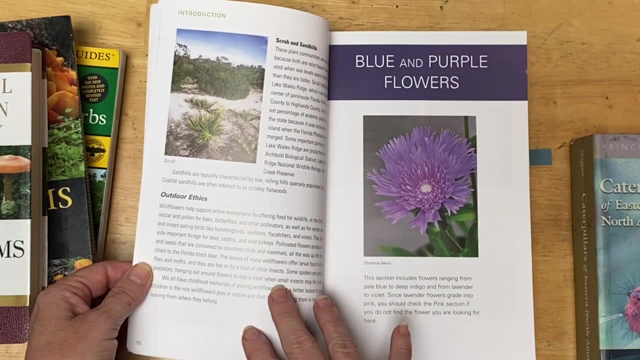 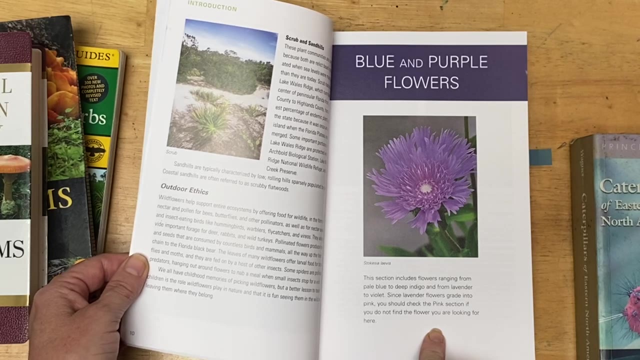 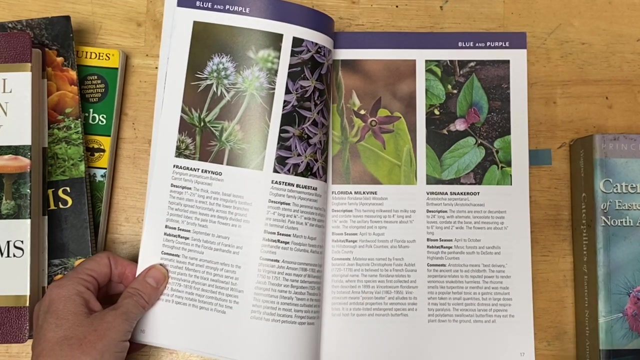 as far as ecosystems and where you might find flowers, but it is completely absent of the different field features, shapes, any drawings or guidance on what to look for you in identification other than the flower. it talks about them in the description of how to identify. it talks about leaf arrangements, margins etc. but it doesn't have. 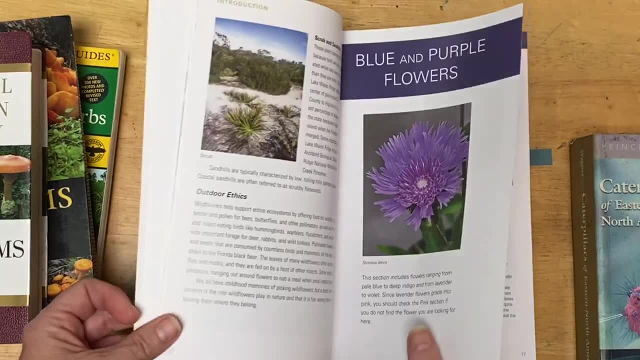 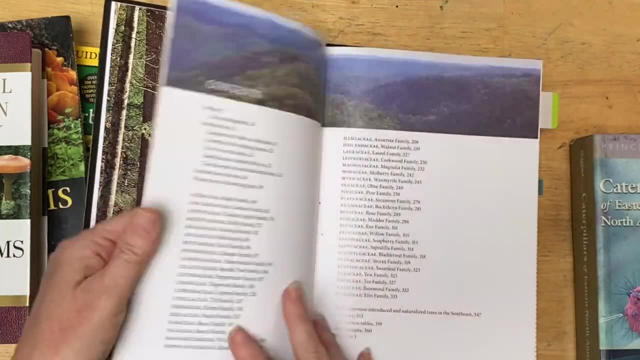 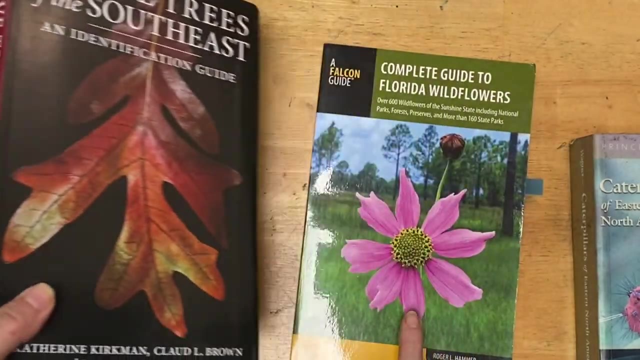 any drawings to show you what those are. so if you don't know, like I do, from this tree book the different information on margins, leaf arrangement, shapes, etc. then you're at a loss somewhat on identification for this book, which, yeah, and then I want to show you my very 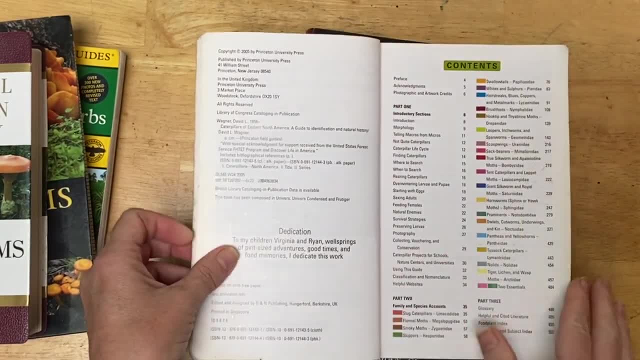 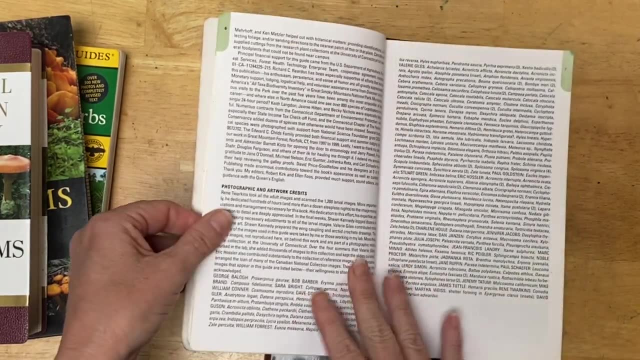 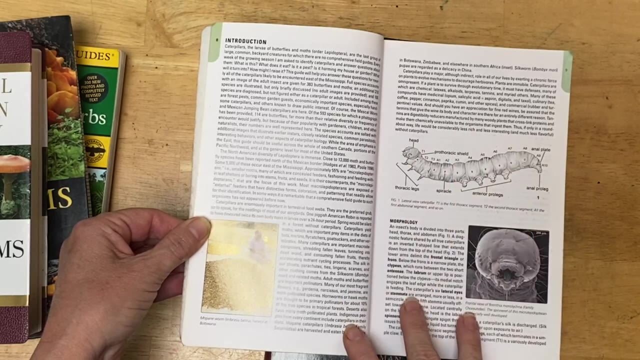 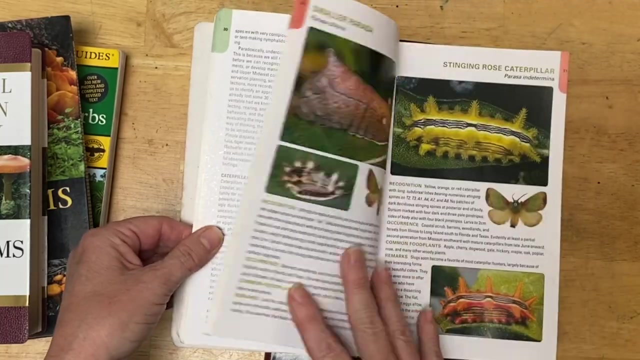 well-loved and dirty caterpillar book. and what I love about this? this one is of eastern North America, so it's not as specific as our other ones. but I love again the identification information and the life cycle information in this guide. so that's the kind of things that you're looking for: the identification and life cycle information. 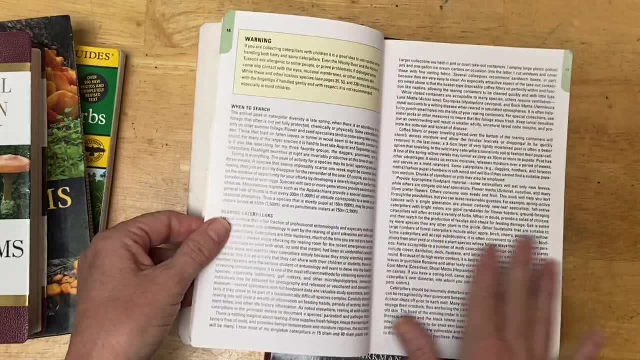 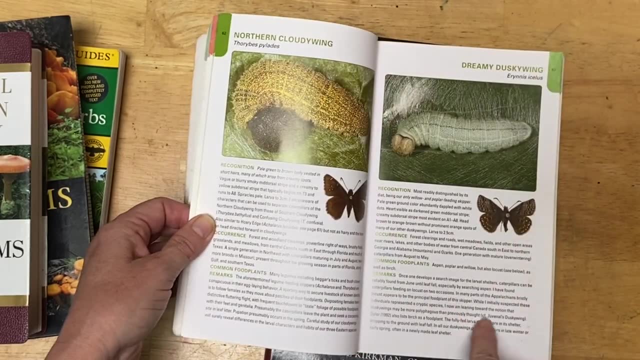 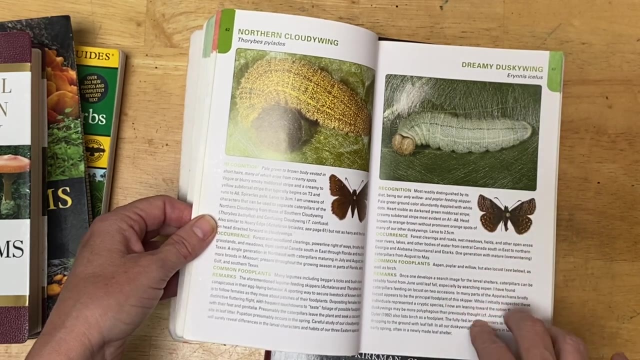 in the beginning, the habitat of your areas, the different ecosystems and micro ecosystems within your areas, and then, ideally, you want plenty of pictures, description, habitat range in there as well, and this doesn't have a lot of information about the soil, so I'm just going to show you a 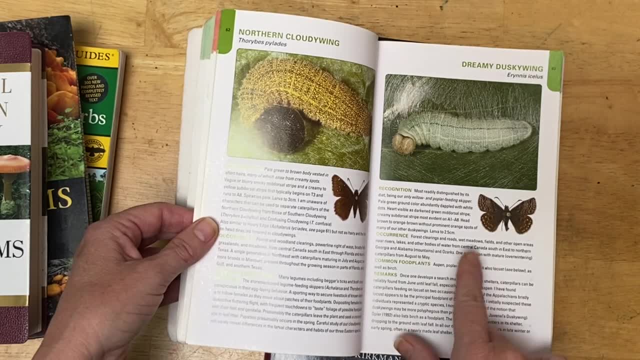 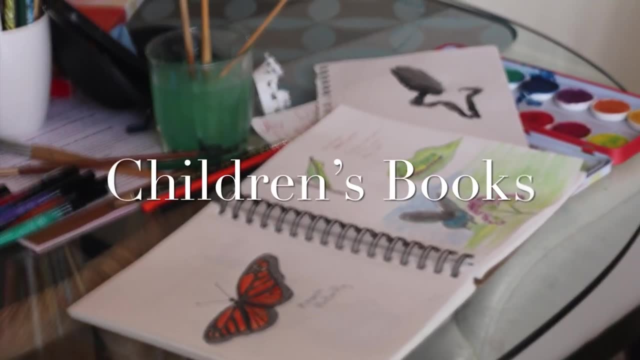 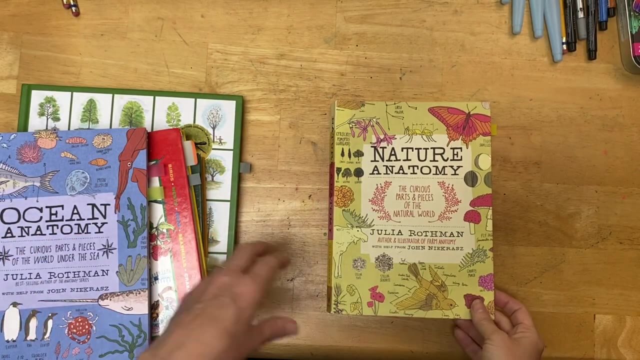 it does have it written where the range is, but it doesn't have the little maps, and I find the maps to be highly useful. Now I want to go through some books for children. I'm just going to spend a little bit of time on this because there can be so many, So one of my favorites is Nature Anatomy. 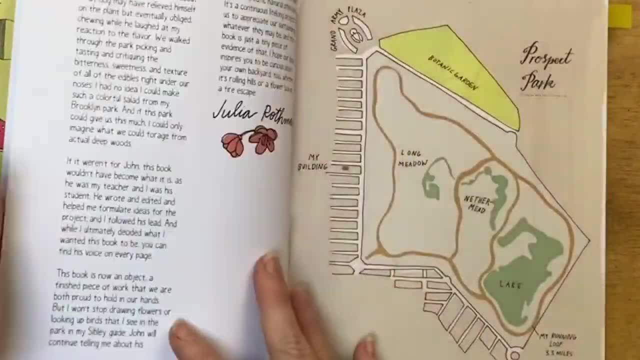 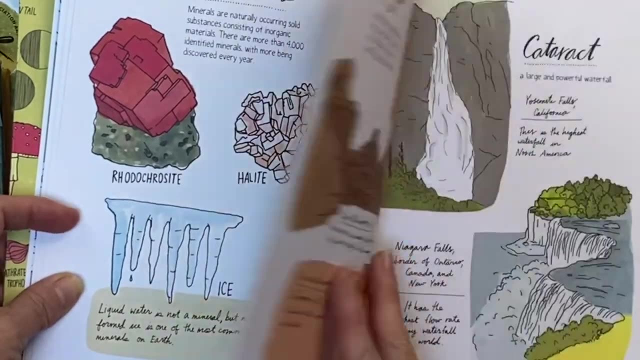 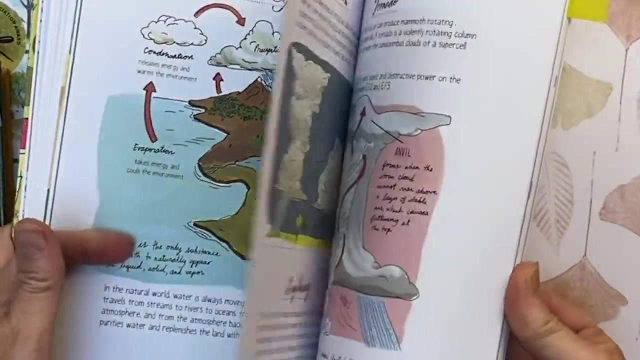 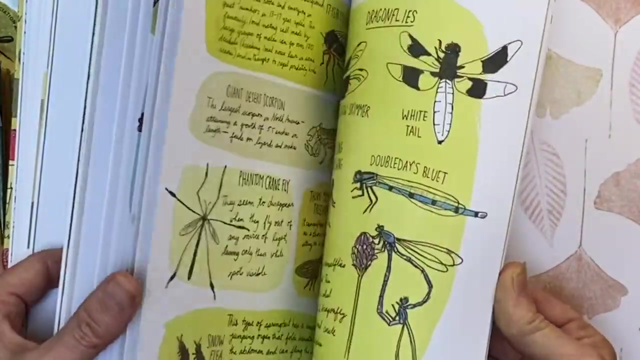 and I like this one because it has so many diagrams and illustrations of different natural concepts and it ranges from geology to habitat, water cycle, all the way to life cycle of plants, insects, birds and so see. it has some of the shapes. It doesn't have the detail that the guide 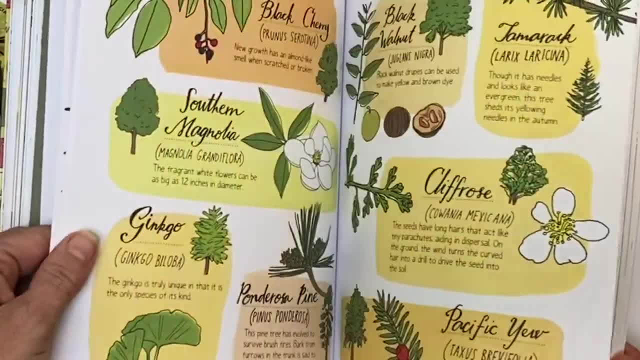 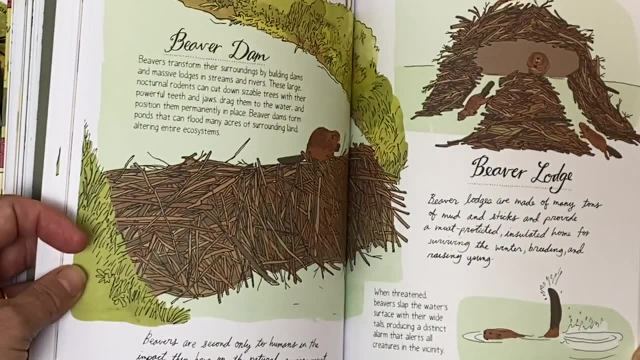 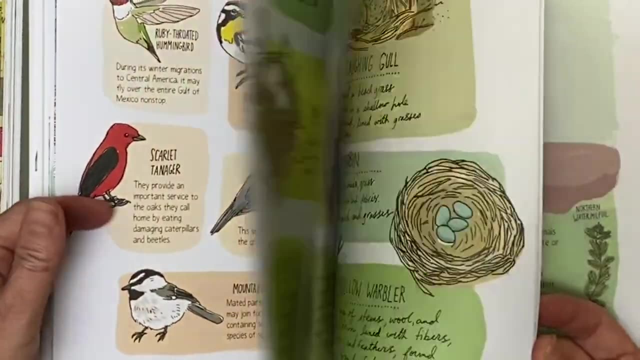 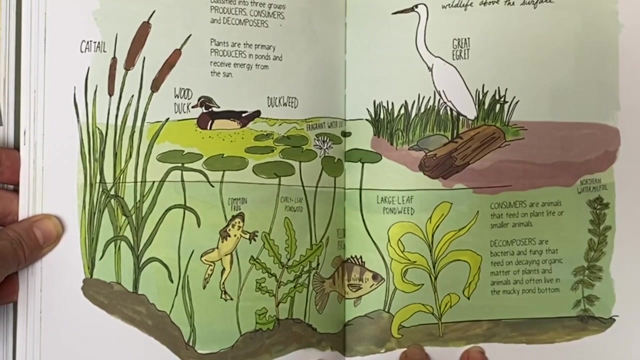 is going to give you, but it's got a fair amount of detail for a children's book with different pictures. It also gives an idea of kind of what a child's nature journal might look like. Here is the ecosystem of a pond, which is really nice, so this would be a very nice diagram to have. 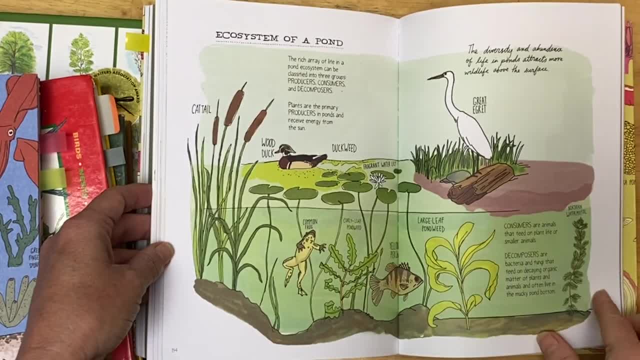 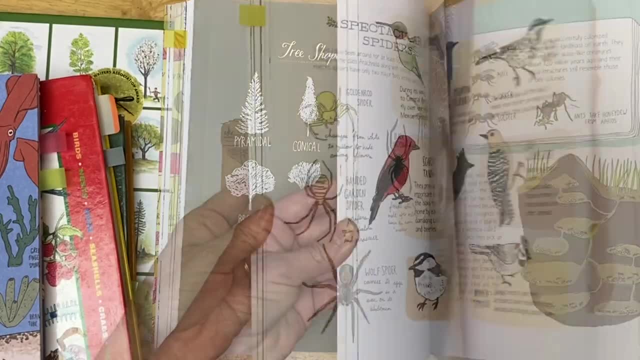 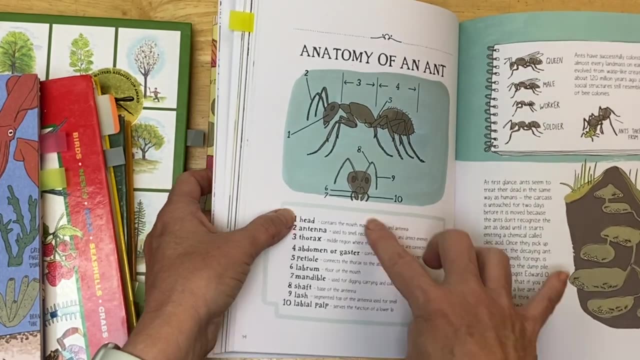 in the nature journal that goes over the different aspects, and I also want to find and show you some of my favorite pictures. So I'm going to go ahead and show you some of my favorite pictures And here's an example of anatomy picture. This is anatomy of the ant and it goes through and has 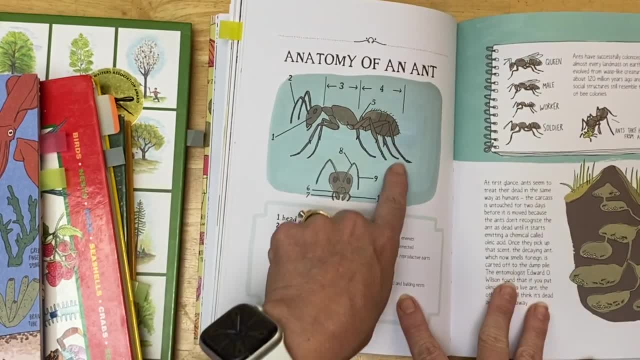 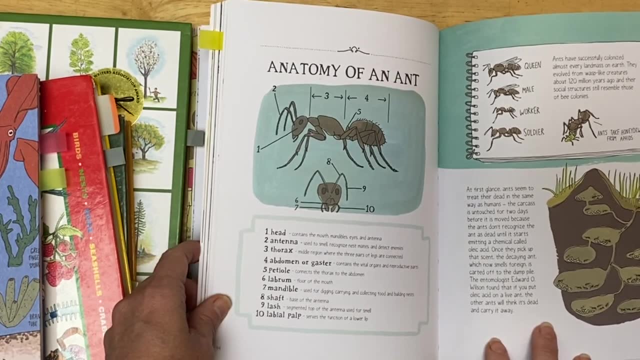 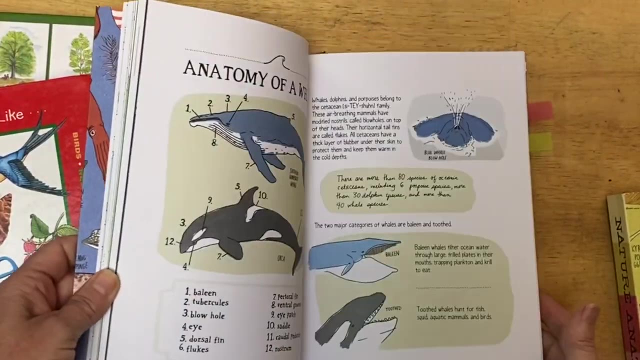 different parts and it is labeled. I wouldn't do the numbers here, but I would actually write the words in. but these: this is also a great example of an entry into a nature journal. They also have one on oceans which you know I had to get, and I love this one just as much as the. other. I'm going to go ahead and show you some of my favorite pictures. So I'm going to go ahead and go ahead and show you some of my favorite pictures. So I'm going to go ahead and show you some of my favorite pictures. 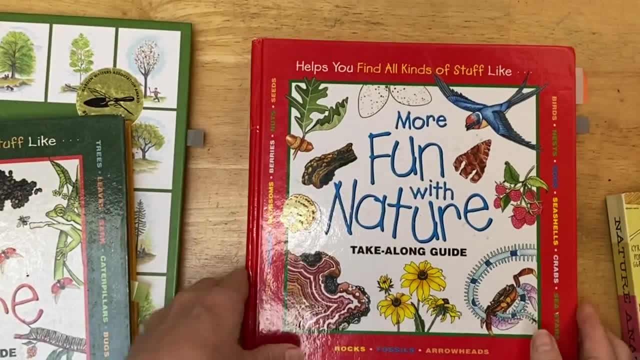 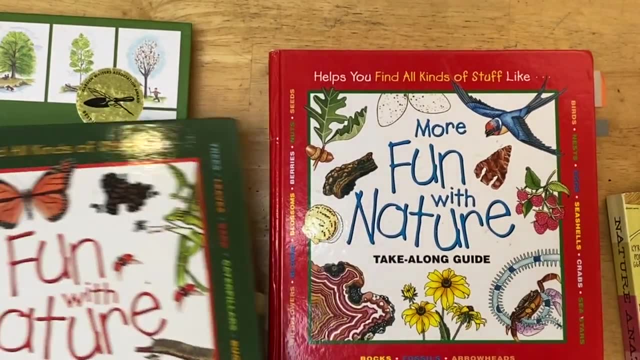 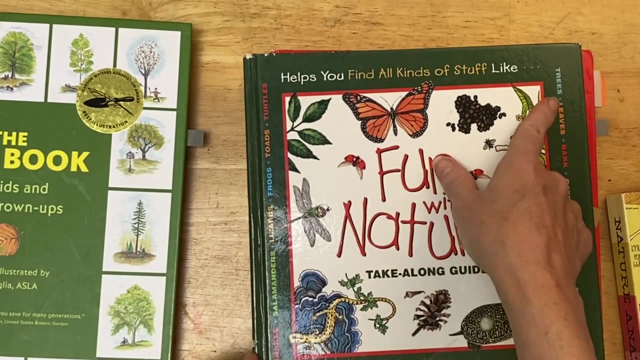 The next guys that I want to talk about. these are for younger children in elementary. are these fun with nature guides? They have a couple different ones. I have two, I'm not sure how many they have- and they are divided by different organisms. so this: 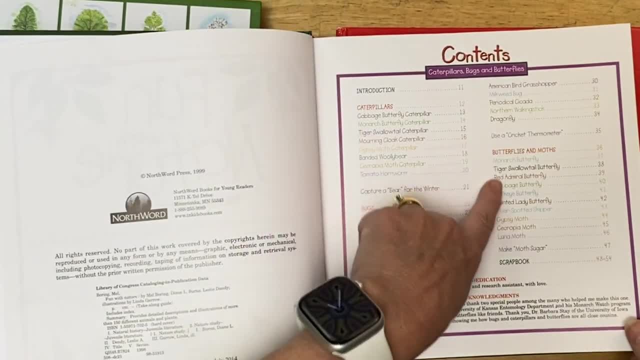 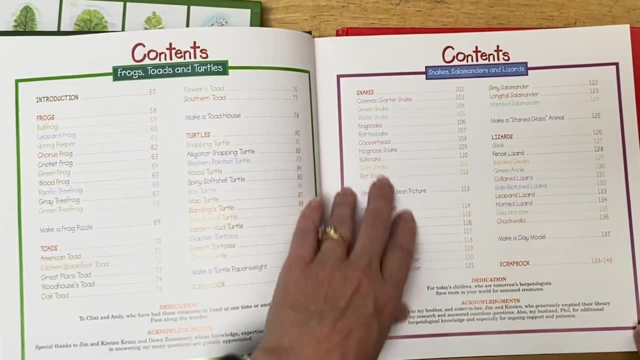 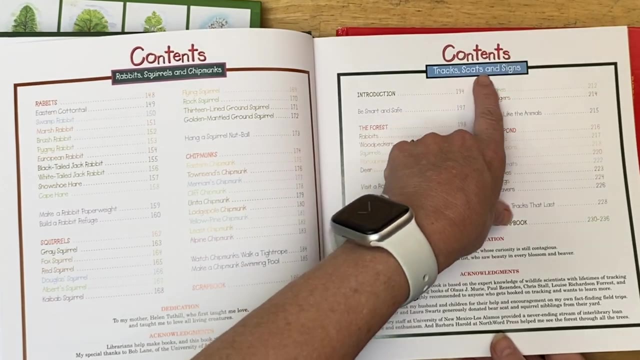 one has caterpillars, bugs, butterflies and moths, frogs and toads, turtles, and then snakes, salamanders, lizards, rabbits, squirrels, chipmunks, tracks, scats and signs. That's always fun And leaves trees and bark. 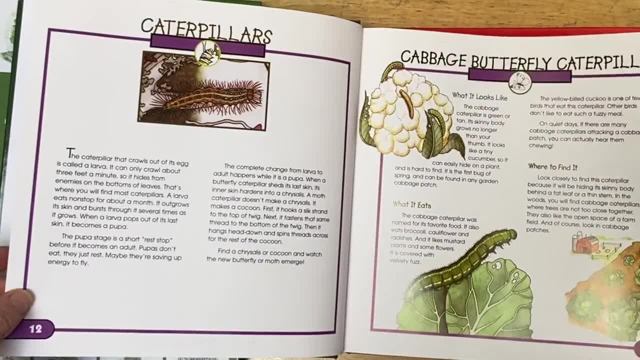 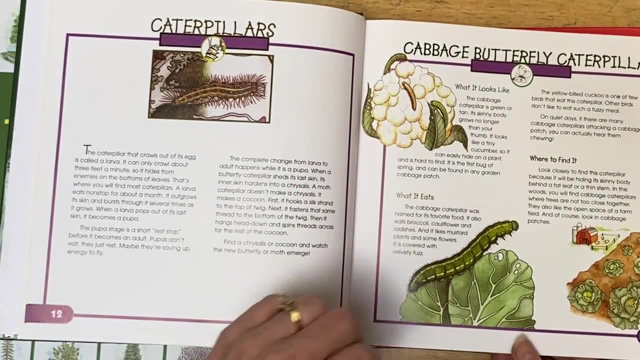 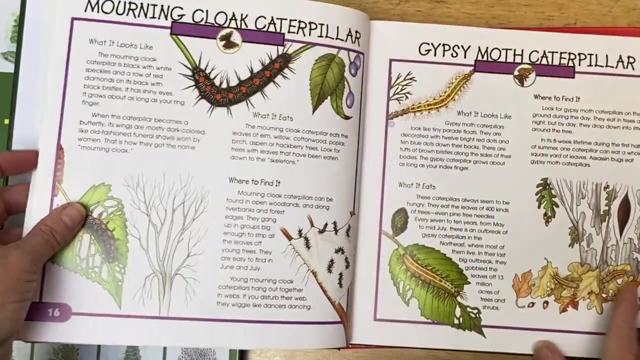 They do a little information at the beginning and they give a little information. It's basic but general information of what you might find. They don't have too many species listed, but that's okay. These tend to be pretty general, so it's more than likely you will have. 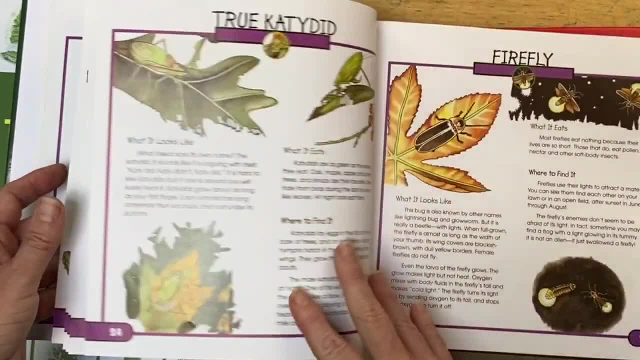 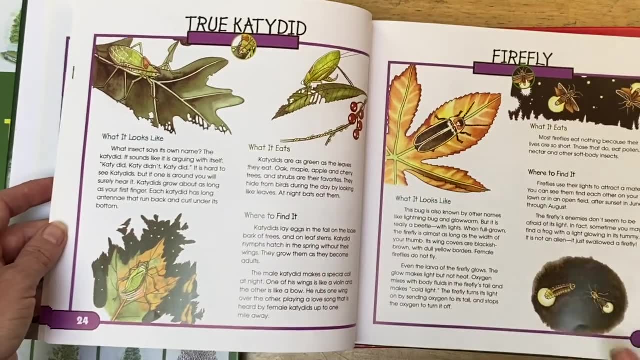 something similar in your area, because they do tend to have a wide range- Not all of them, Like I know, fireflies aren't throughout all of the United States, but on the East Coast they do tend to have a wide range, Not all of them. Like I know, fireflies aren't. 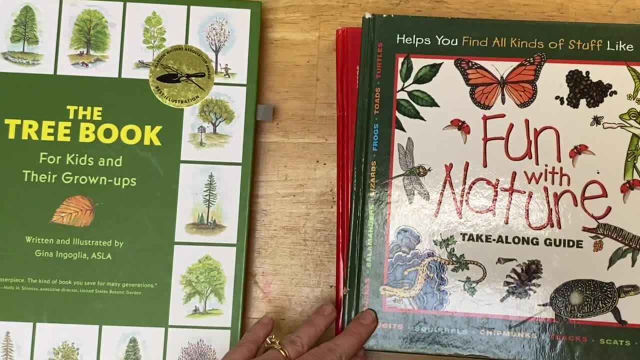 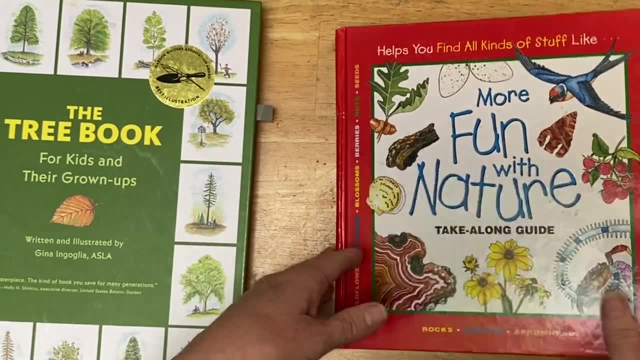 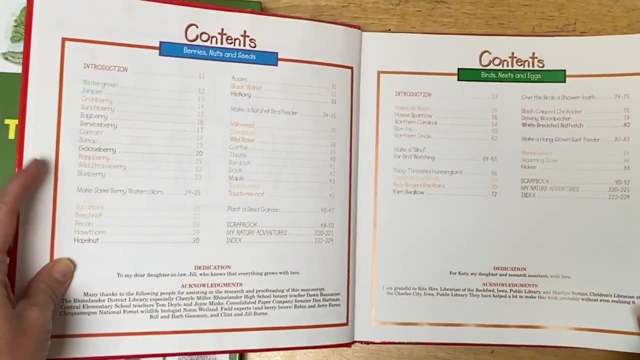 throughout all of the United States, but on the East Coast they do tend to have a wide range, And I want to say that this is more the United States. And then they also have another one, And this one goes over birds nests and eggs, berries, nuts and seeds. 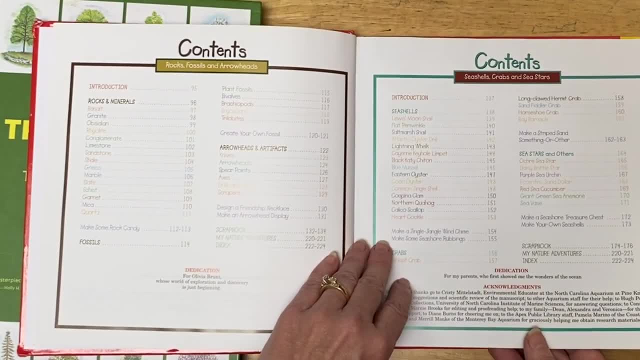 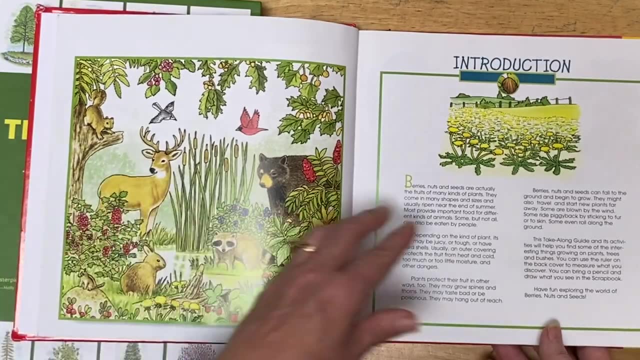 fossils, rocks, arrowheads, seashells, crabs and sea stars, as well as wildflowers, blooms and blossoms, And it's the same kind of thing. It's pretty basic, but it has general information at the beginning and more specific information. 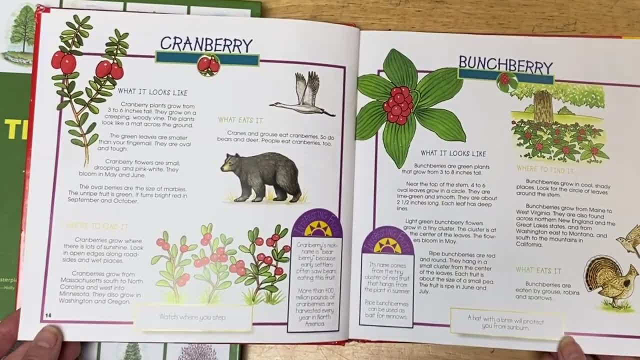 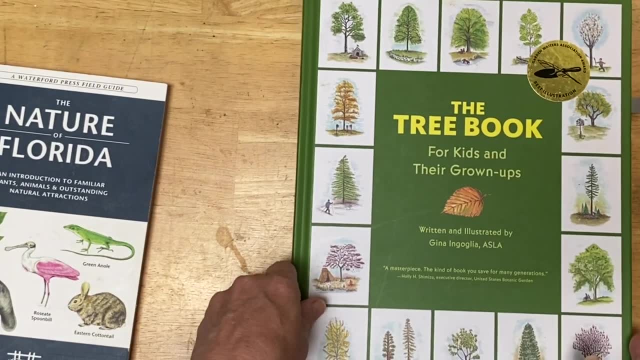 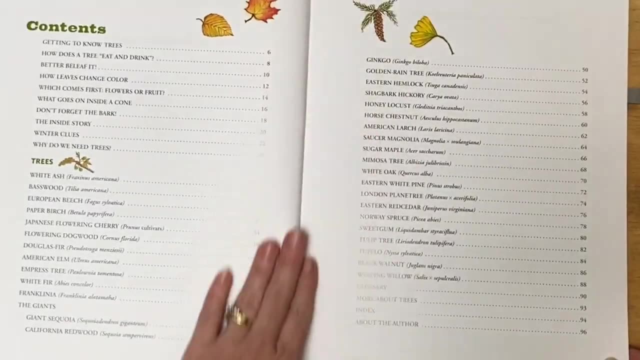 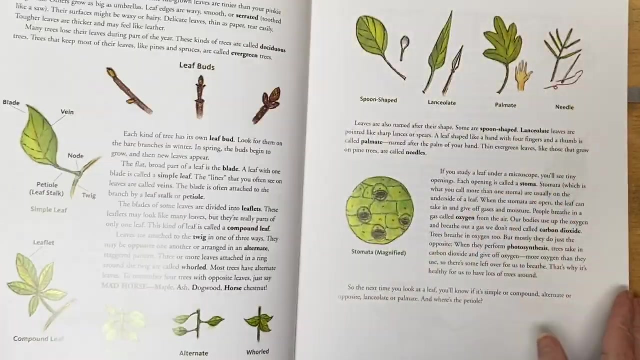 as you go along, But it's still pretty general. It's not going to be what a local guide would be. And then I also love the tree book. This one is, of course, about trees, but I love it for the information that it gives in the beginning about trees in general. 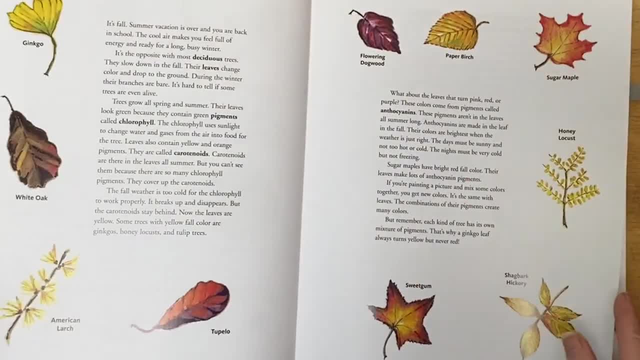 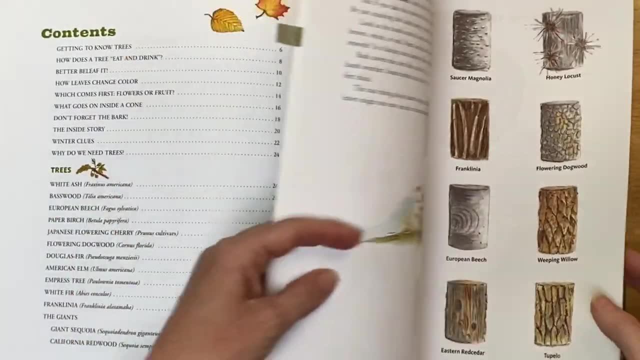 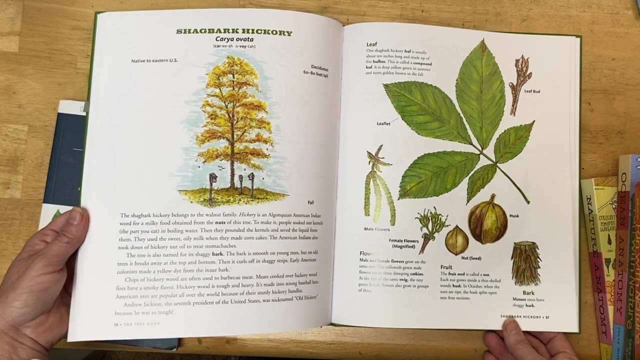 and about tree identification. It has just some fabulous information on that, And it does have a few tree guides in the back. But you know, being a children's book, it is going to be limited on what trees it has, And so 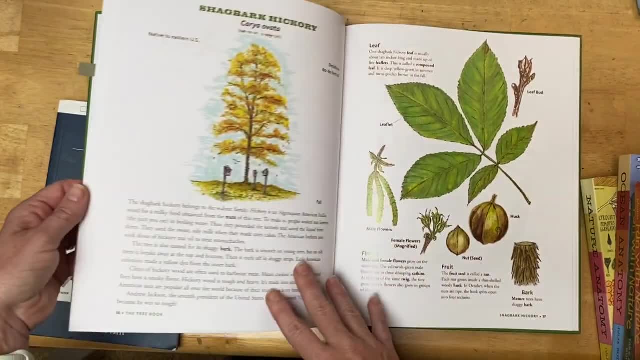 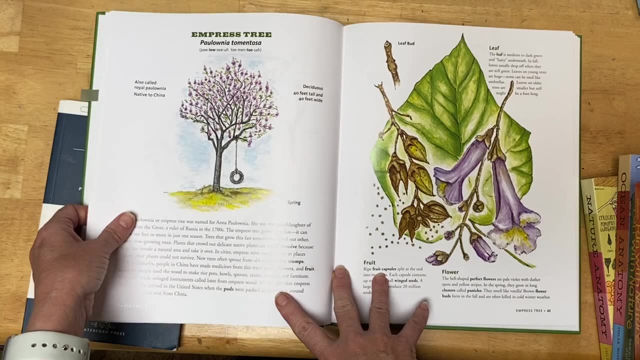 it does tell you where the trees are native to, but it's not going to tell you where the trees are native to, And I'm really happy with this because I think it's great. I think it's been a really nice chance to be able to share that kind of information, and some of people love that. 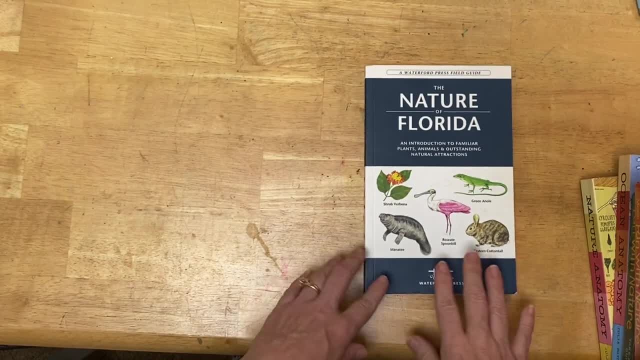 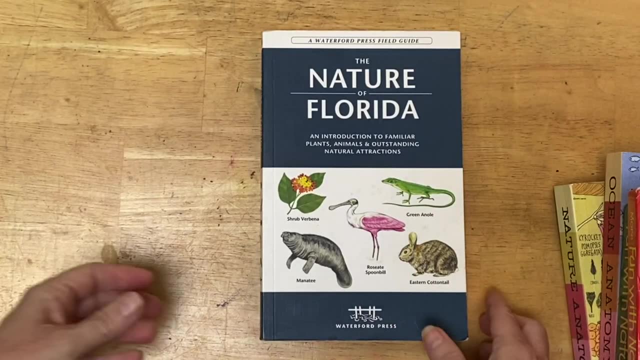 Speaking of local guides, there are a very few Clark County book contenders here, And I love that there's a book called one that talks about research or research guides, And also the magazine that I sometimes read called edesmtersmongacocom. 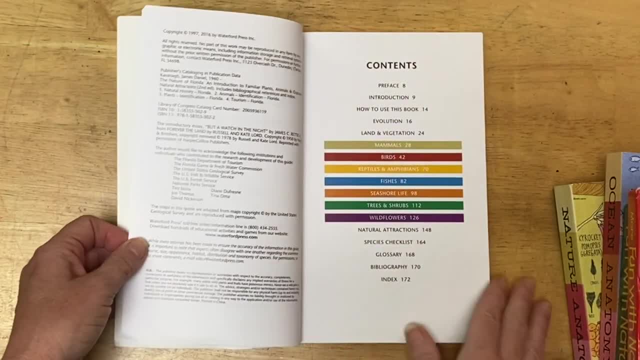 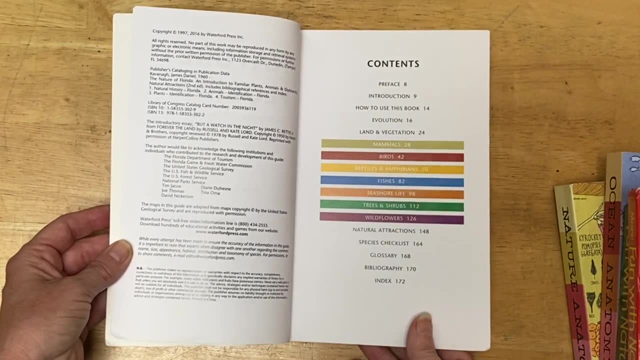 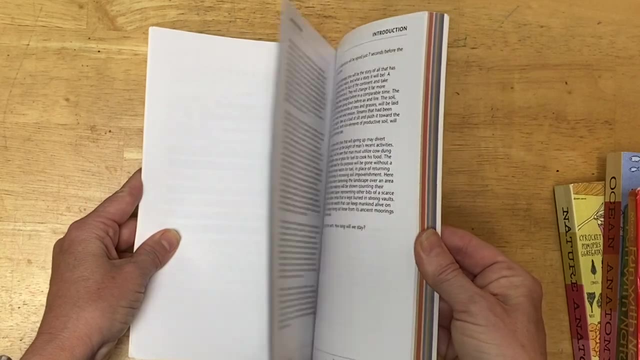 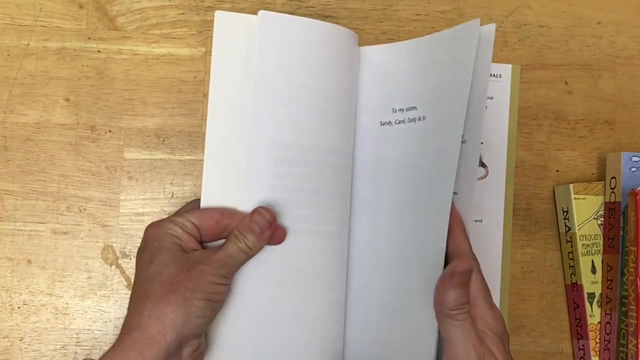 well, but it's a really good gift resource to have because it has such a wide variety of different animals, species within your ecosystem. this one is for florida. i'm sure that they have other states and it goes through. let me see if i can find the table of contents. 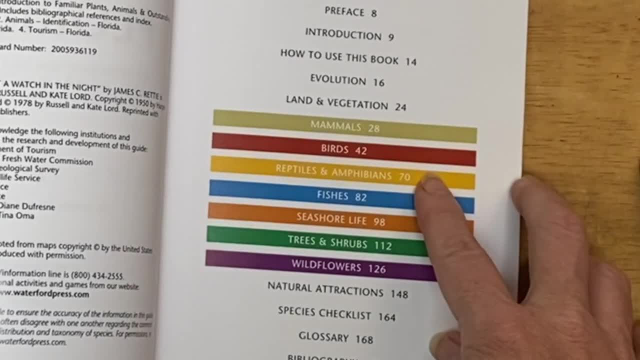 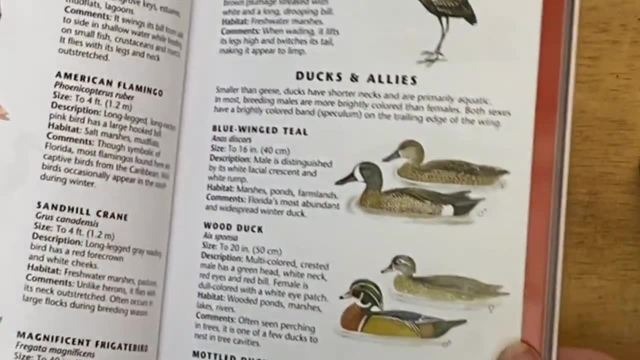 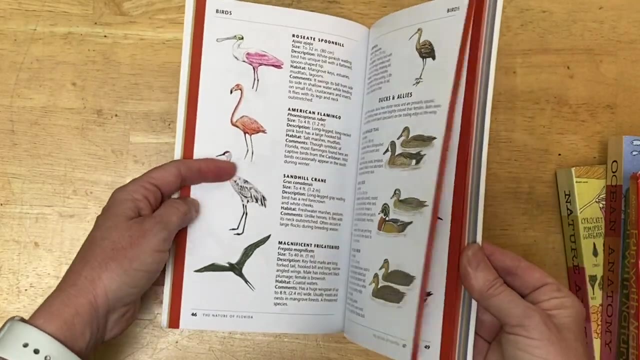 it goes through mammals, birds, reptiles and amphibians, fishes, shore life, trees, and shrubs and wildflowers, and what's great about this book is that we have found it to be fairly useful for our area, like we are able to see a good number of these, so they're using a wider range for these. 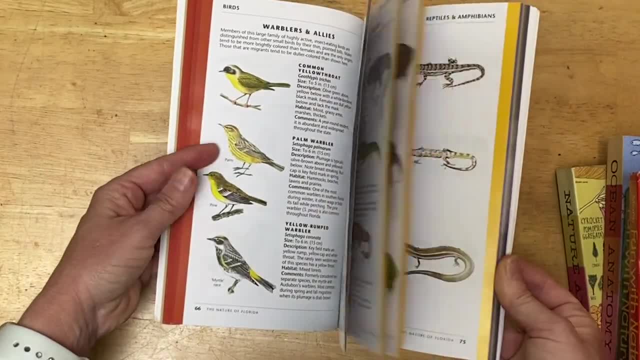 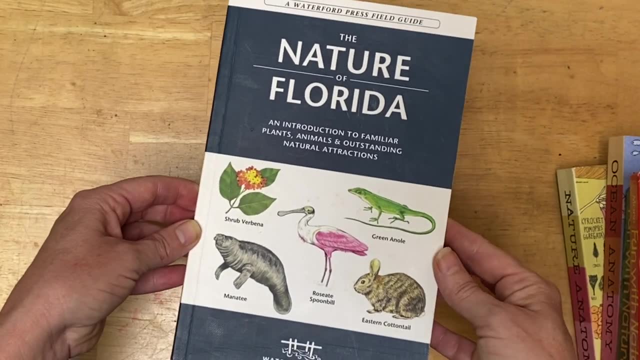 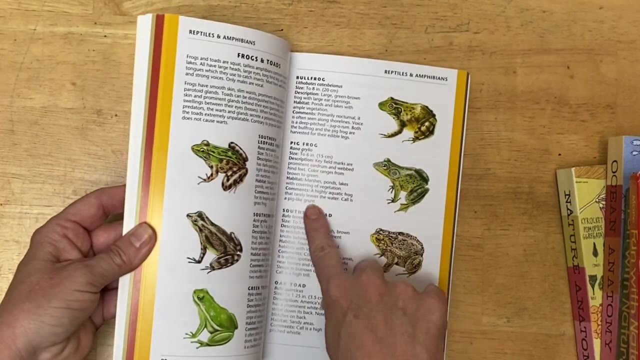 species, which is really nice, and this is small enough that it's perfect to take with you, you, you, you, and it sparks curiosity and my children were always really excited to find something that was in the book and it gives you a little bit of a description of each one again, because this is 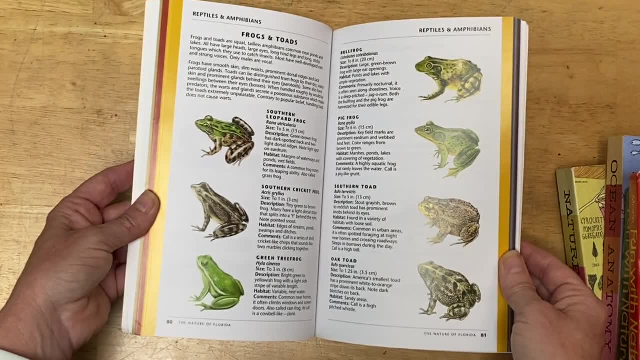 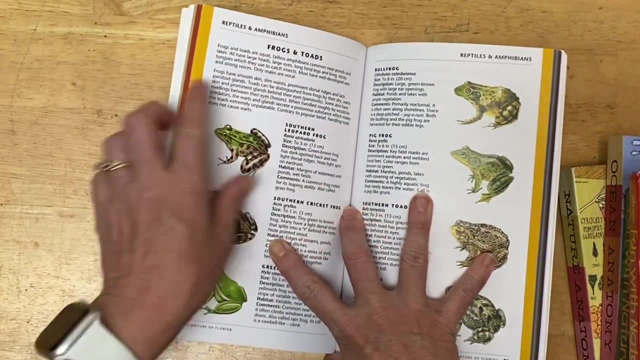 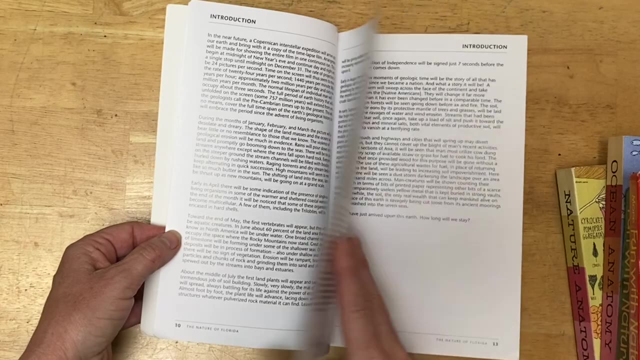 a small book. it doesn't have very specific information, but it does have information in the beginning, like this goes over frogs and toads- and at the very beginning of the book. that i think is really useful and worth having, especially when you're first starting out, because 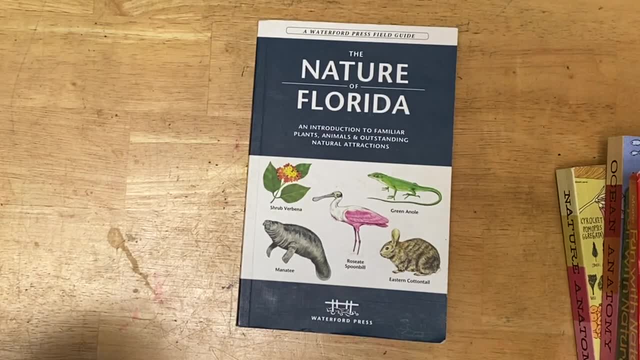 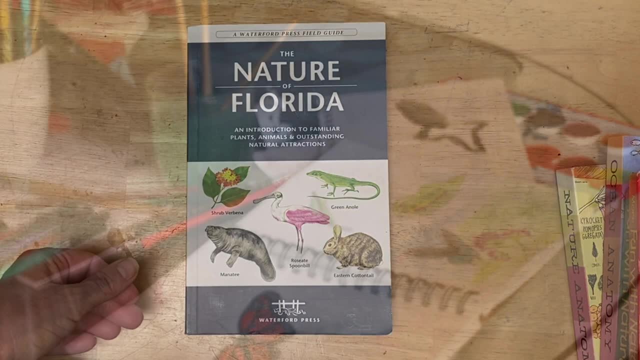 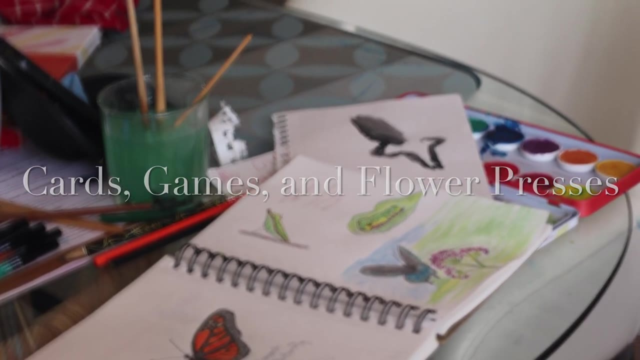 i've been schooling for 15 years, so we've accumulated books and guides and supplies, but if you're just starting out, this kind of guide is perfect. i'm also going to show you some games cards and various things that we have. their helpful edition for nature. 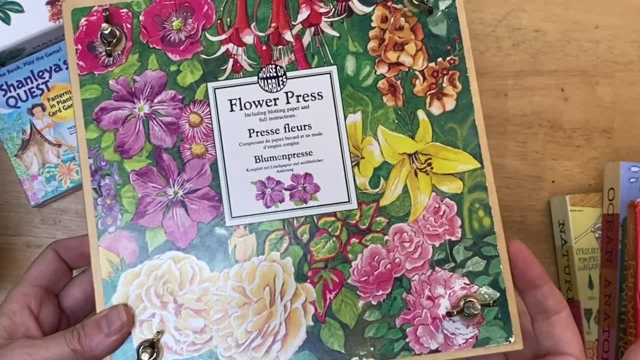 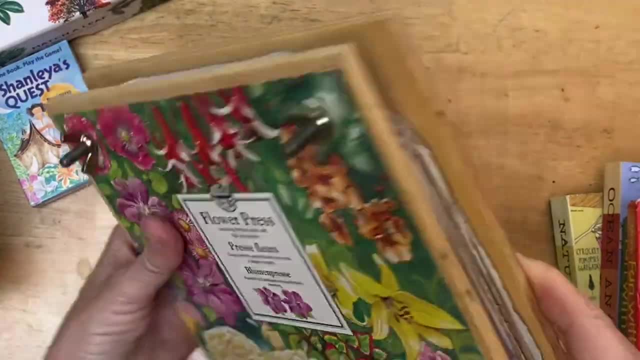 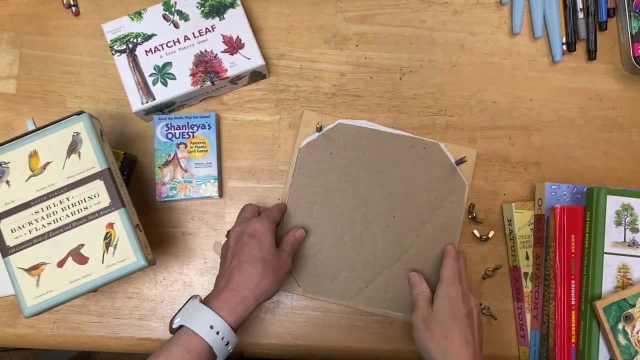 one is a flower press. now, this flower press was purchased for us as a gift from a thrift store, but really you don't need much. you can see this is two boards. i'll open it up for you. okay, here we are. you can see, there are pieces of cardboard. 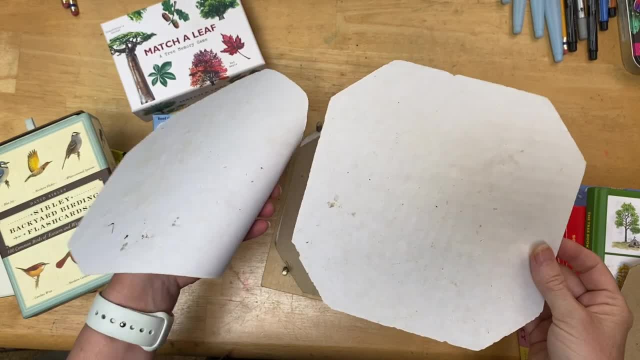 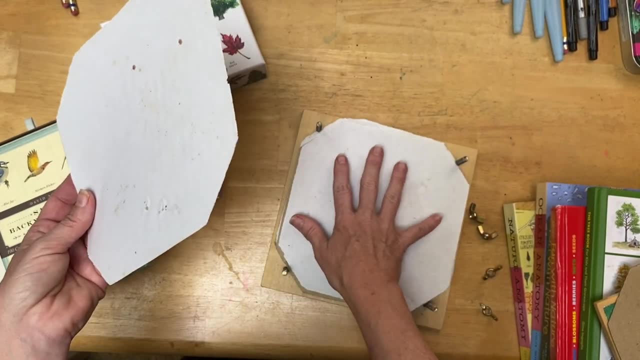 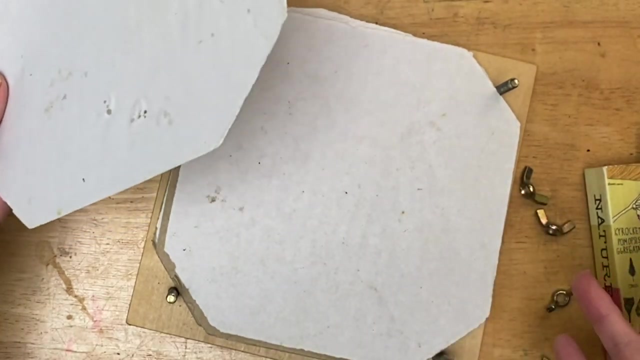 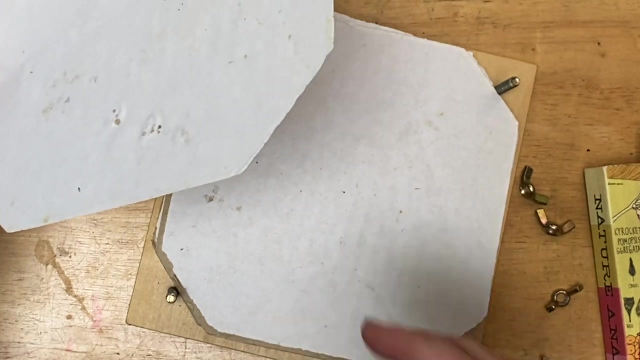 and in between are two layers of blotting paper. ours have been well used and loved, so you can see that we can see that a lot, and that one has a little smaller flower at the bottom on one side of this one. so it's one piece of paper, and then of course we have a two-by-ugly. 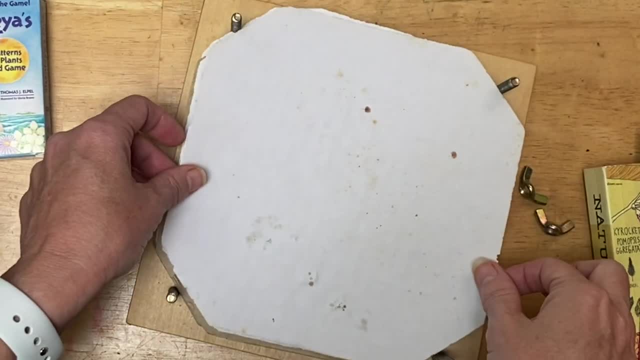 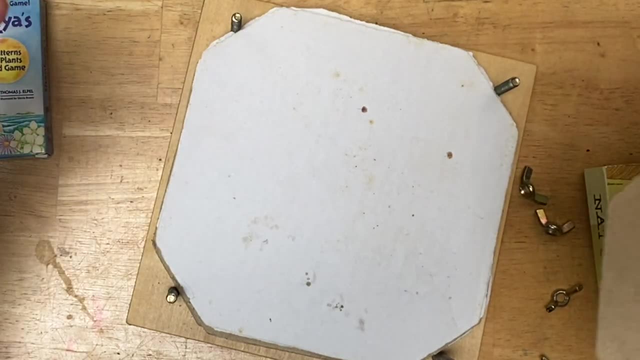 flower we have here and we have a little flower in the center here and here too. so it's a little bit more complex to see the difference. i'm going to see how those are placed on the flower press: temperamental, they're frail and so they will tear, and then you just construct this back together. 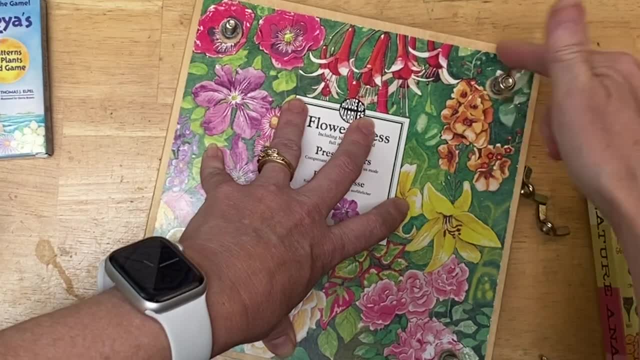 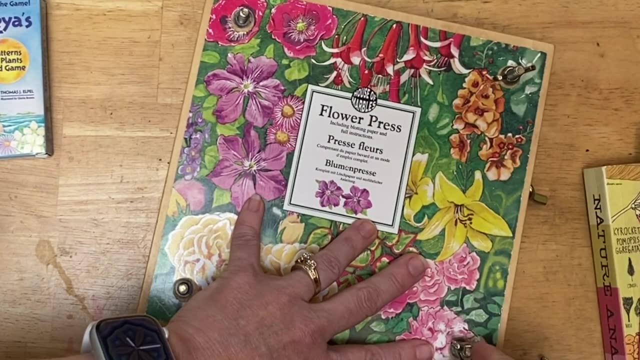 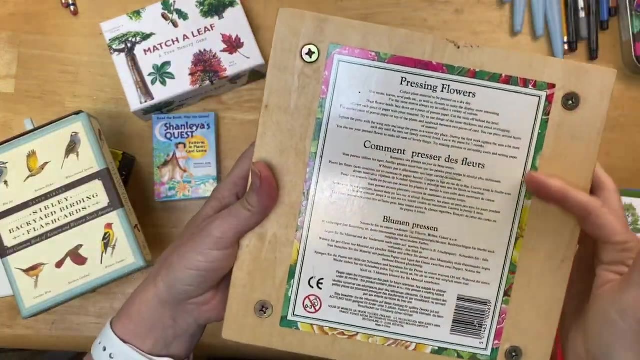 place the. i think these are called ice cream wing nuts- wing nuts, i think- and then you tighten them and then go back a day or two later and continue to tighten. it's fairly simple with instructions, and i think most of them have instructions on the back or it'll be easy to look up the. 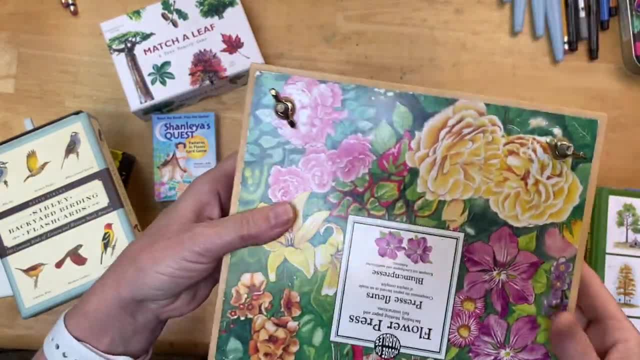 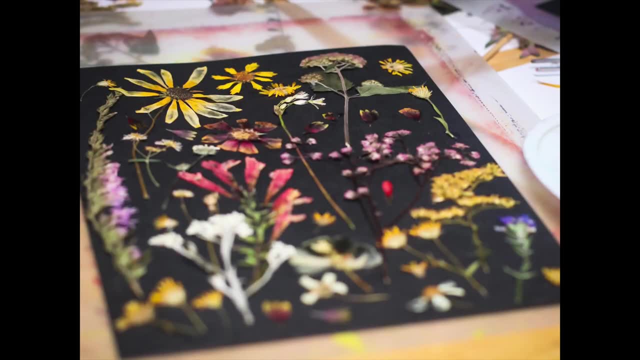 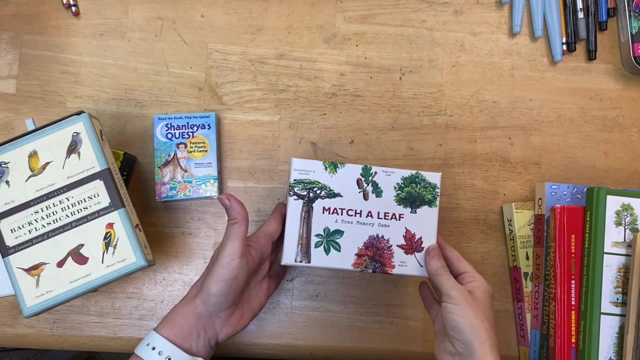 instructions, but you just want to leave it there a period of time so that all the moisture is absorbed and it leaves you a dry flower. i will also show you a recent project that we did with some of these dried flowers. this game is matcha leaf and it has trees throughout the world. 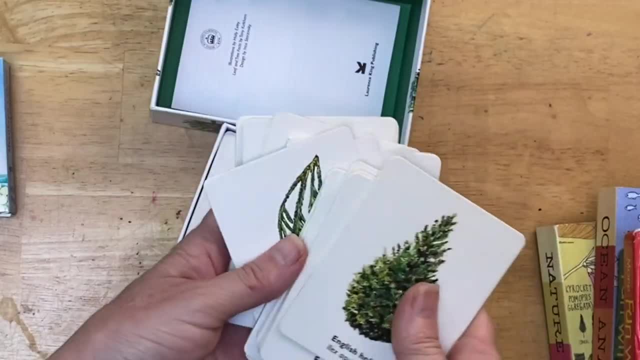 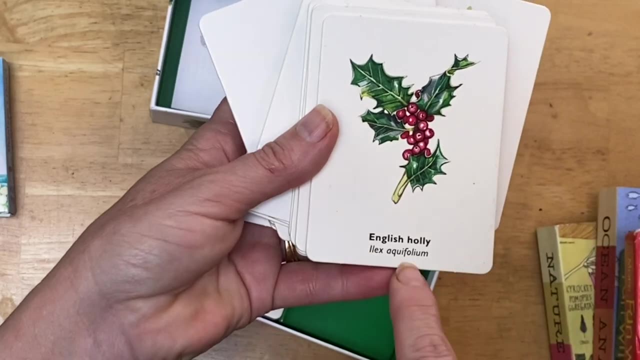 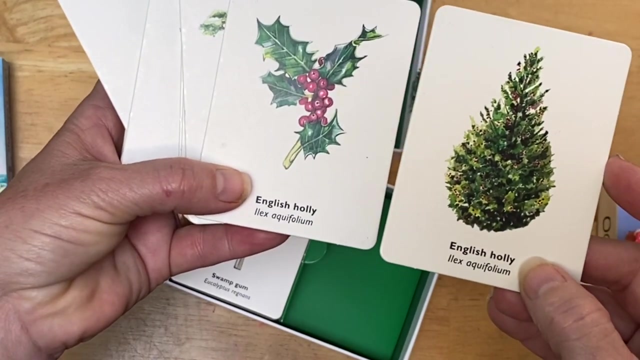 this pairs well with the tree guide. it will have the tree shape on one card and then the leaf of that on the other. it has the common name and the latin name, which is nice, but it doesn't really exhibit a lot of memory recall. it's great for familiarity, but if you're 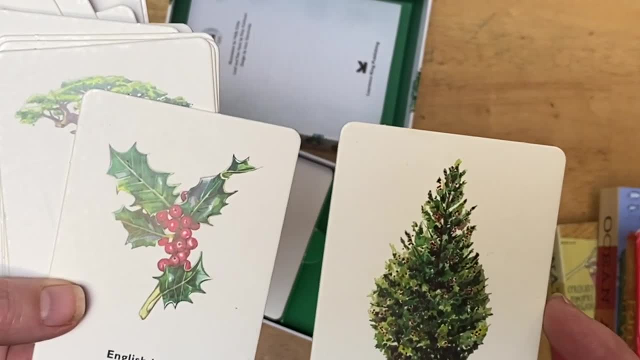 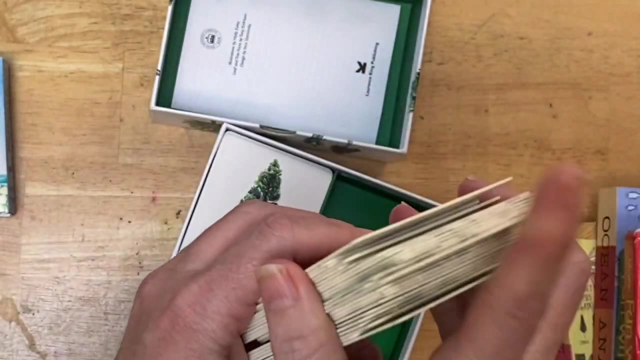 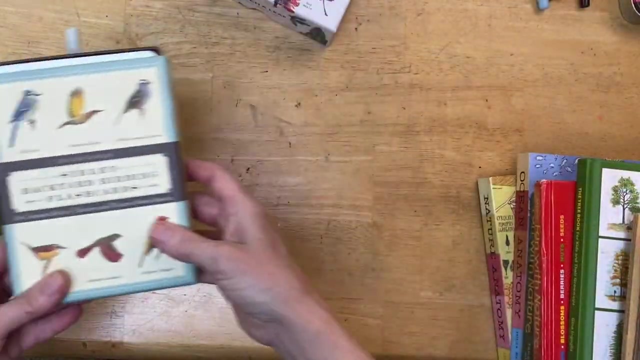 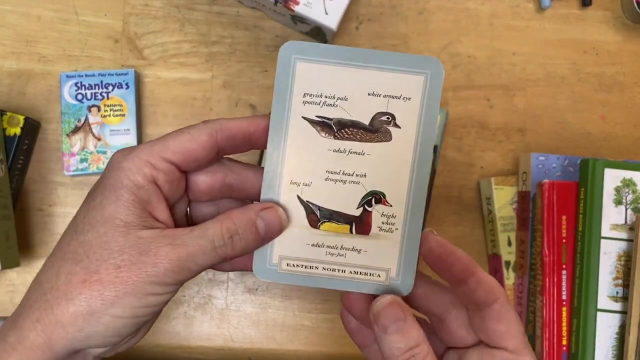 looking for retention. these aren't fabulous for that kind of material, but they have served really well for opening games and connection time before we start school, so i really like this game. sibley's cards are based on their book and they are fabulous. i have two sets of sibley's cards. 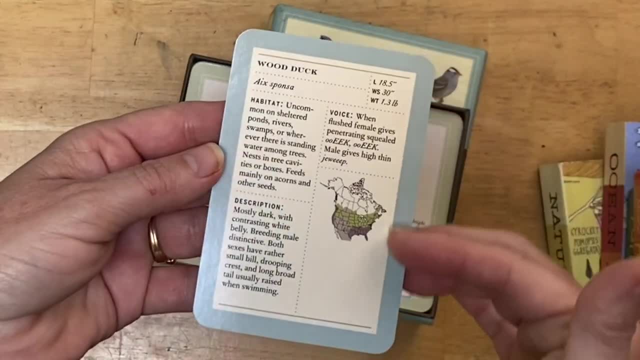 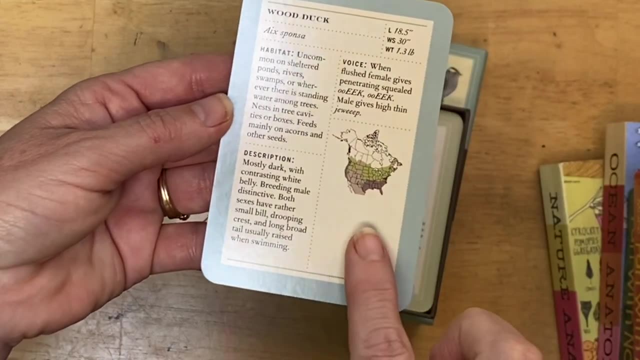 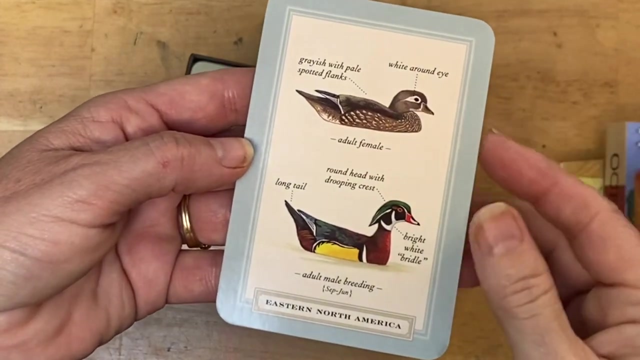 this one is for birds. you can see on this side. it gives the name with a habitat description, voice and the range. i love this range. this is what i love about sibley's: it has fabulous information. it also has very detailed and helpful information on field marks for identification. field marks are 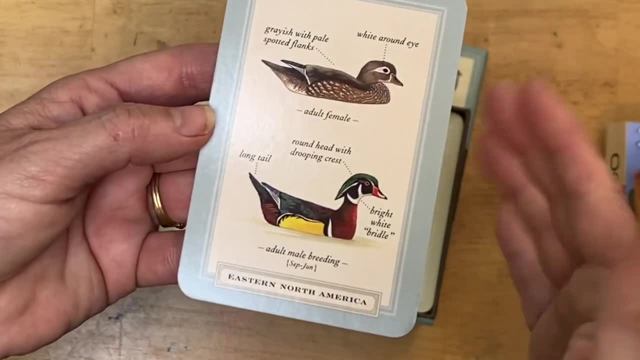 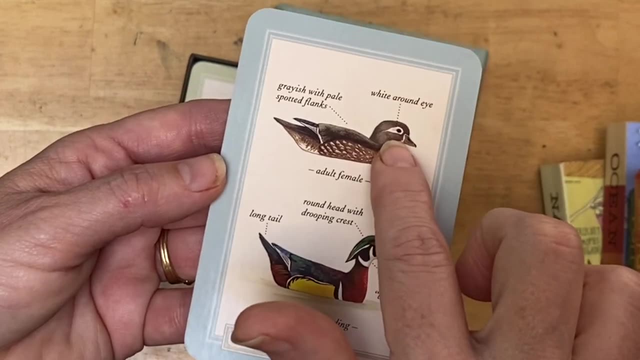 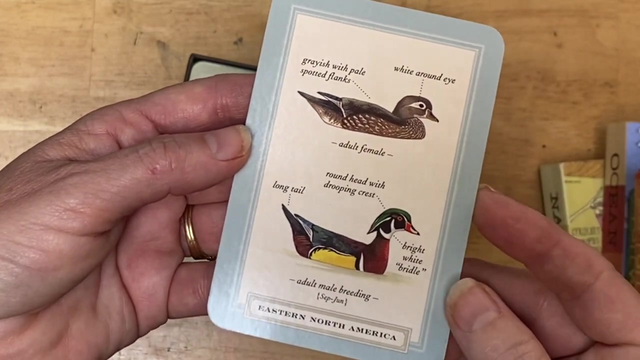 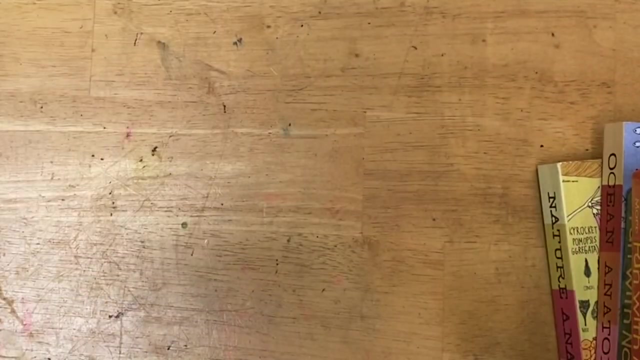 just different aspects of the species that really separate them from the other species. for instance, this one on the female talks about how there's white around this mark and how the back is grayish, and then, of course, it talks about all the male's colors in addition to the bird. we also have sibley's tree books, which are 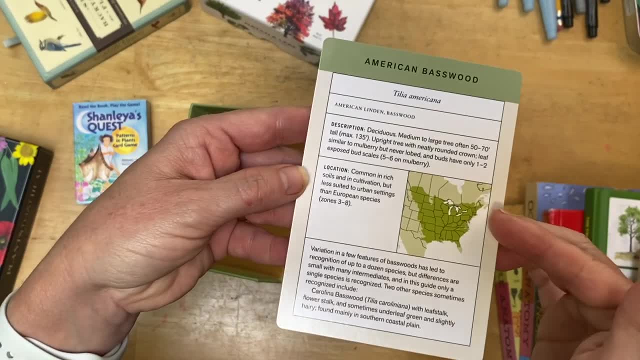 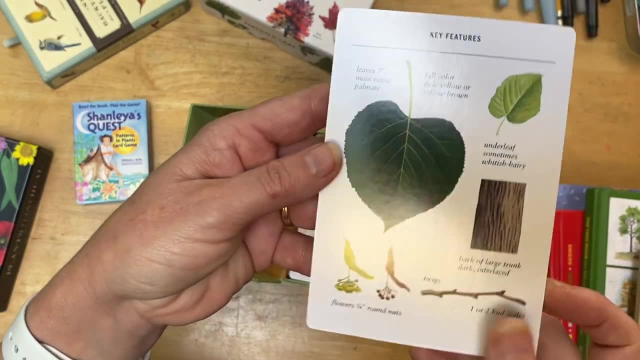 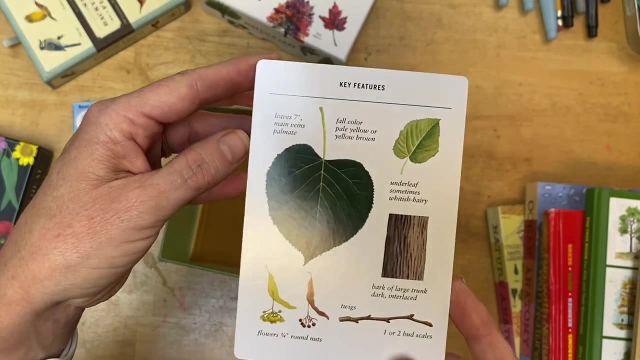 very similar. again. they have this beautiful map that gives the range they have: description, location information and then key features for the tree. i would say the only thing that i would add to this is: it would be really nice to see the tree in its entirety, but you're limited on what. 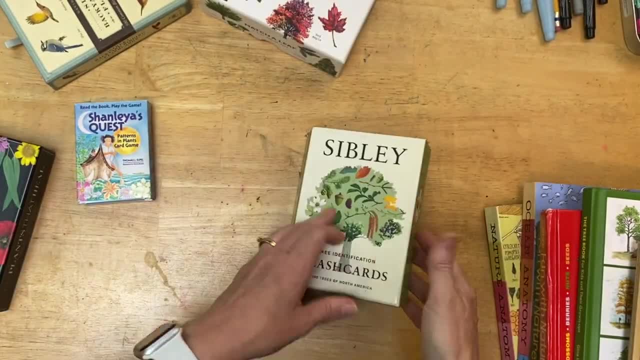 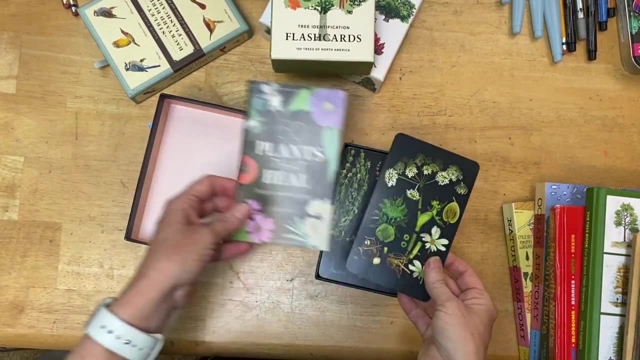 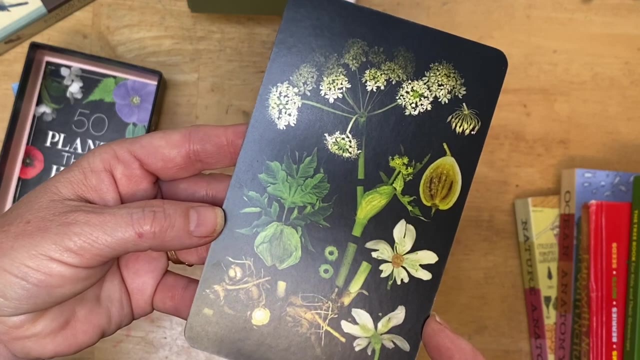 you can do with a card like this. another set of cards that i really like- it's a beautiful set- is 50 plants that heal. these have photographs of the plants on one side and this has been really nice for us in botany and practicing our family skills like knowing the different. 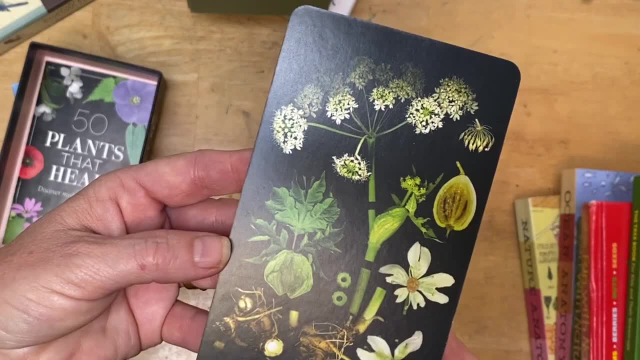 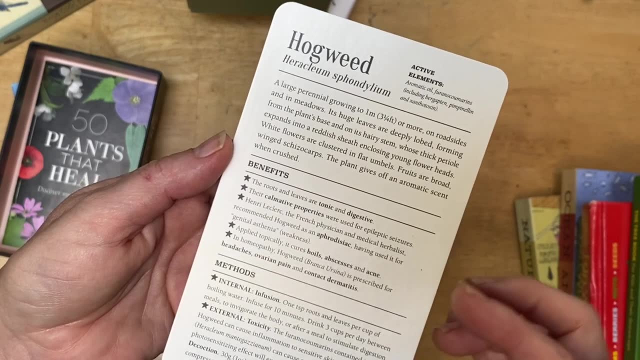 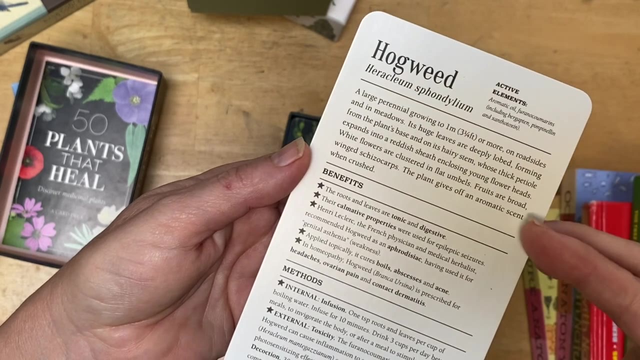 features to look for for those families and finding plants that fit into that family. the other side is we actually have to look it up to see if we have it in the right family, because it does not tell the family name but it does tell the common name and the latin name, as well as the. 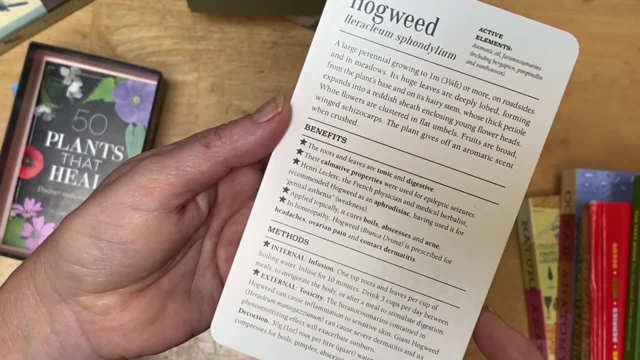 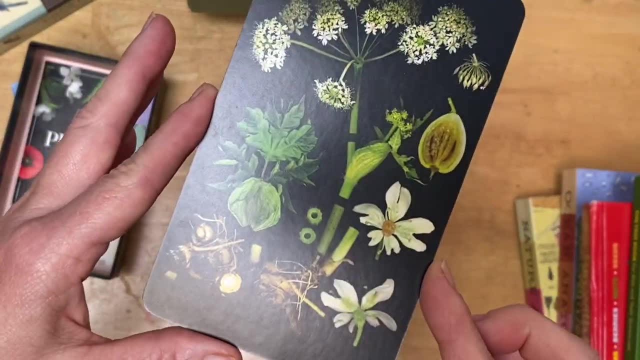 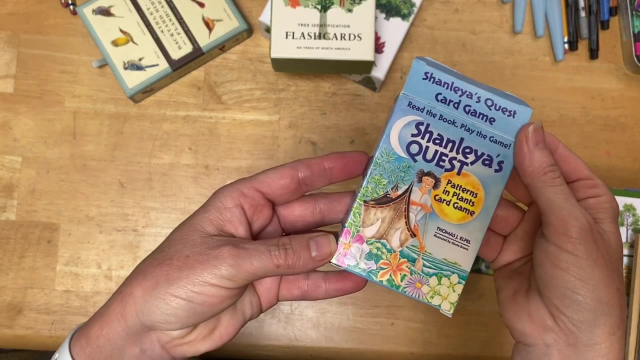 description and then the benefits and the methods used. and the other thing that i think is really nice about all these cards that we're using is it clearly labels when there's toxicity. show you are shanay nela's quest, and these cards are part of the botany in a day which is fabulous. 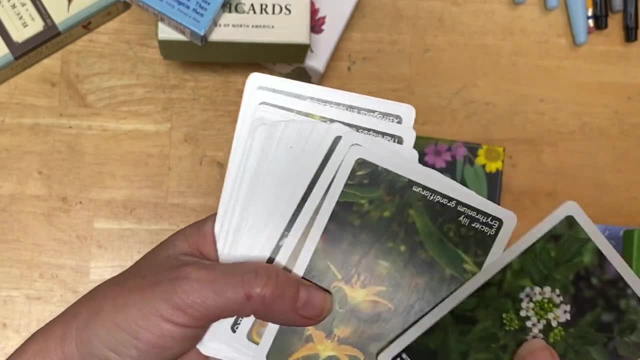 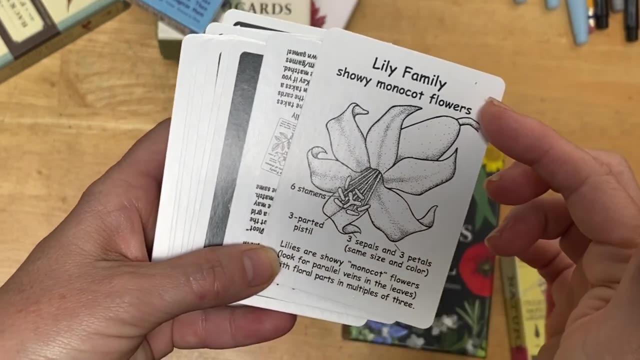 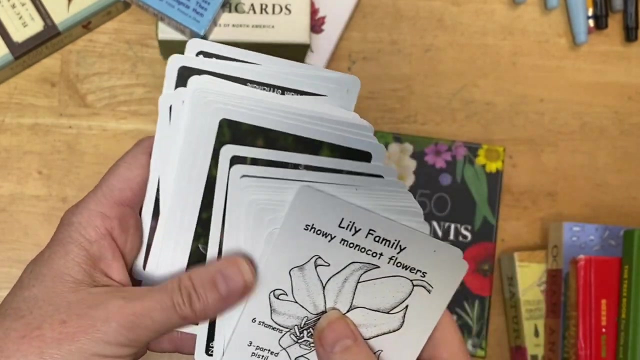 fabulous book. it teaches botany by family groups, which we are doing. it has these cards that give the family name, as well as all the information or key features for the flower when you're looking for that family, and it's a card game, a matching game. so it also has several examples and this is 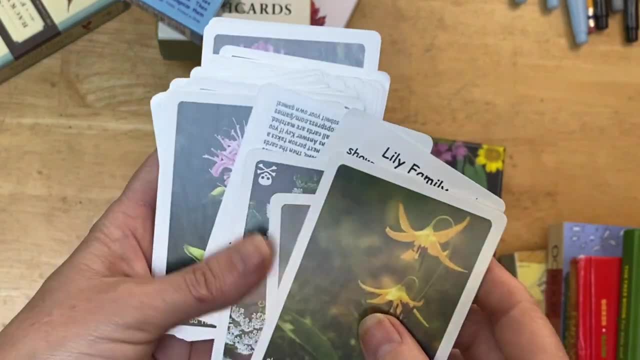 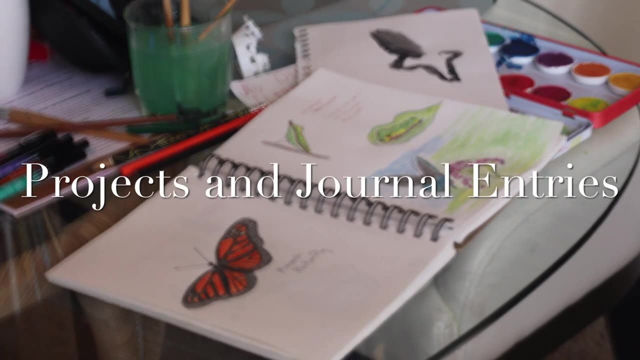 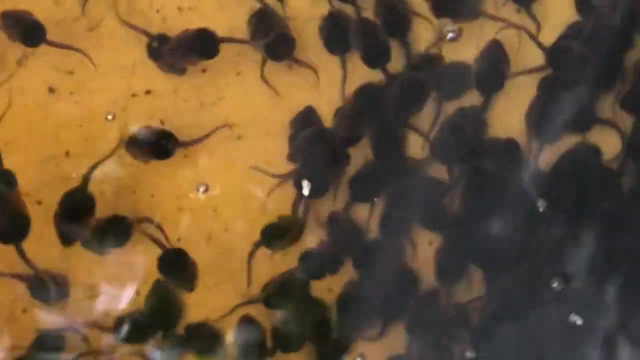 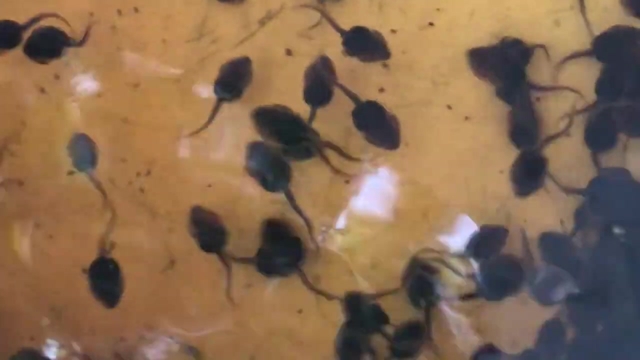 to practice your identification skills in looking for these field marks for the flowers. now let's talk about different projects and entry ideas for nature journaling. so, as i said before, nature journaling doesn't always have to be outside, and I'm going to give you some projects and ideas that don't 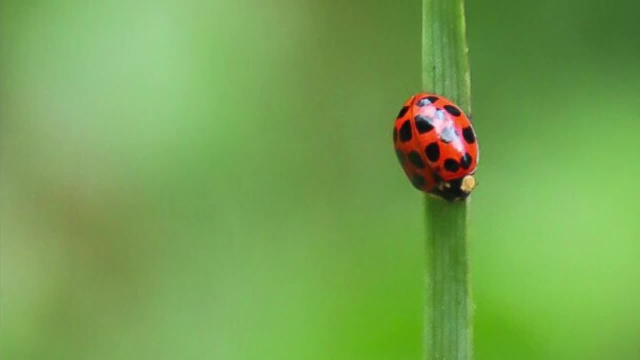 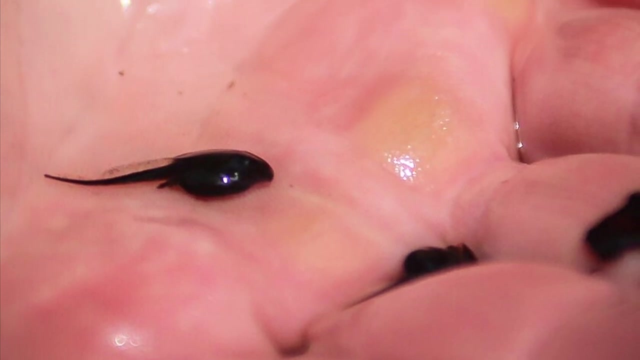 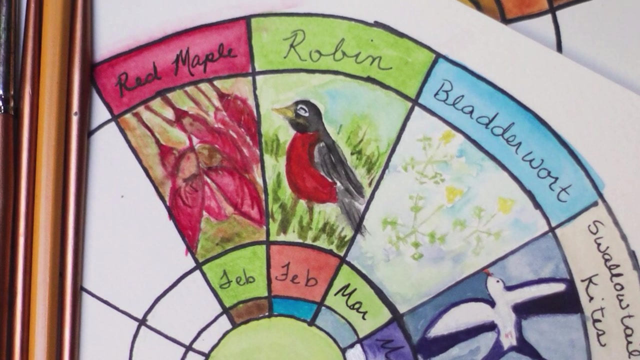 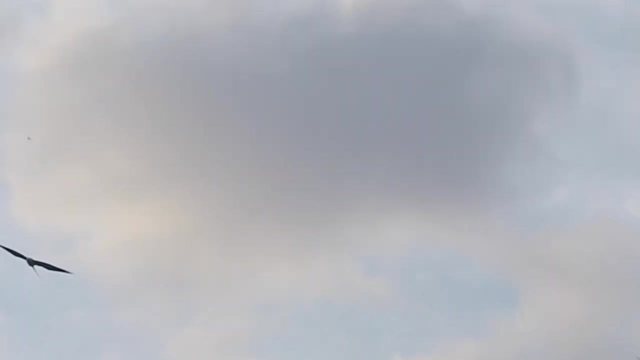 require being outside for that, but some of these will include being outside and are perfect for nature walks and journaling. Here's some ideas for nature journaling. First signs of spring: This is like one of my favorite. We're very much a first sighting kind of family here, so when we see our 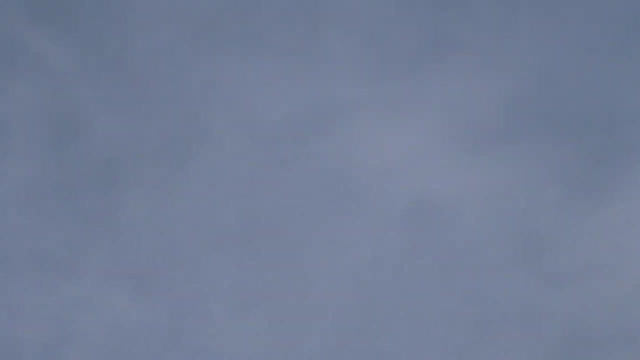 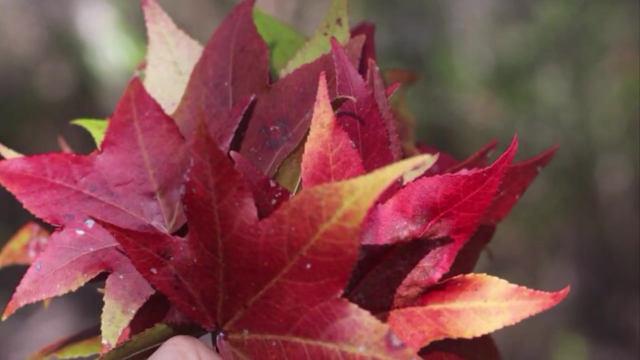 first swallowtail kite, we run in to tell everybody else. My husband will often see the first fireflies because he's out at dusk more than the rest of us and that's a really exciting time. We love fireflies over here Also the first signs of season, or just signs of any other season. 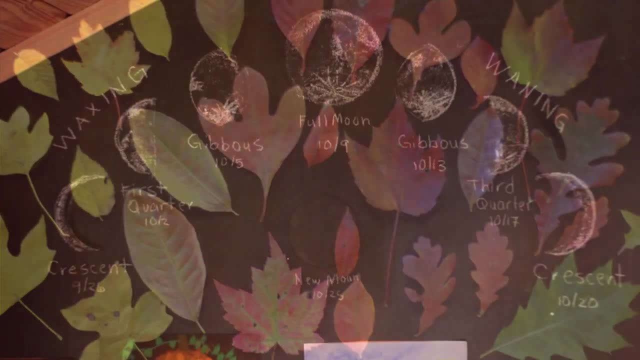 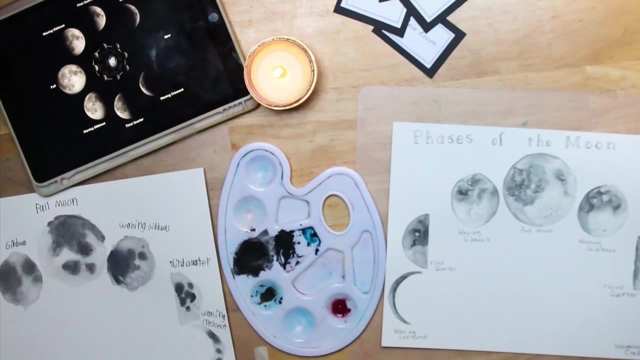 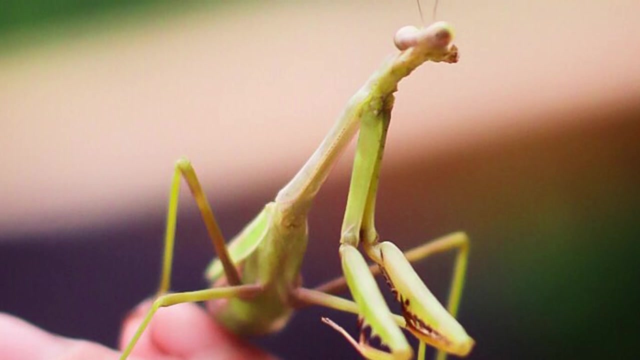 Temperature collection, Moon phases, Paying attention to the moon and drawing where those are, Changes in season, Just something that you notice in nature, which we did a lot of. Just choose one thing and draw it, Often if it's something like an insect or a butterfly that doesn't sit. 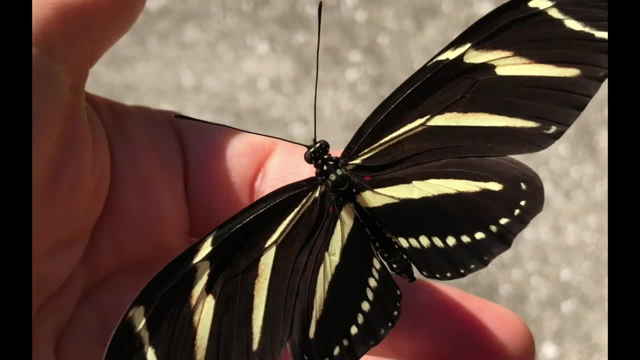 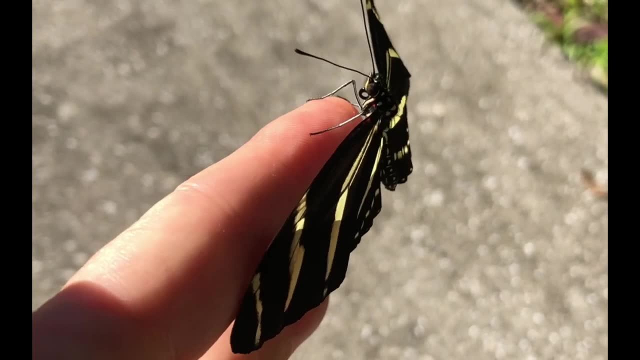 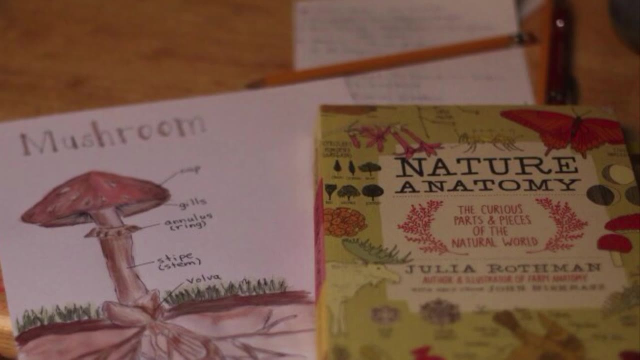 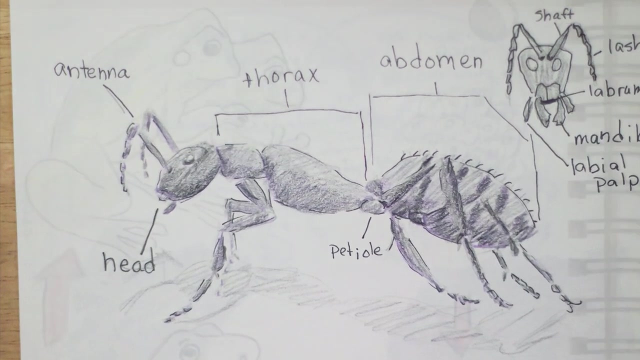 still. you can also look that up on a screen of some sort and use that photograph For drawing or copying, because it's difficult to draw something that won't sit still. Anatomy of a specific thing, item such as mushrooms, if you are working, or trees, If you're working on. 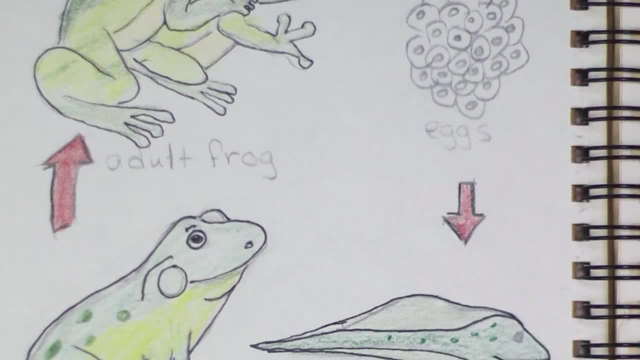 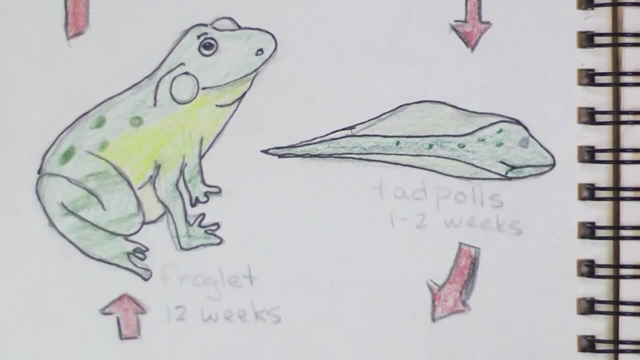 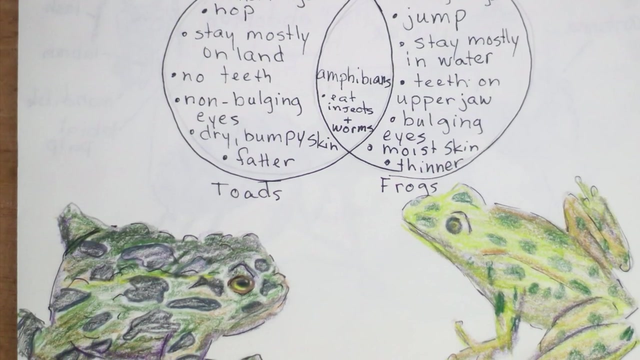 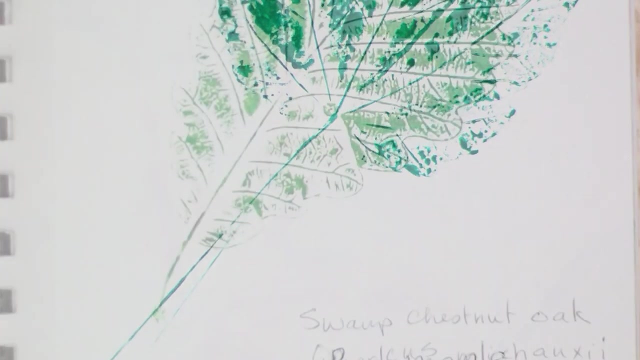 mushroom identification. it's helpful to have the anatomy there. Life cycle diagrams, Comparisons, For instance frogs and toads, would be helpful. How are they similar? how are they different? in a Venn diagram Prints: Prints are really easy and there's a couple different ways you can do prints. You can collect items and bring. 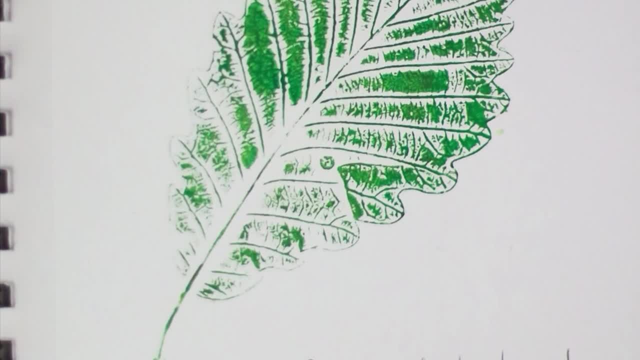 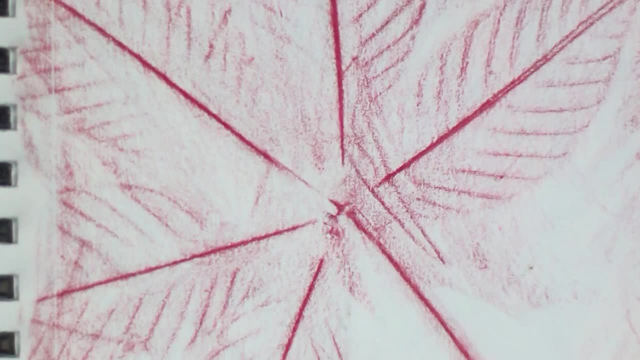 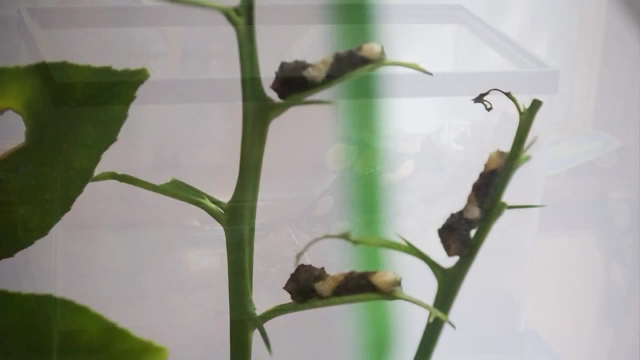 them in and use ink or paint prints, and you can also do rubbings. In addition to that, you can use classroom observations like butterflies or tadpoles and keep those observations in your nature journal. You can collect stats on what you've done in your nature journal. You can also 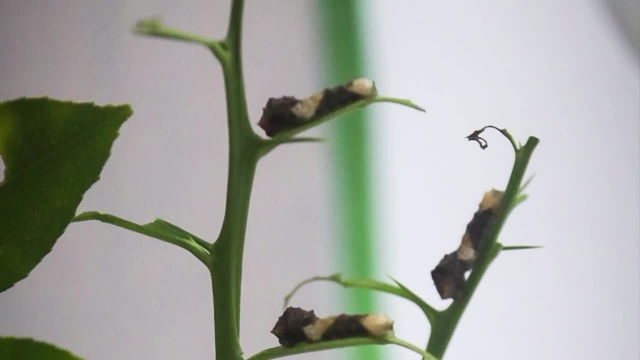 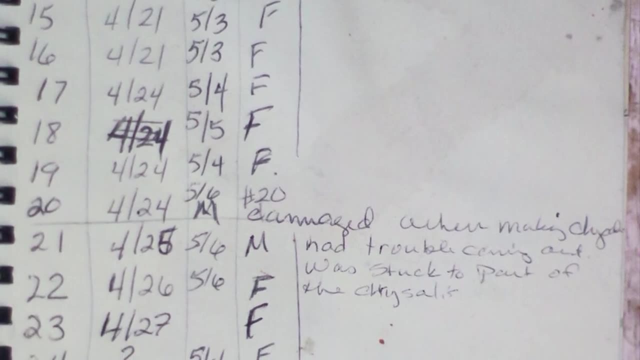 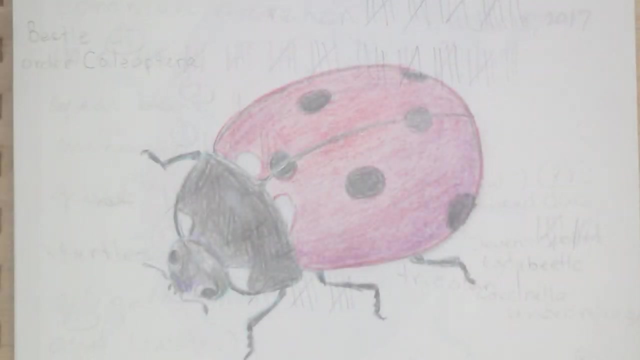 see what you see, The different species that you see for each season of the year. or we have a local state park that gives boat tours. We write down the species and count the number that we see on our boat tours. Drawing practice: You can use nature study for drawing practice, So you can. 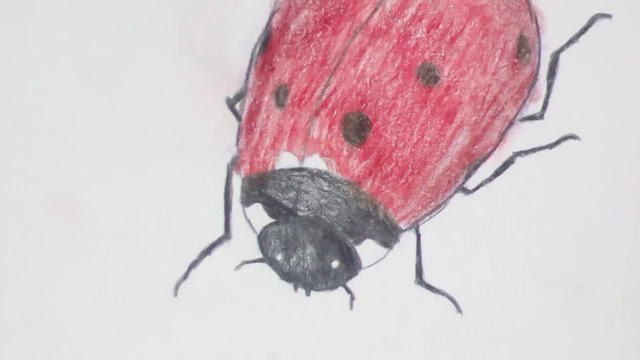 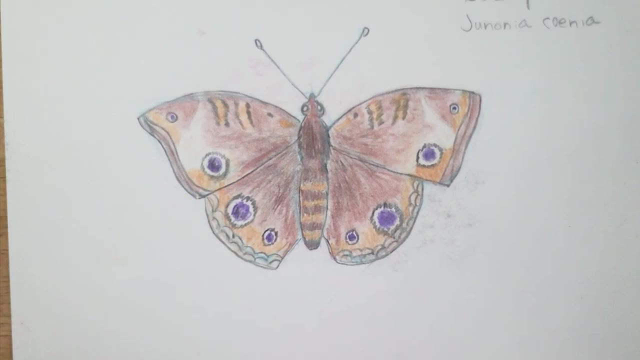 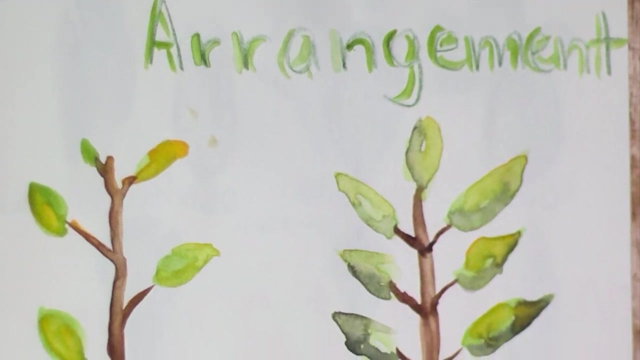 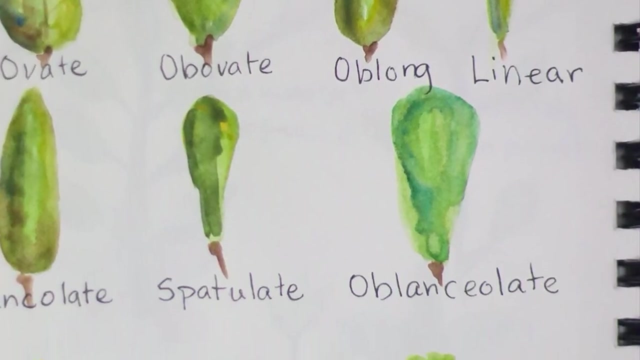 choose something out of John Muir Law's books or some other water coloring or other course and use that to do drawing or painting practice. You can also use the cards to mark and identify key features in identification, For instance for the birds, what you're looking for, or. 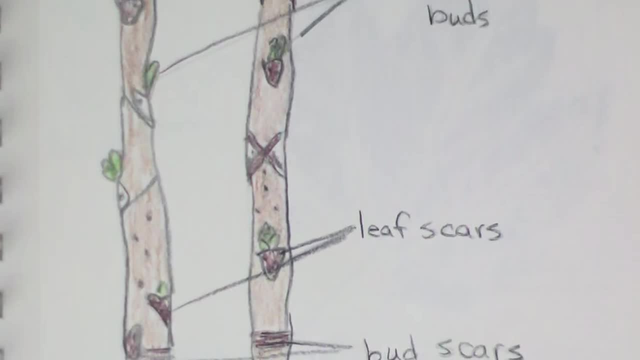 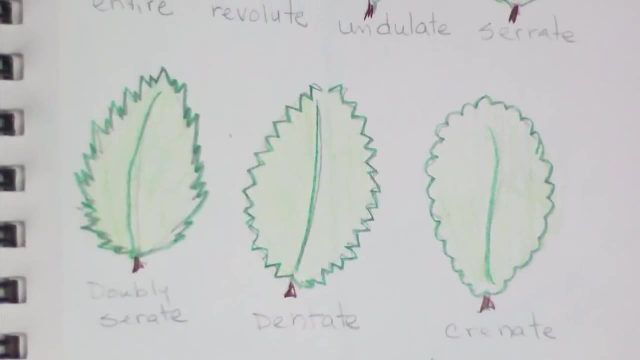 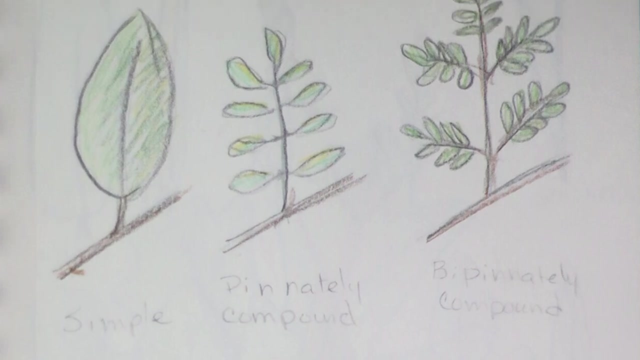 you can do a chart of the different leaped types: margins, venation, etc. If your child is not into drawing or if you just want to keep a simpler thing. there are phenology wheels that are available that make nature journaling really simple and easy, but it will only hold small. 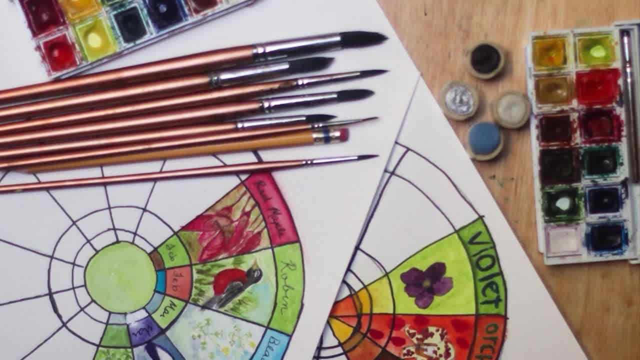 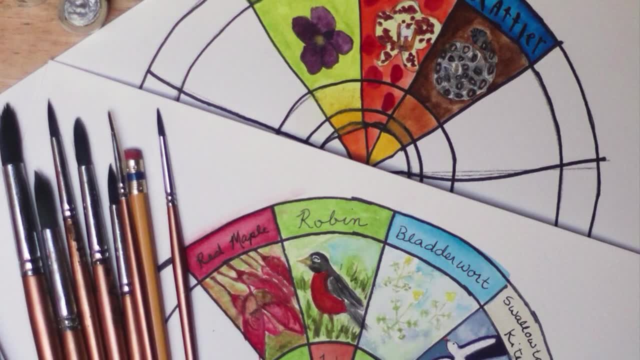 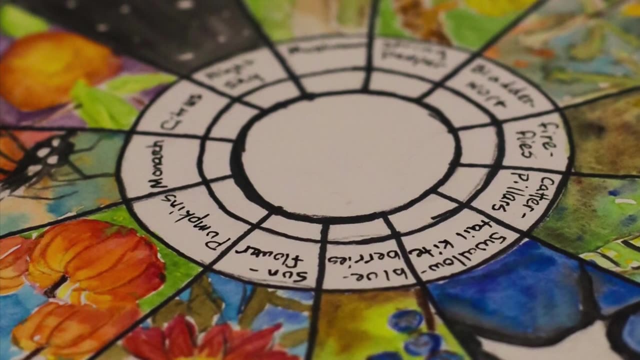 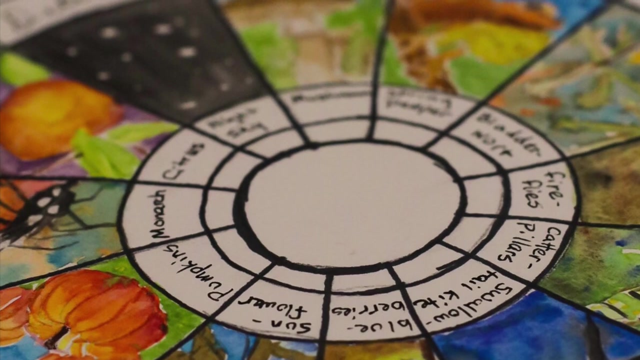 amounts of information. We are currently using a phenology wheel to keep track of our first of spring, which has been really nice, but you can also do one entry a month in a phenology wheel, which is really nice, Or you can easily keep up with temperature by color and moon phase and various other highs. 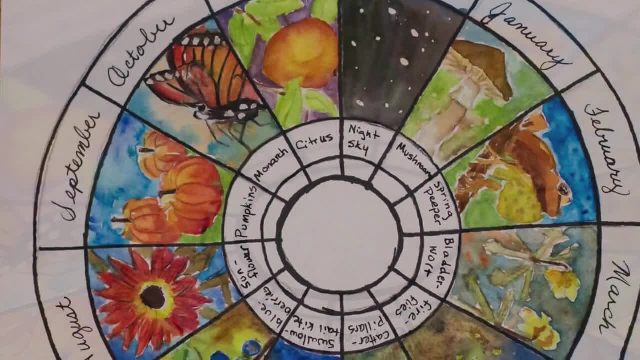 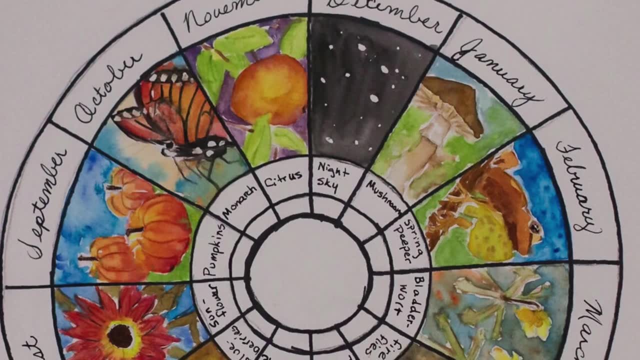 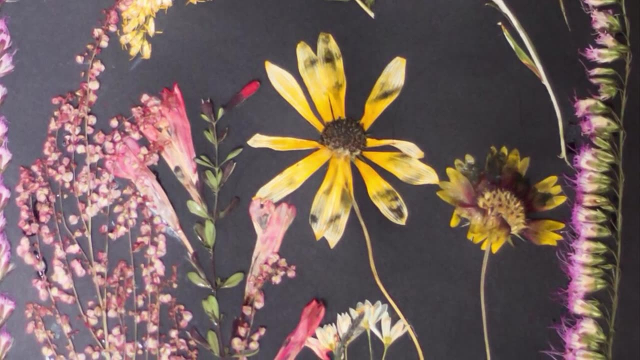 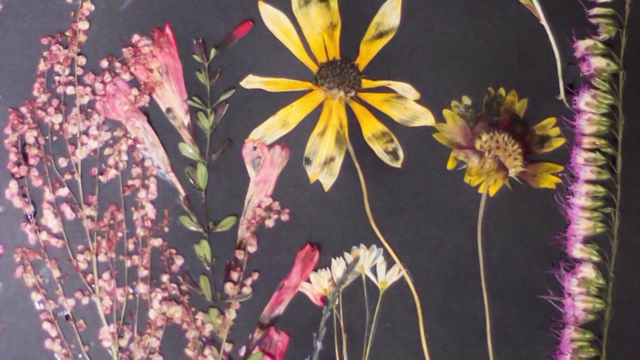 and lows and so forth on a phenology wheel. It's really easy to keep those kind of data points on a phenology wheel. Some projects that you can do for nature study is a leaf and plant prints which I earlier Keeping your own personal herbarium, so in this you would use the flower press and you 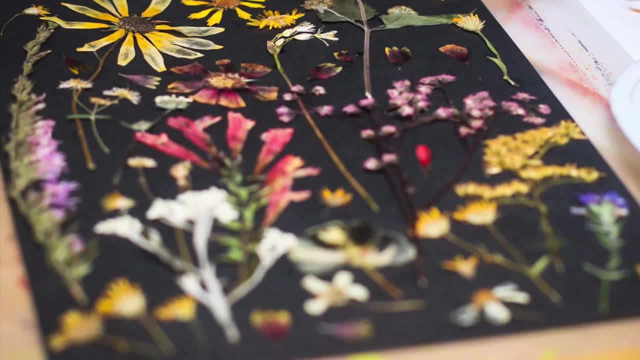 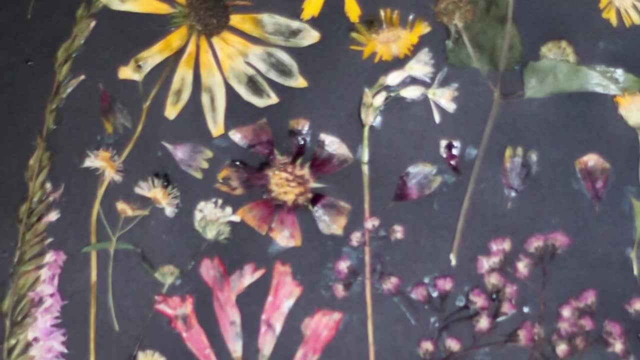 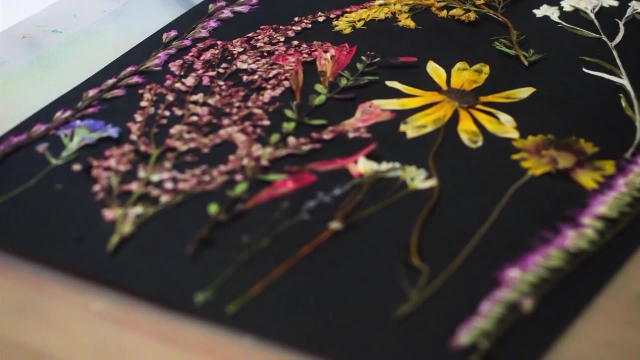 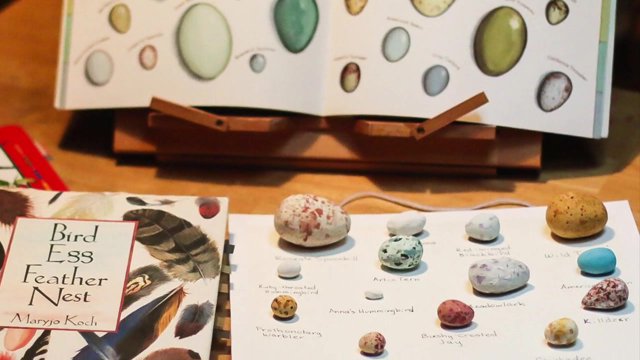 would press the plant and then place that with some information about the plant in your nature journal. You could also do a plant collage with those same dried flowers and plants. We've done egg replicates, so take in either air dry clay or woodpecker. crafts has wooden eggs and you can. 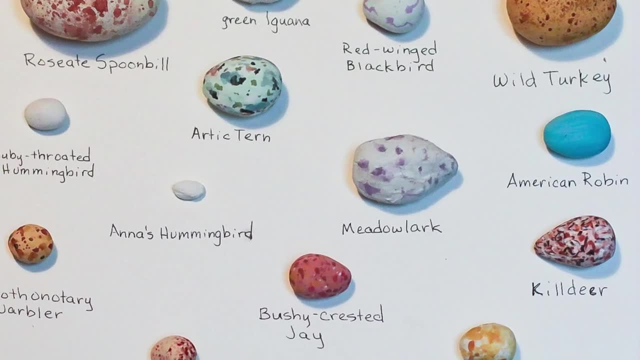 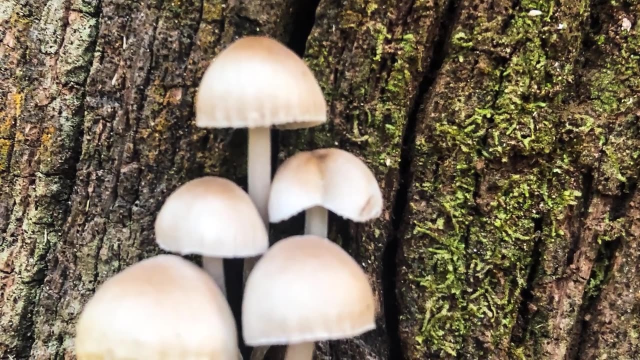 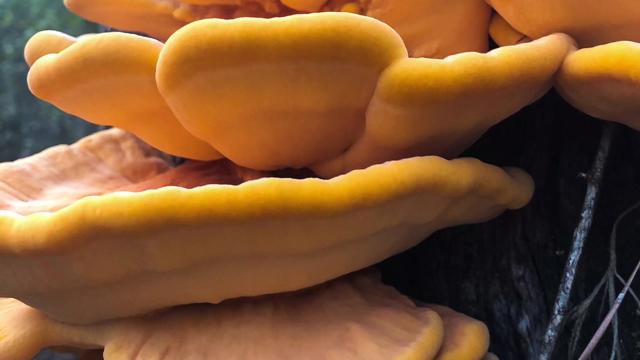 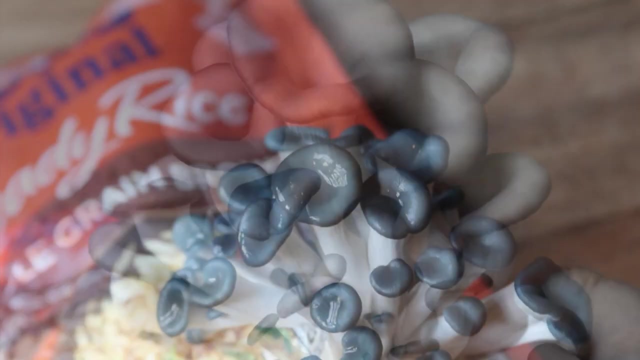 paint those eggs to resemble the eggs of birds that you see in nature. The nature study guides are really good for this. You can also use clay to replicate mushrooms, where you sculpt the mushroom to what you see. You can also grow mushrooms as part of the project and mushroom prints Mushroom. 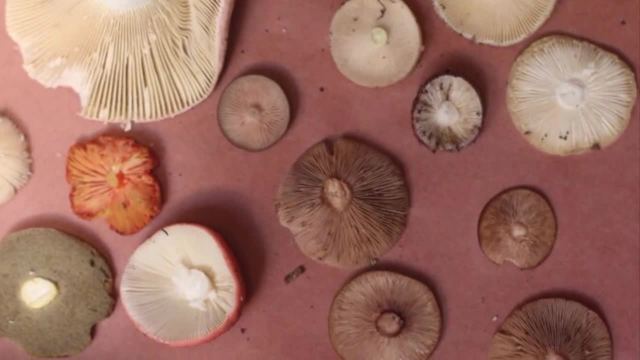 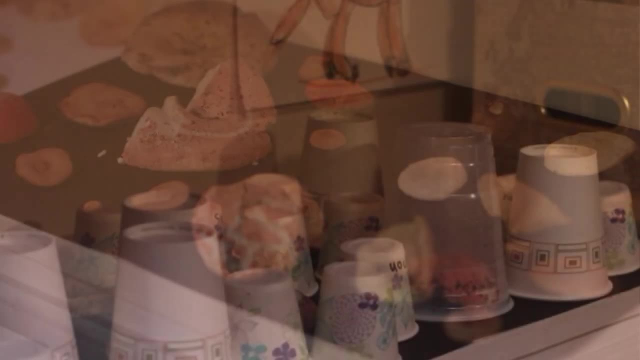 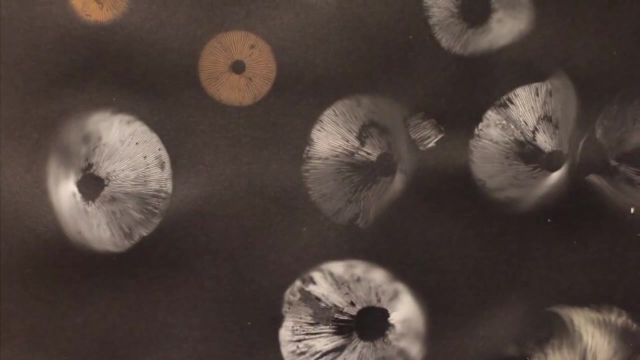 prints are very simple to make. You take a gilt mushroom, cut off the stem, place it down and then cover it with the cup so the air doesn't get to it, and check it within a few hours. Some say to leave it 24 hours. I find that to be slightly too long for a nice, clear print. 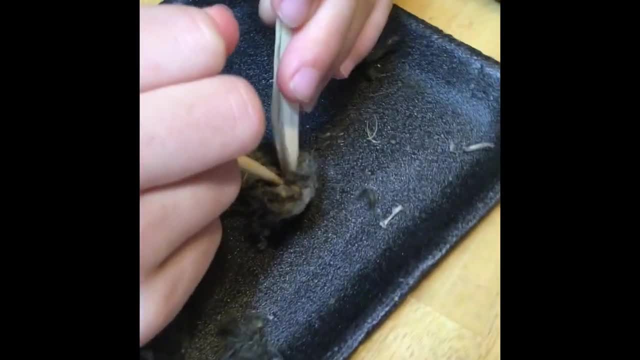 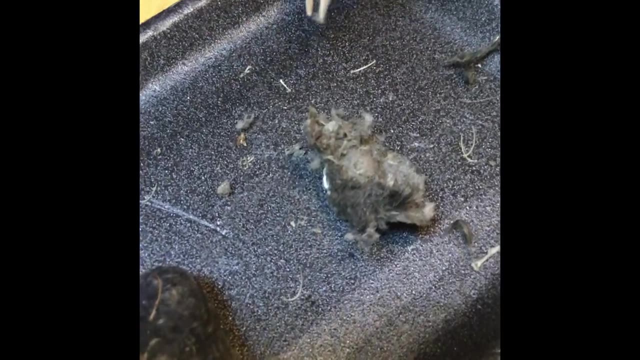 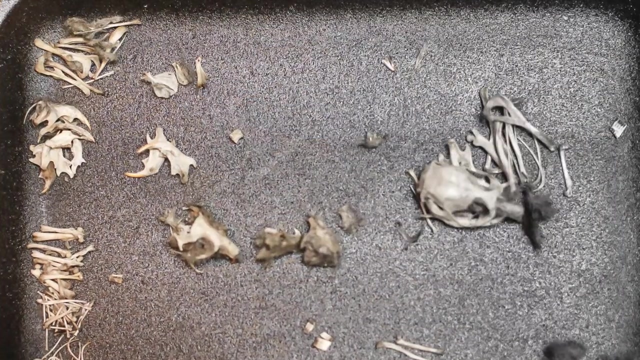 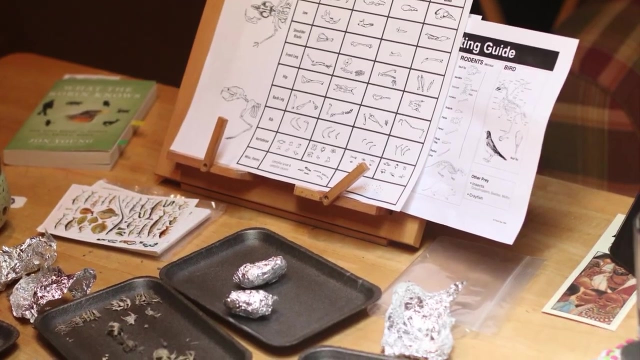 The last project that I'm going to talk about is owl pellets: dissecting owl pellets. This is a really nice project if you're looking at bones or skeletal structures, because you're likely to find a lot of skeletal structures in an owl pellet. That's all for today. I hope you enjoyed the video. I will try to leave as many links and 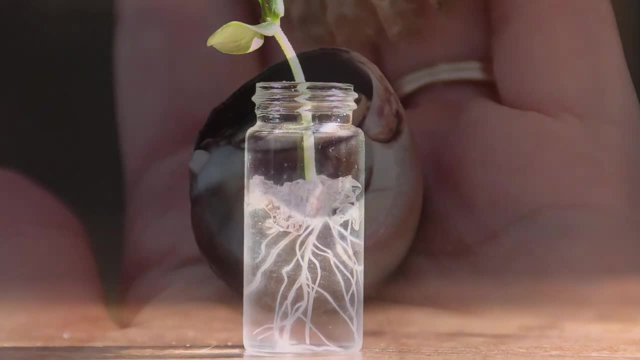 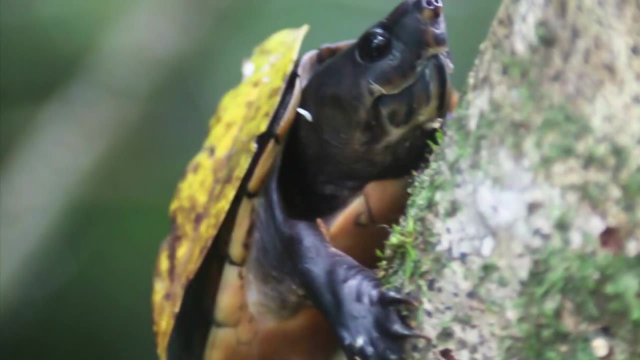 sources, as I can in the description below. If you have any questions, please feel free to ask them in the comments below In the blog post, as well as a gallery of some of our earlier nature journaling pages, so that you can get a view of what they looked like for us. 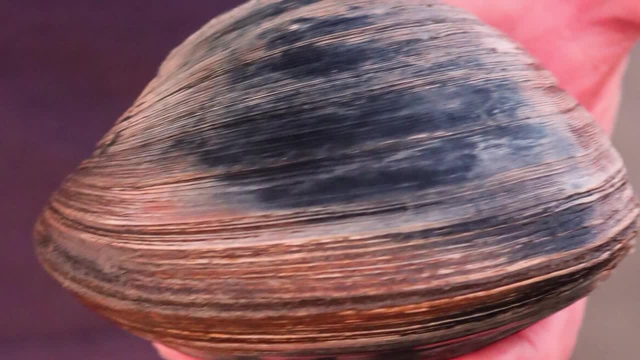 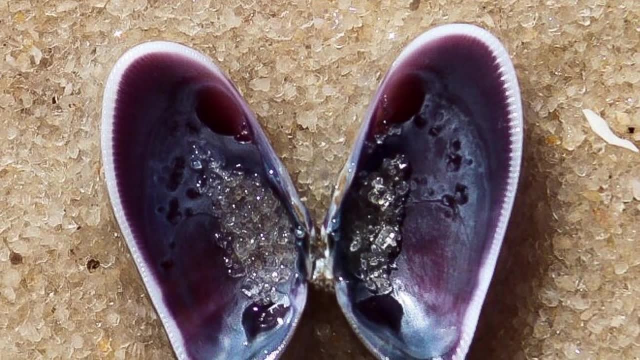 As always, if you have any questions, just leave them below or there's a contact form in your membership area. Until next time, happy homeschooling. Thanks for watching. 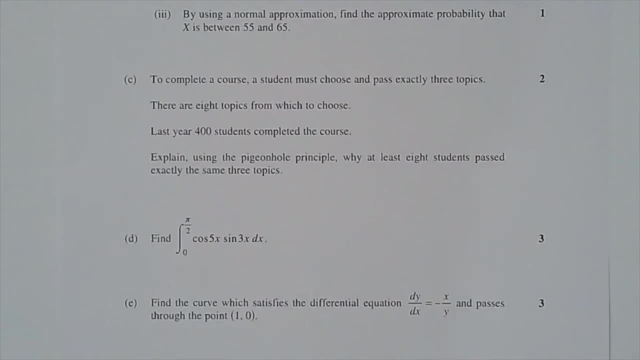 Question 12c: To complete a course, a student must choose and pass exactly 3 topics. There are 8 topics from which to choose. Last year, 400 students completed the course. Explain, using the pigeonhole principle, why at least 8 students passed exactly the same 3 topics. 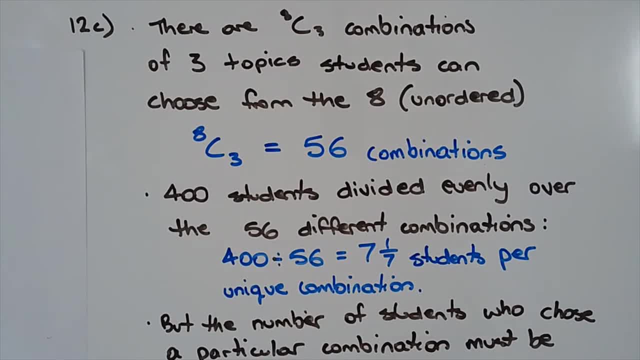 Firstly, we'll consider the number of ways a student can choose 3 topics from the 8.. Now, this is an unordered selection, so we'll use combinations to determine this. 8 choose 3 is equal to 56 combinations, so there are 56 different ways a student can choose 3 topics. 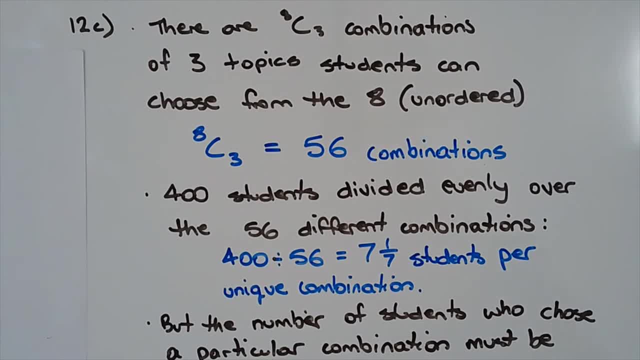 from the 8.. Next, we'll consider the 400 students who passed a course, and a course consists of 3 topics. Now the 400 students divided evenly over the 56 different combinations is equal to 7, and 1 over 7 students per unique combination. 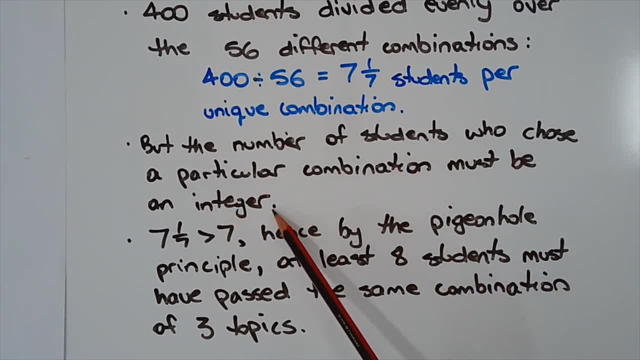 But the number of students who chose a particular combination must be an integer. This failure here doesn't make sense, since we're talking about a whole number of students, Now 7, and 1 over 7 is greater than 7.. Hence, by the pigeonhole principle, at least 8 students.